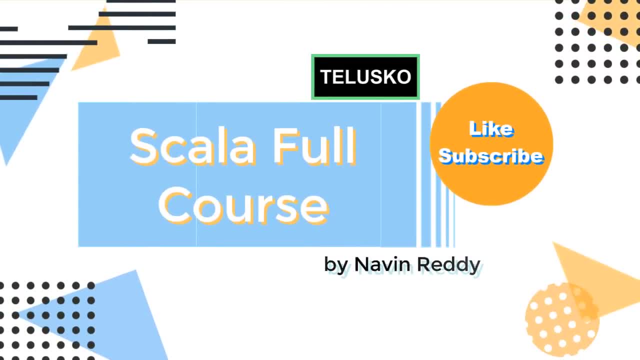 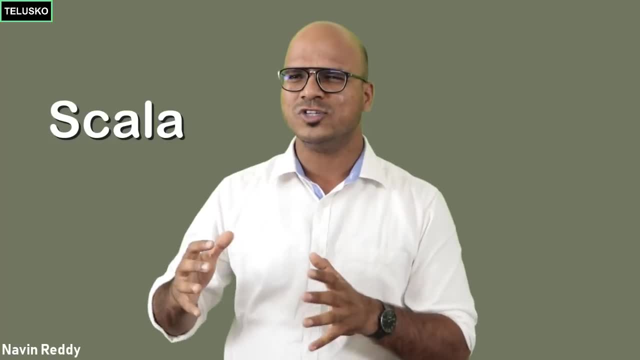 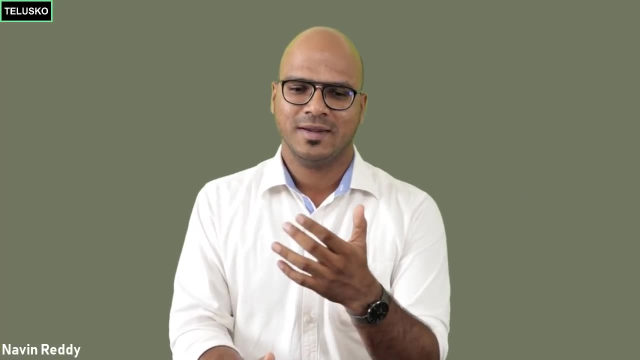 Welcome back everyone. My name is Devin Reddy, and let's learn Scala Now. Scala is one of the most underrated programming language. It's because it's very powerful, but not everyone knows about it Right Now. think about this: We have all these languages right. We have Java, we have Python. 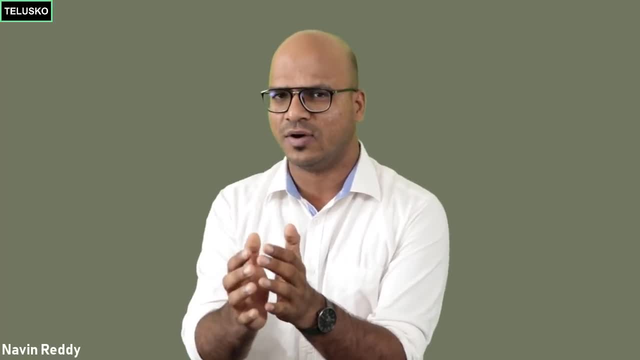 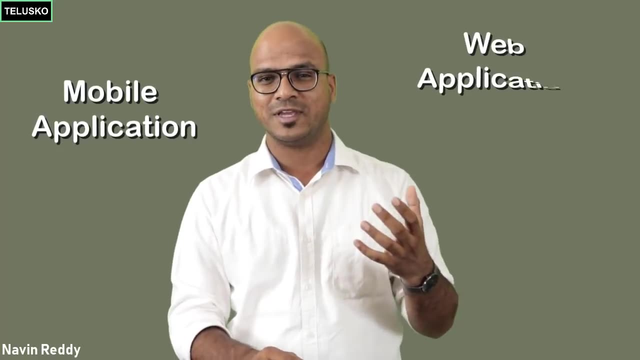 C, Sharp. Now, those languages are powerful. Let's talk about Java here. Java is powerful. It's an awesome language. You can build amazing applications there, starting from mobile application to web application. We can also build enterprise application. but still, we have one issue with Java. 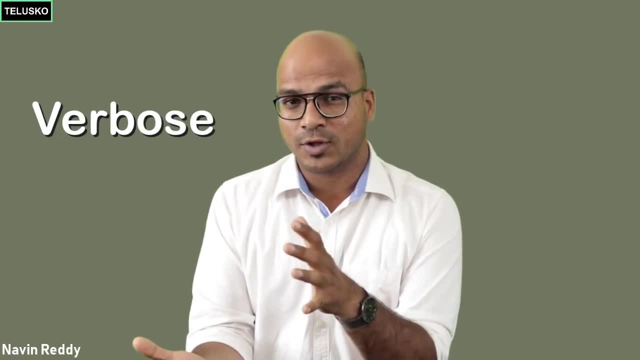 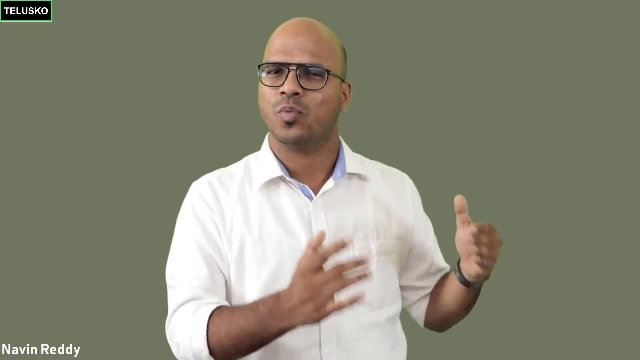 which is it's very verbose. It means you have to write a lot of boilerplate code. On the other hand, in Scala we write less code. We don't write boilerplate codes there. So if you want to achieve a task, just code what you need. That's not the case with Java, right, But you might be thinking. 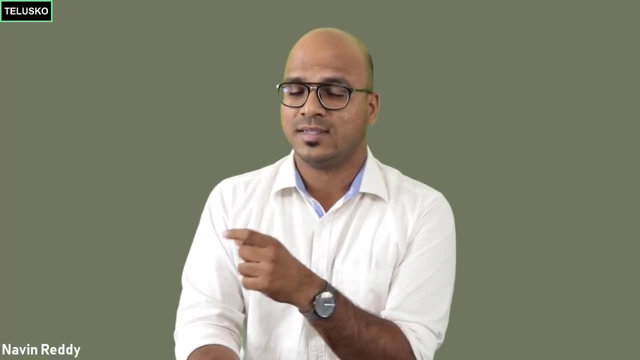 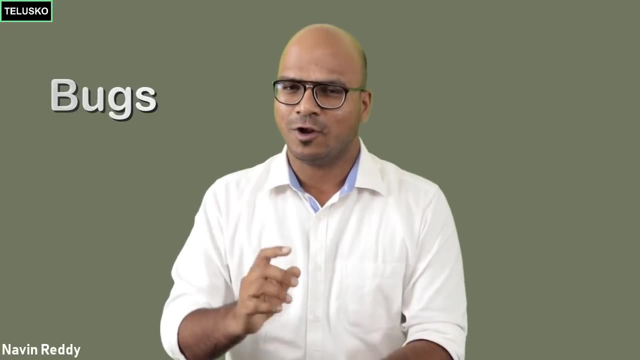 that's fine. You know, we are happy with Java. It's okay to write some extra lines. That's where the problem starts. The more lines you write, it increases the possibility of having more bugs. right. It also means the bugs are directly proportional to number of lines. So if you write less lines, you will have less. 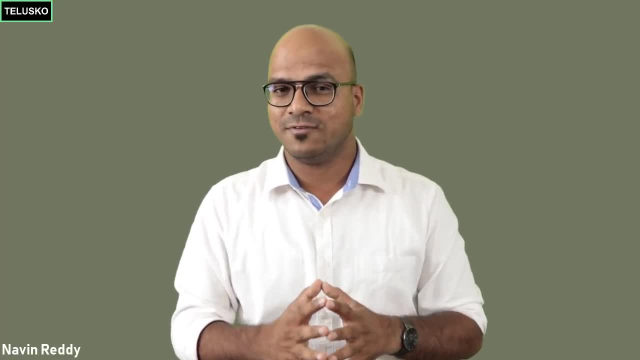 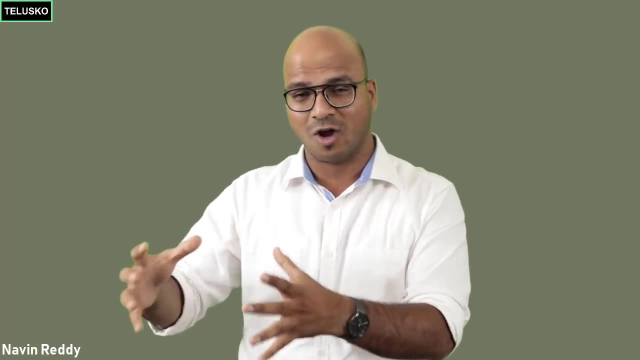 bugs. That's one thing you will get with Scala. Now, one of the amazing features of Scala, which I like, is it's a JVM language, which means it uses the same concept with Java users. We have JVM there. All the internal working is same, The language changes. Plus, it gives you a functional styling. 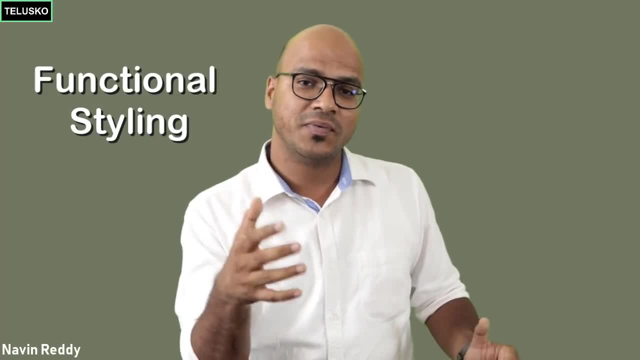 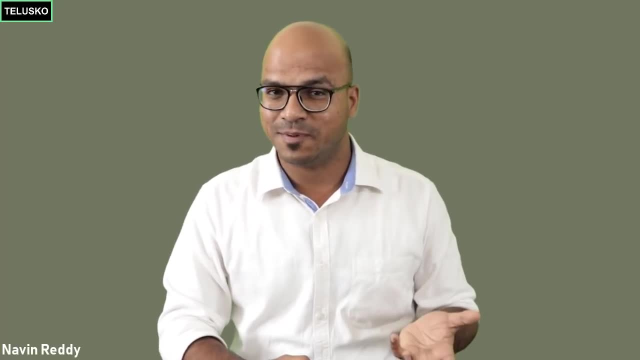 as well, which means not just object-oriented, but it gives you a functional styling as well. So it's a combination of both, and that's what makes your programming experience better. So, while learning Scala, it will change the way you think about programming, about the task right. 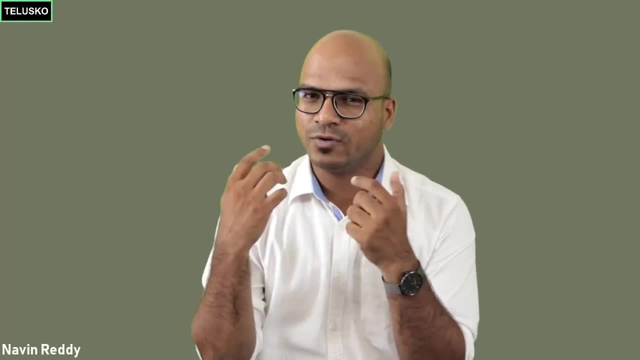 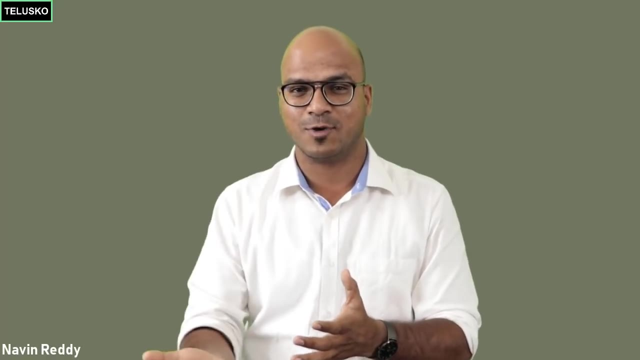 In fact, I have seen this. as we learn new languages, it will change the way you think about language and then the way you implement them. So when I work on Java, I have a different mindset. Same goes for Python: We have a different mindset, and Scala will give you a very different experience. So I hope you. 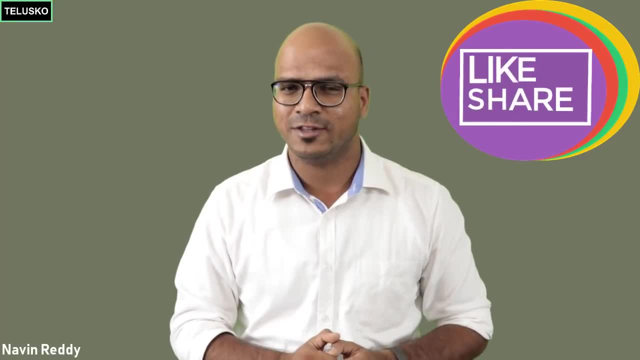 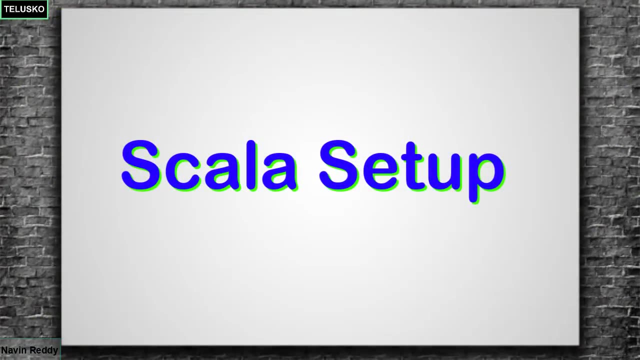 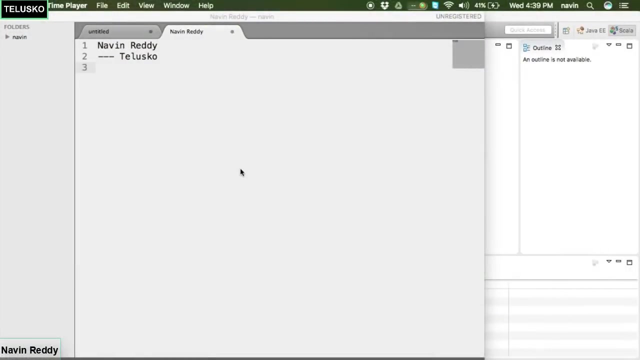 will enjoy the entire course. If you are excited, hit that like button and do subscribe, because on this channel we post lot of programming videos. In this video, we will see how to set up Scala Now, once we know what is Scala, once we know 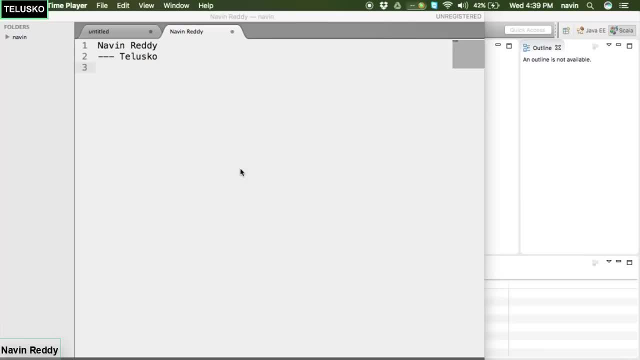 why we need to learn it, and the prerequisite to learn Scala is Java, of course. So you should know the basics of Java and you are good to go. So let's. in this video, we will see how to set up Scala so that we can work on it. 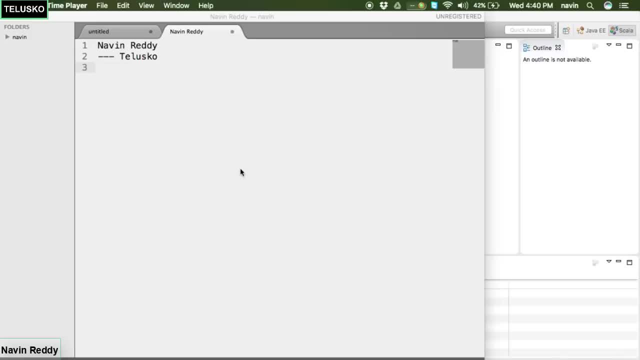 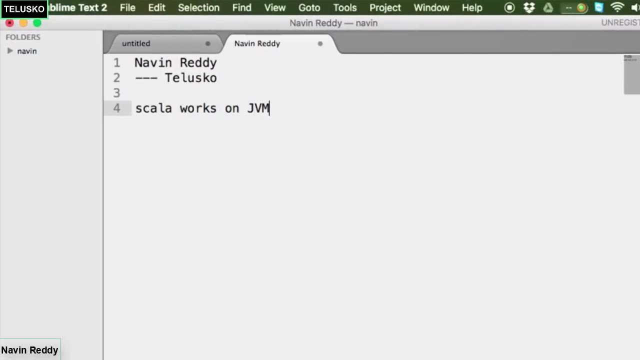 So, when you work with any programming language, let's say C, C++, Java, the first step you have to do is you have to download some software so that we can work on it. So, for Scala, what we need now? Scala, since, as we know, that Scala works on JVM. so that means, since Scala works, 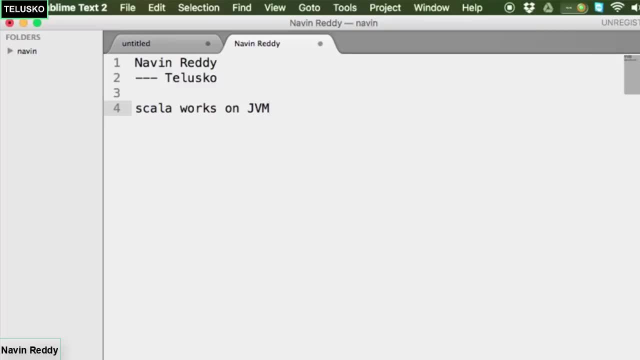 on JVM. Eclipse supports the languages which works on JVM, so we can run Scala on Eclipse, right, And that's one of the amazing thing about Scala- And you don't have to learn a different IDE for that. you can simply use Eclipse, which. 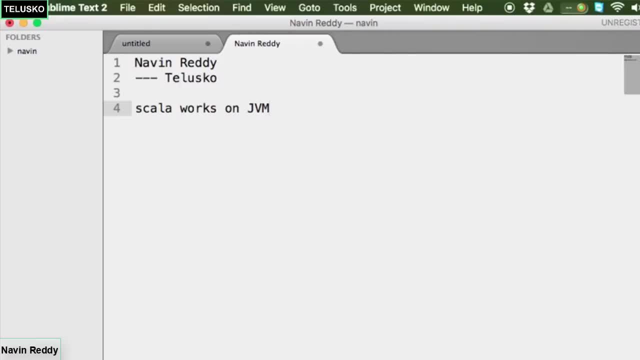 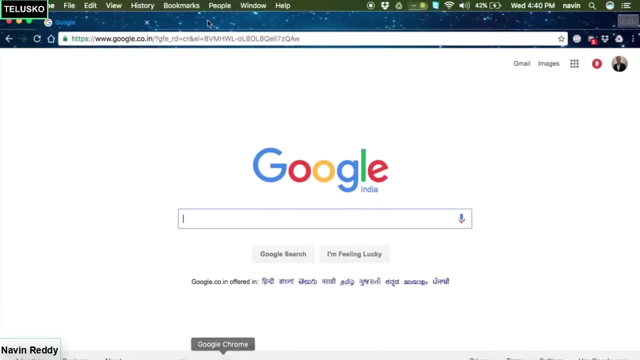 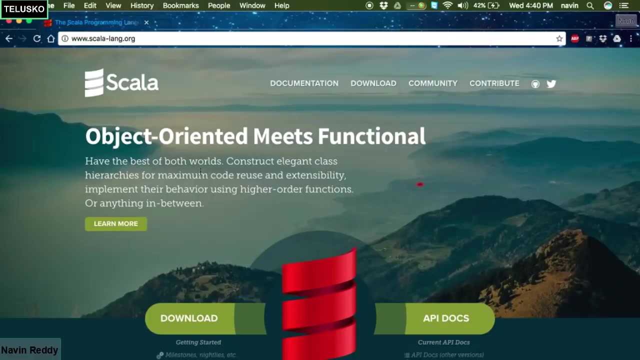 is our old golden Eclipse, which we work with Java. right, So we can do. we can work with Scala on Eclipse also. But if you go to the official website of Scala, so you just have to search for Scala and it will take you to the official website, which is Scala lang org. right, And if you go here, 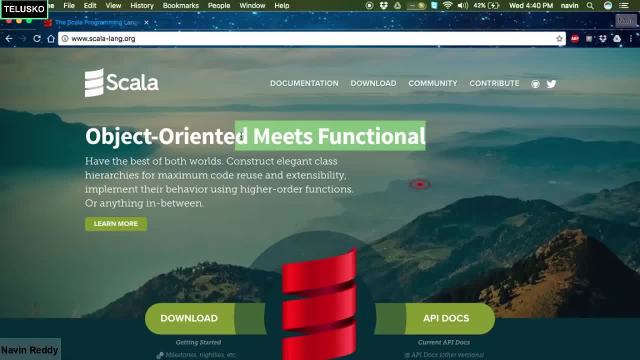 so see the heading. it is object oriented meets functional, and that is awesomeness. you know, Scala is both object oriented and functional, so it has lots of power in it. So if you want to be a powerful programmer, Scala is the way. 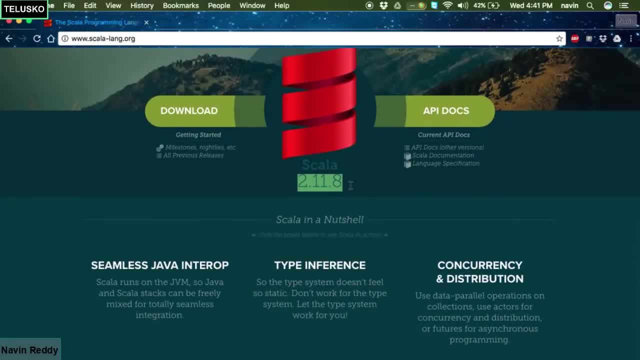 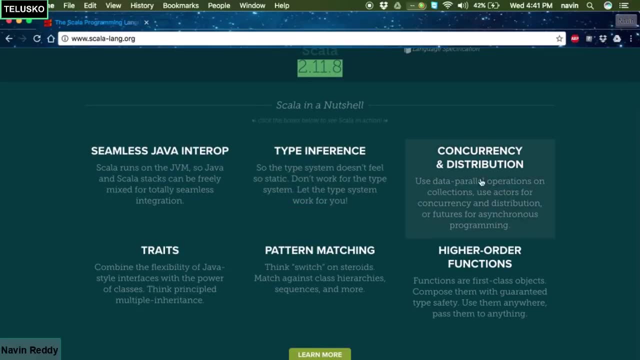 And the latest version of Scala is 2.11.8. and these are the features of Scala: it is Java interoperable, then type inference, then it provides concurrency and distribution. It supports high add-on function- we are very excited for this part- Then it has pattern. 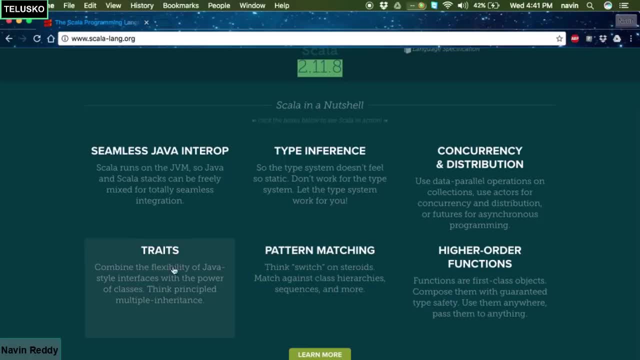 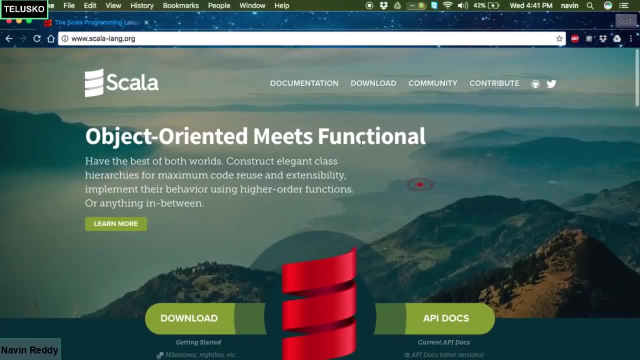 matching. It has threads. If you know interfaces in Java, that is threads in Scala, I have to learn the pronunciation of it first. Okay, so we can go through this download tab here and if you click on this download you can see you got three options. 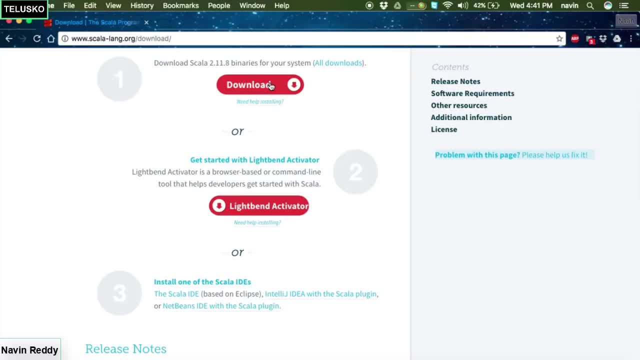 So you got this option, which is the download, the binary version of it, so that you can, if you want to work on terminal or if you want to work on CMD, this is the best way. You can also use the light bend activator. 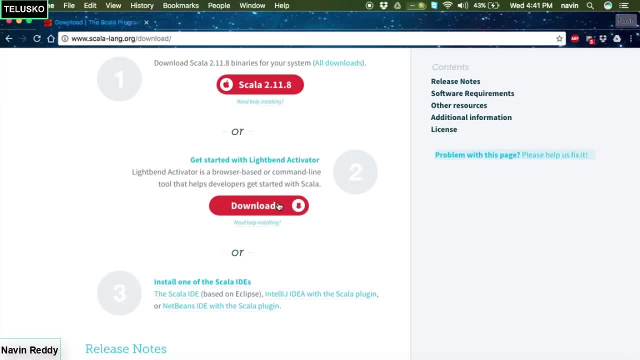 This is another tool which we can use. Now, if you use this tool, it is a web-based tool, So that means the software will be installed on your machine, but to access that we have to use web browser. So if you will be typing your code on web browser, you will be running it in your web. 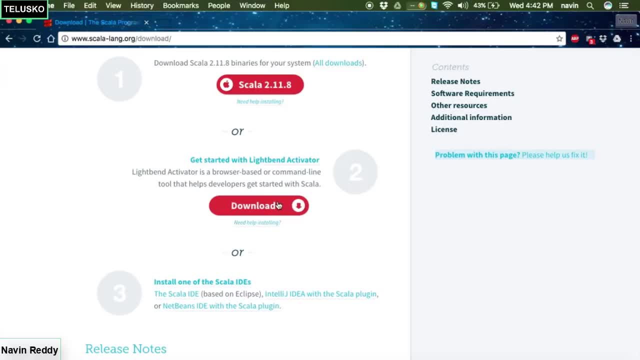 browser. Okay, this is an amazing tool. In fact, if you download this, it is very heavy file- around 700 MB if I'm not wrong- And we can also use the Scala on IDE, So you can run Scala on Eclipse, you can run Scala on IntelliJ or you can run Scala on 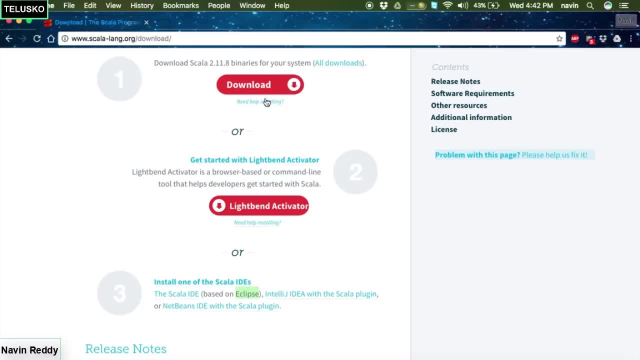 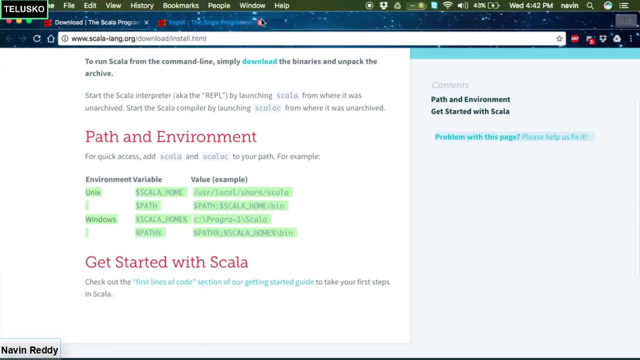 NetBeans, And this is a great tool, I mean. so if you work with this, you have to do this step. So if you click on this, need help in installation, you have to set all these parts. That's one way. 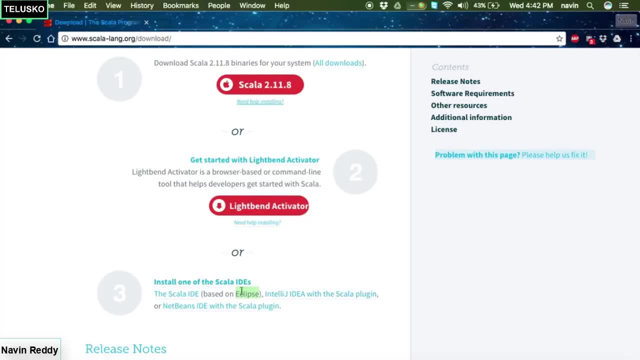 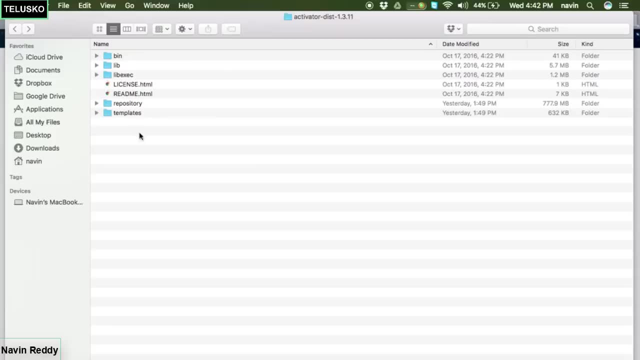 A second way. if you download this one again, we'll be using Scala IDE Eclipse for our tutorials, But let me show you how this works. So if you download this part and if you unzip it, this is how it looks. 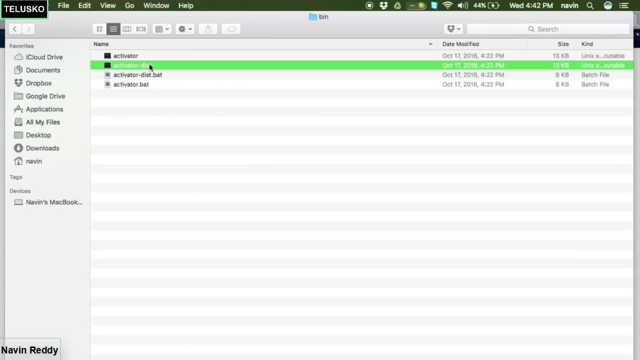 So this is how it will look like: Go to bin and there's an option of activator disk. Again, you don't have to do this, It is just for if you are curious about it, Then you can do the experiment. Otherwise, leave this. 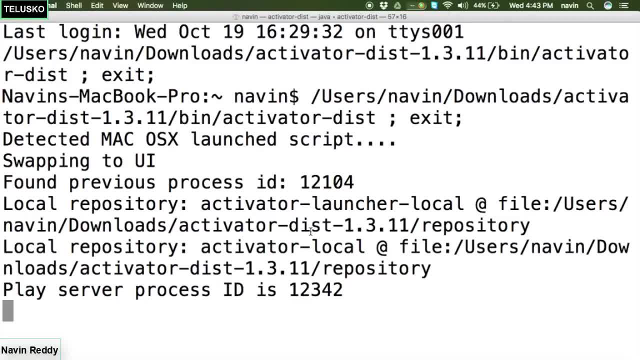 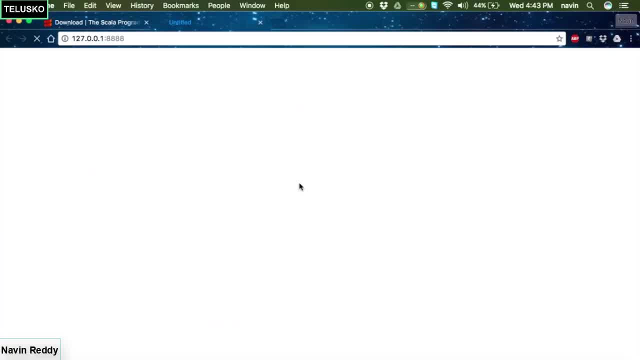 We'll save this once we got some experience on Scala, So it will take some time to open. Don't worry, I've just changed the font of my terminal. That's why I'm just showing you so much big text there, So it will open in this way. 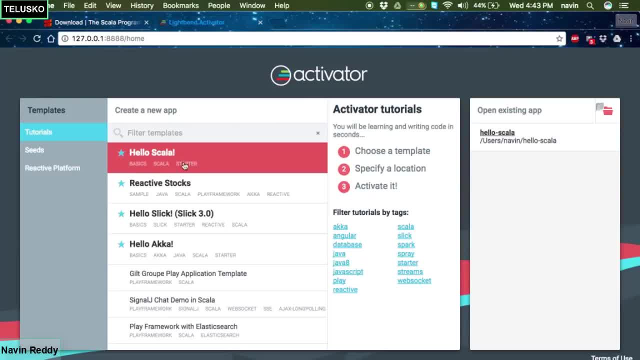 You can create a new project. So you can click on Scala here. So this is Scala, This is slick. Slick is for database. I mean, if you want to work with some database framework, with Scala, you can click on this. 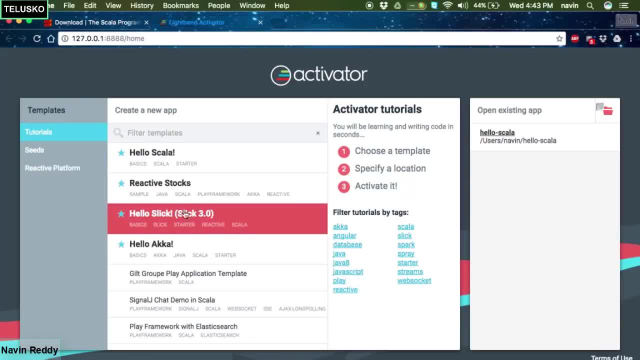 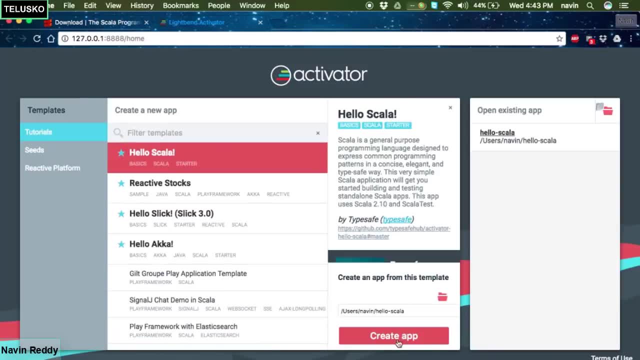 So this is Scala. This is slick. Slick is for database. This is Scala. We can use slick. We can also use play framework here. Play is an amazing framework to work with. So if you click on Scala, it will ask you to create an application. 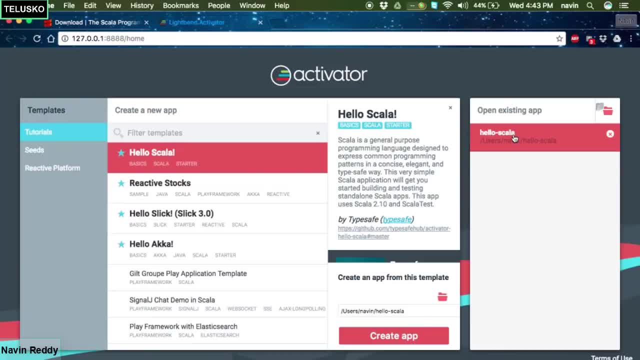 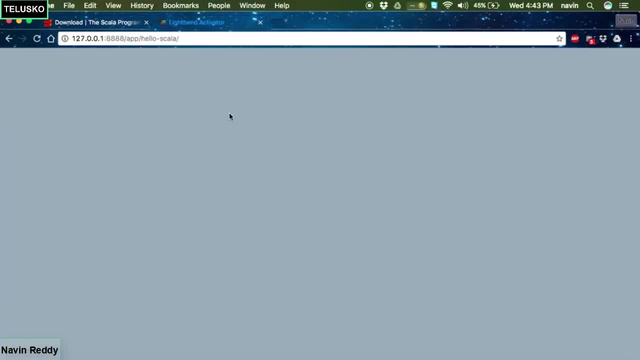 So I have done some experiments, So I already have an application here. The point to remember is this: Scala, I mean this Scala is supported by type safe company And if you click on this project, I mean if you click on the existing app which I 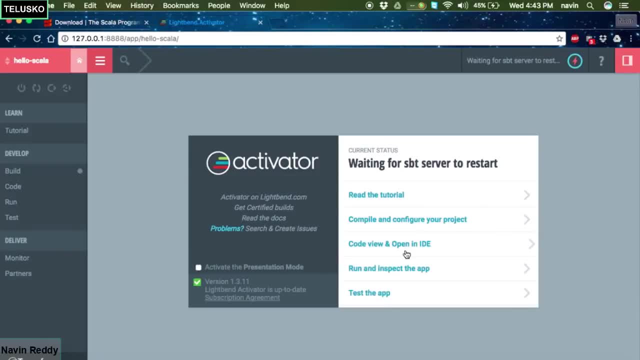 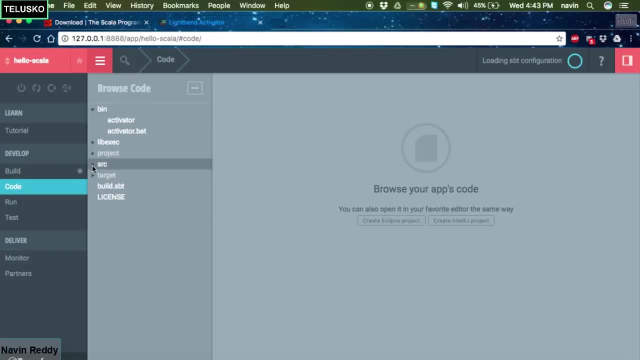 have created. So this is how it looks like. I will run an inspector object. So that's good. Where is my code? So this is what I was doing on that day: I was doing some experiment, I was printing all those stuff. 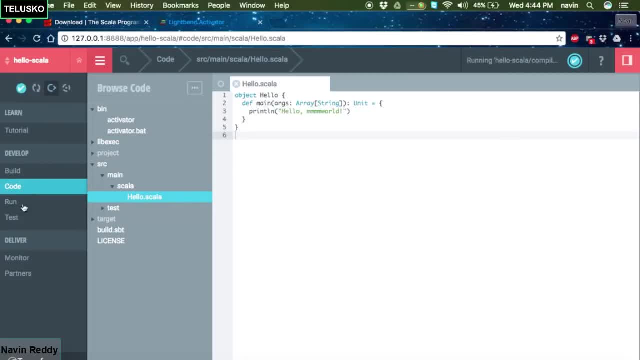 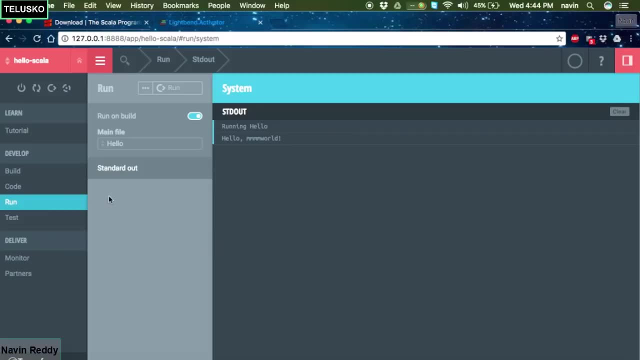 You can just simply run this code by clicking here and you can see the output in the run tab and you can see we got the output. Okay, so we can use this window, But I'm not a big fan of this window. I don't like web console based things. 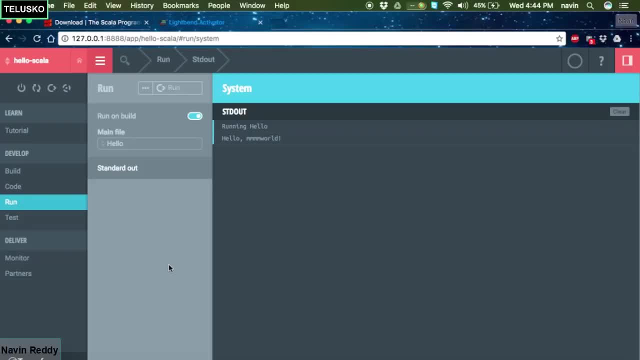 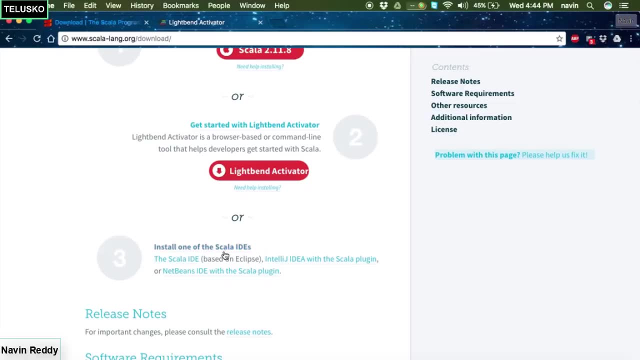 But if you like it, you can explore this thing. There's no harm in that. But my interest is more on the Scala, on Eclipse. Okay, Now, how to do that. So there are two ways. One, you can download the Scala IDE itself, which will be around 200 to 300 MB. 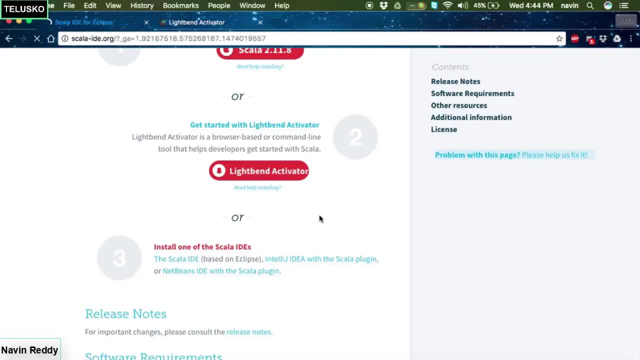 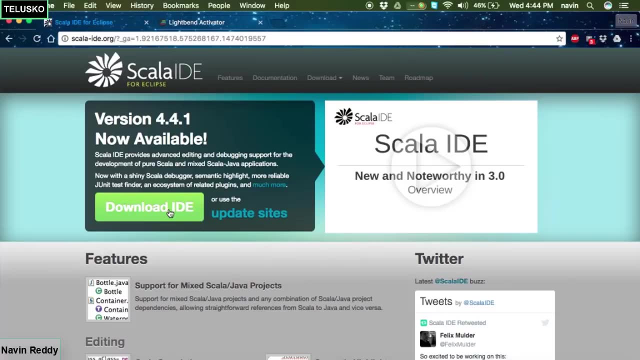 I'm not sure about the size. The another way is, if you already have Eclipse in your machine, see if you can. if you can, click on this, it will download the whole Eclipse for you, where you'll be having Scala in build. But if you already have Eclipse in your machine, 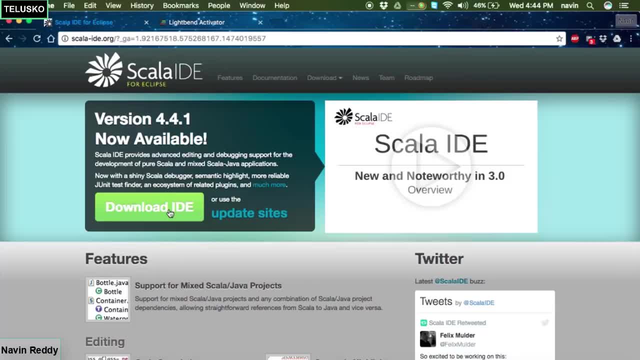 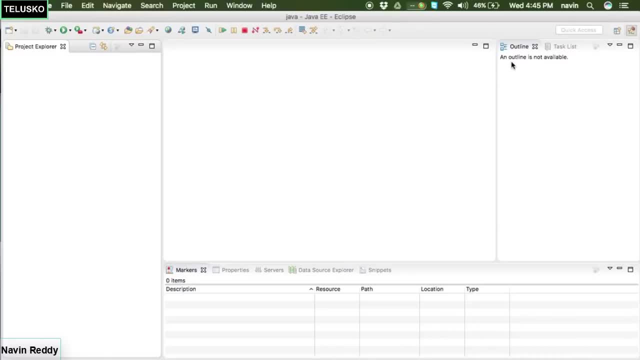 Where do you have Eclipse? Where you used to work with Java? What you can do is: example: I have my Eclipse here, So you can see I have Eclipse here, But in this Eclipse I don't have Scala. You can see if I click on new. there's no Scala project option here. 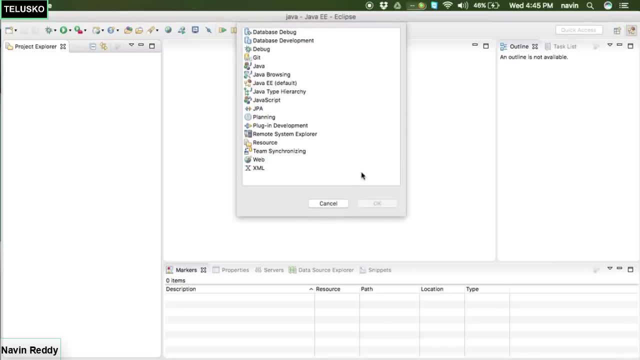 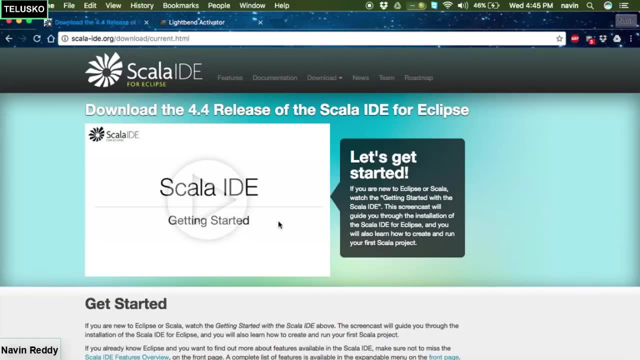 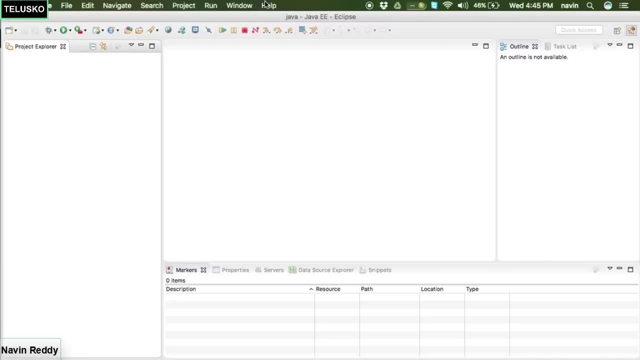 And even if I change the perspective to Scala, there's no option of Scala here. So for that we have to go to downloads and latest table. You just have to select this year U R L here, copy it and go to help. go to install new software in your Eclipse and paste. 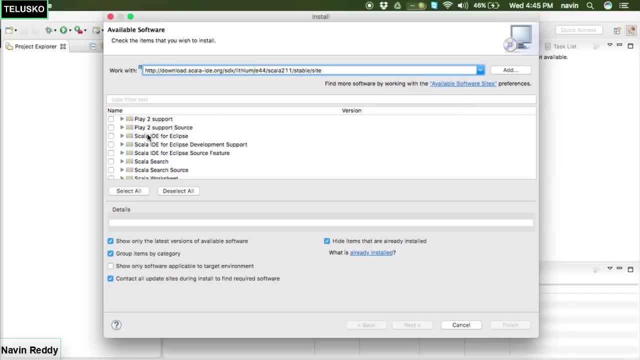 that URL here. So once you paste it here it will give you, it will show you all those options and which two things you have to install. You have to install the Scala IDE for Eclipse and you have to install Scala worksheet. Again, we'll talk about worksheet bit later. 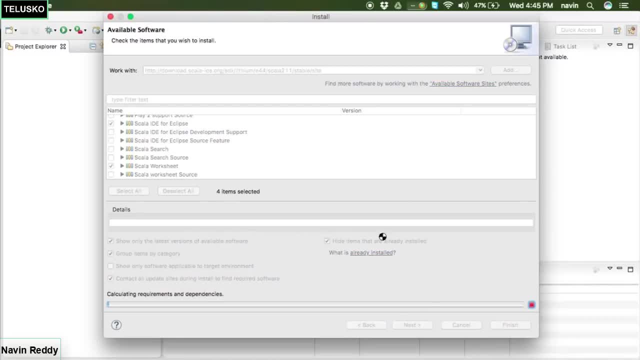 Select those two, click on next. It will download this stuff for you, and then you have to say next, next, and your Scala will be installed On your Eclipse. Now, once you install Scala on Eclipse, your Eclipse will look like this: okay, 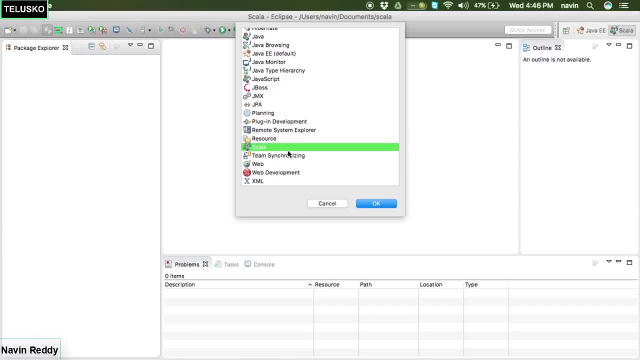 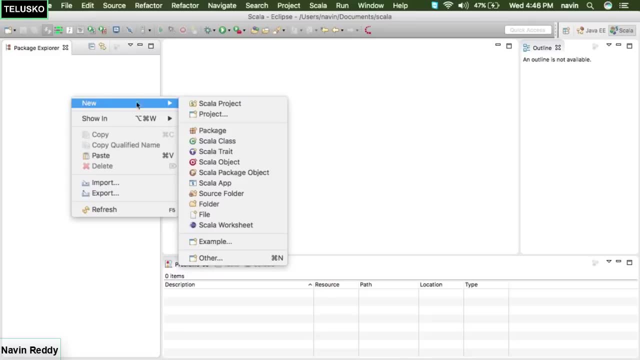 And if you open the perspective you can see you will get Scala there. You just have to click on okay and you will get a Scala perspective here And now. if you right click on your project, we'll say new and you got the option of Scala. 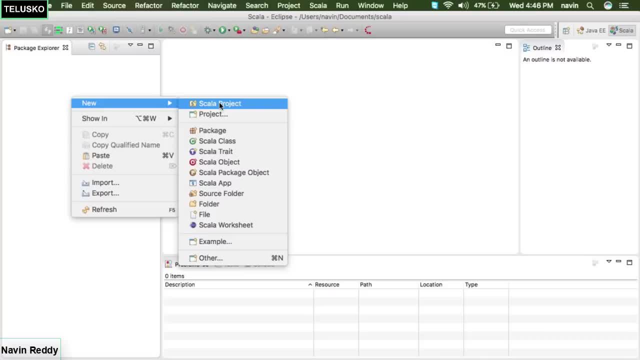 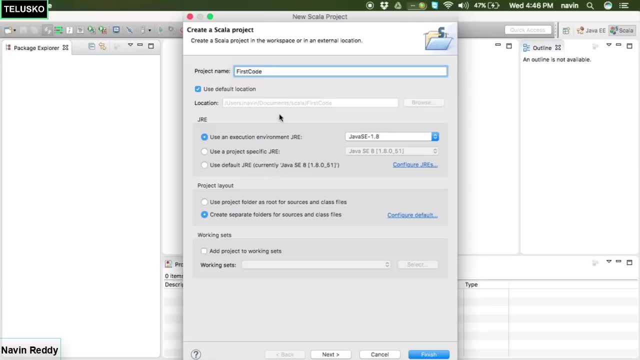 project. Now, this is possible only when you have downloaded the Scala plugin. So click on Scala project. You can give any name, You can give any code and you can see it says runtime environment is Java SE. I mean, that's awesome, right. 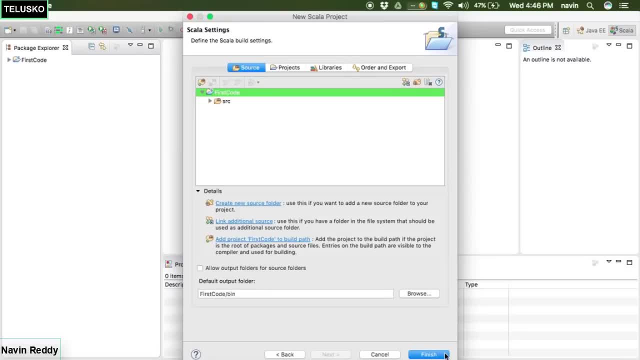 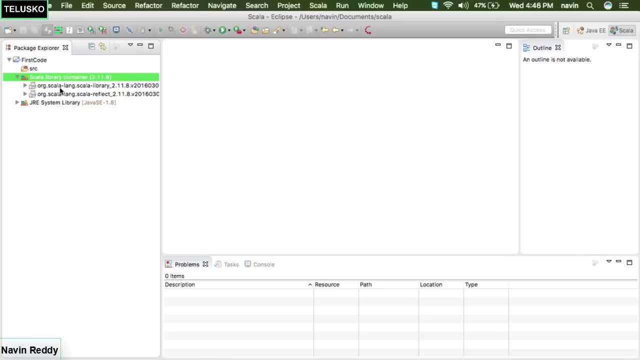 Scala works on JVM. What else we need? Click on next and click on finish. You've got your first Scala project. So you can see it has two things. It has certain. it has certain libraries for Scala. It has certain libraries for Java. 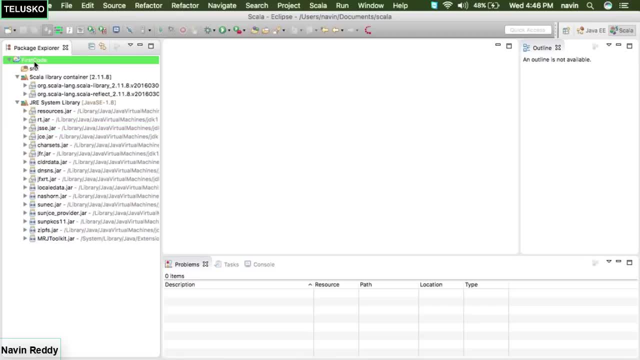 That means you can write Scala code inside this. You can also write a Java code inside this, So you can write both the codes in one project, And that's why I'm very excited for this. Okay, So let's say, if you are a web developer and you're working on Spring Framework, you're 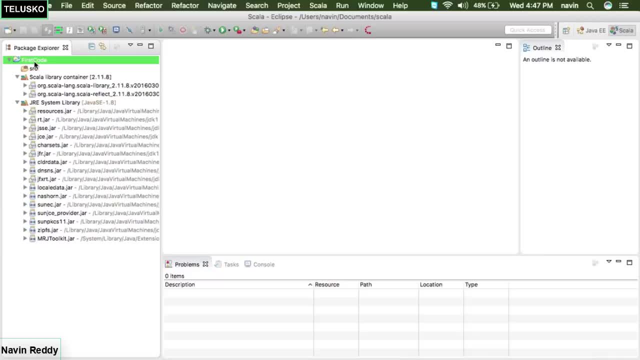 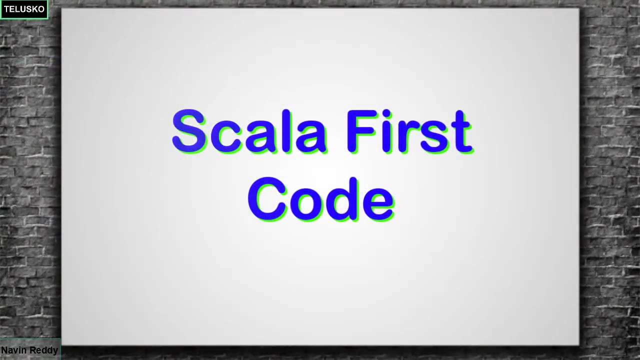 working on Hibernate, you can also use Scala in your web application. Okay, so that's something which is awesome about Scala. So that's our first project. In the next video, we'll talk about how to write our first code. So, once we have created the project- and it is here- 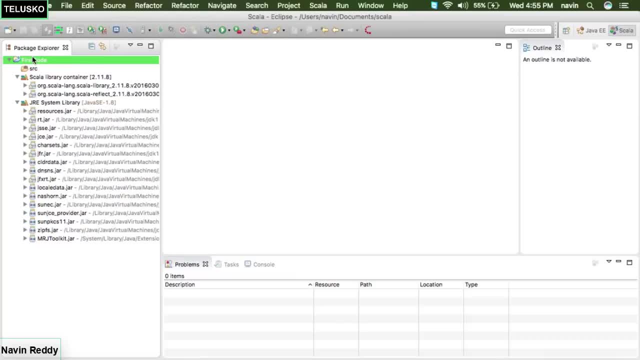 Now what I need is: Let's let's write some code, and we all are excited for the first code in Scala, right? In fact, I'm excited to tell you that. So what we'll do is now, if you, if you are from Java background, you know how to create. 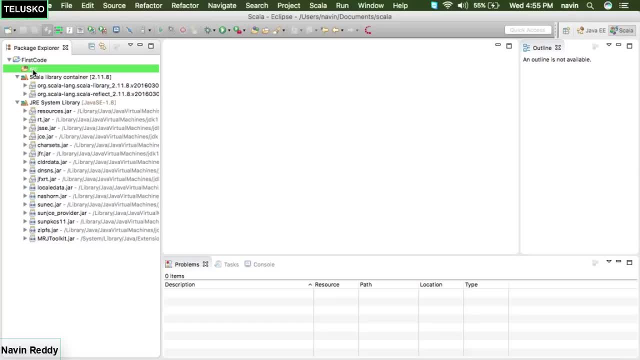 a new class and how to write hello world. right, And we cannot live without hello world. It doesn't matter which language you learn- maybe C, C++, Java- The first code you write is always hello world. But in Scala what we'll do is, I mean, we'll write hello world, don't worry. 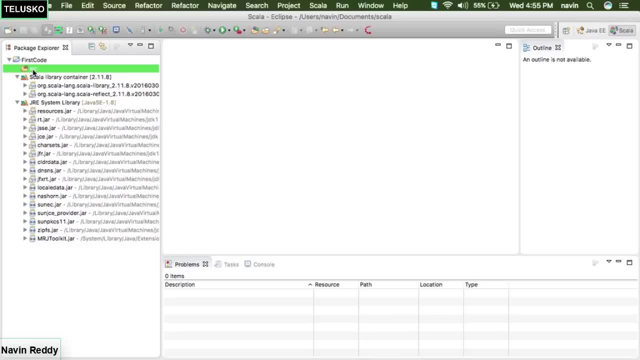 Okay, We'll write hello world, But we'll not write. See, We'll write hello world in C programming. What we have to do, We have to type Hold on. What we have to type, We have to type: hash include. 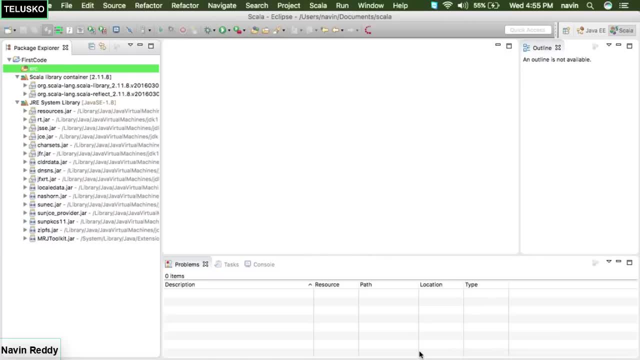 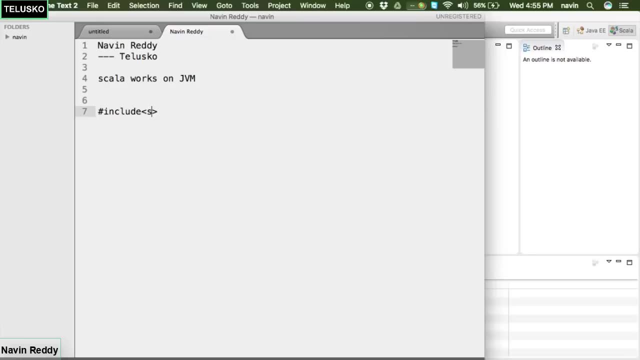 We have to mention. Be with me, Okay. So when you say in C programming, the way you write, you write your, you write your code is you have to write hash include. Then you have to say stdioh, right. 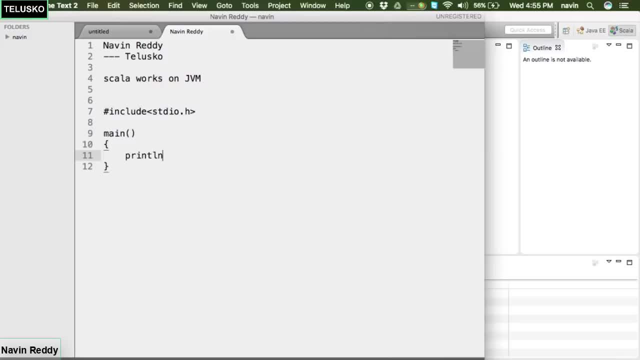 And then we have to mention a main function. Then the main function: you can write printf and in printf we can print hello world. Just imagine how many lines of code we are writing here. Can you see that We are writing hello world? How many lines of code we have there. 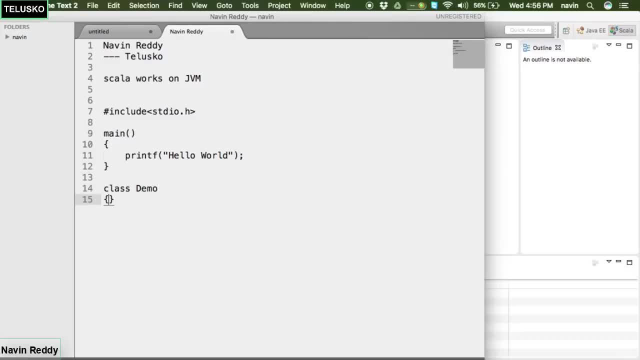 Now, when it comes to Java, what we do? we create a class. we create, let's say, the class name is demo. we write public static void main right And then we'll say string a. Then what we do next? 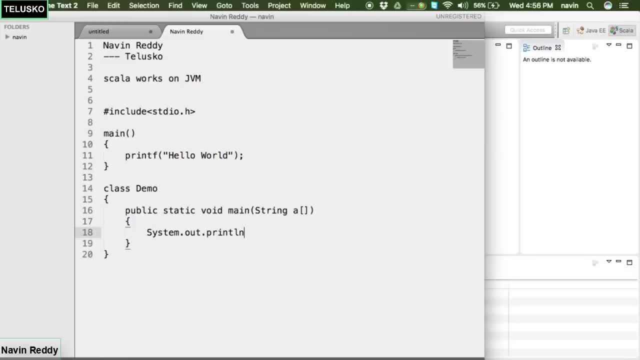 We say systemoutprintln, we say hello world. See, the only thing I mean just to print hello world. we have to write so much of lines of code, right? So when it comes to C programming, we have to write five lines of code. 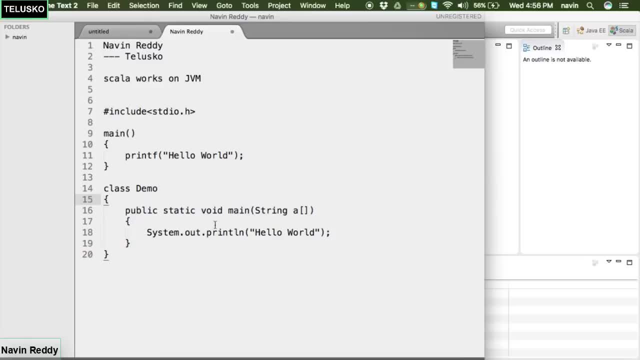 When it comes to Java, we have to write again six lines of code. Is it six? Yeah, maybe. So six lines of code right Now. just imagine, if you want to do this in Scala, why to write this stuff with this much? 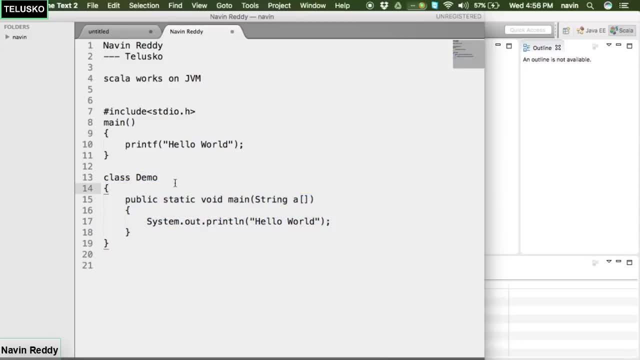 of code. right, Because this is a boilerplate code. Now, what happens is when somebody says, okay, let's say I'm going to my native place next month, and then let's say in my native place, I have my cousins there. Let's say they're from different field and they say, hey, Navin, what you do. 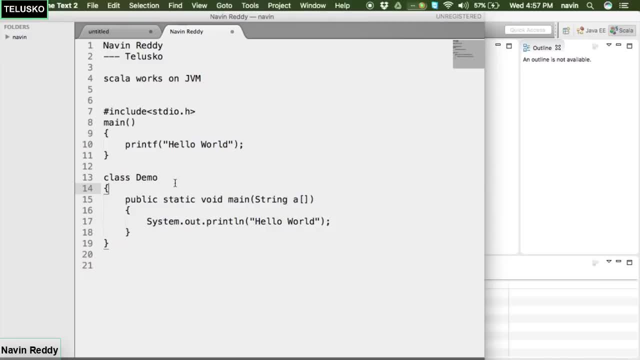 I will say, okay, I teach Java. What do you teach? I teach Java. So if they ask me, can you explain me one example in Java, I will say, okay, fine, Of course. I will start with hello world, right. 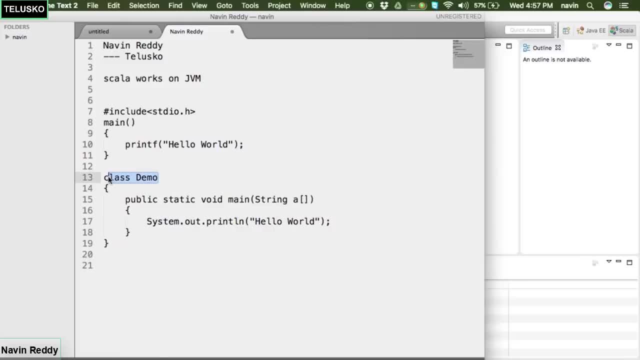 So what I will do, I will tell them okay. first we have to create a class demo. What is class? We'll see later. Then we have to write public static hold on these two things, we'll see later. 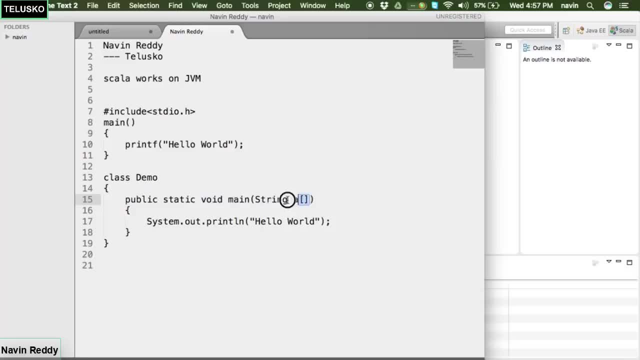 Then we write void main. that we'll see later why we have to do that. Then we have to create a string arguments- that we'll see later why we do that. We'll talk about systemoutprintln. We'll do that later. 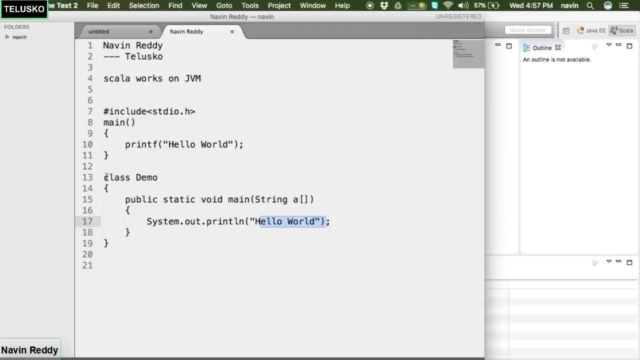 And that's how you print hello world. I mean, just imagine just to print hello world. we are skipping all this thing, we are not talking about all this stuff, right? So trust me, as a Java programmer, as a Java trainer especially, I find it very difficult. 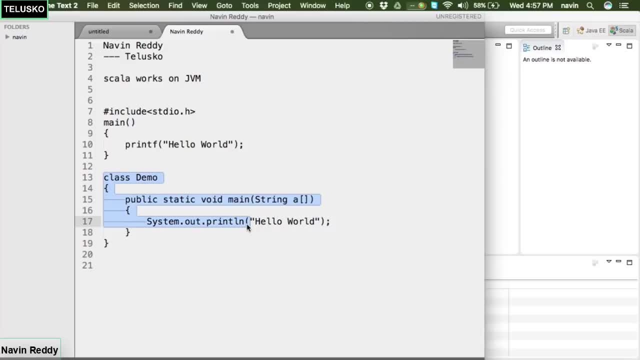 to write the first code. It's very easy. once you know the first code, it is very easy to learn Java. But just imagine that instance of teaching this part to a fresher or to the person who don't know Java. So what Scala says is: why to write all this code when you can do it very easily? 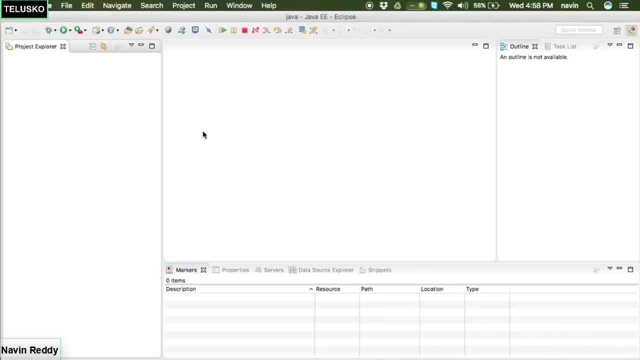 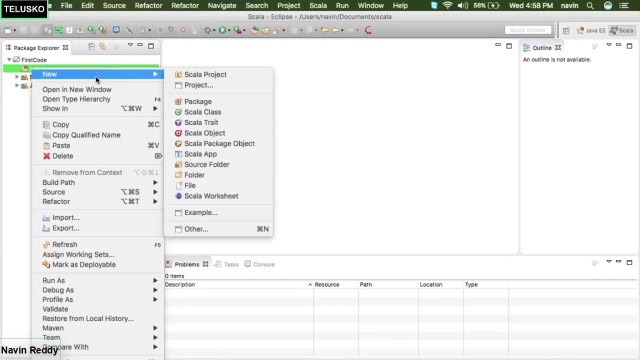 So in Scala, Scala provides you. if you want to teach someone Scala, don't go for all this stuff. What you can do is you can create a worksheet. Now, how to get a worksheet: Right click on your SRC, say new. there is an option of Scala worksheet. 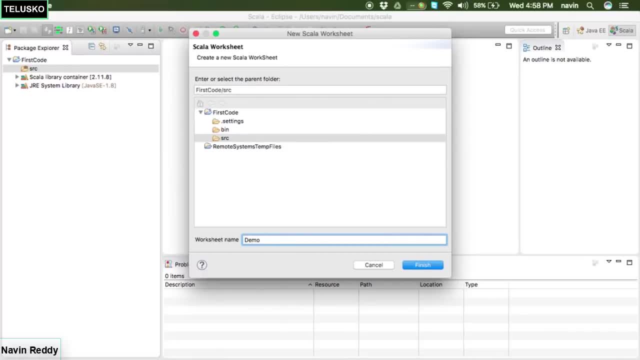 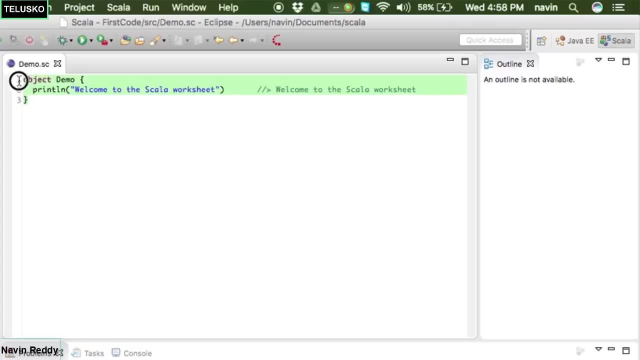 Now worksheet. let's name it anything. we'll say: this is demo finish And your worksheet will have this extension sc at the end. Now this is your worksheet looks like. again, just ignore this part. we'll not use this. As I mentioned, we'll not talk about anything. 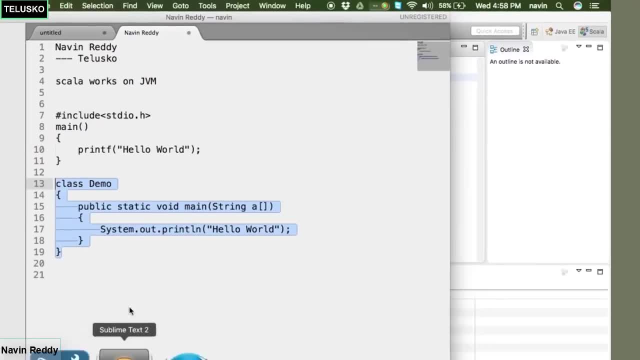 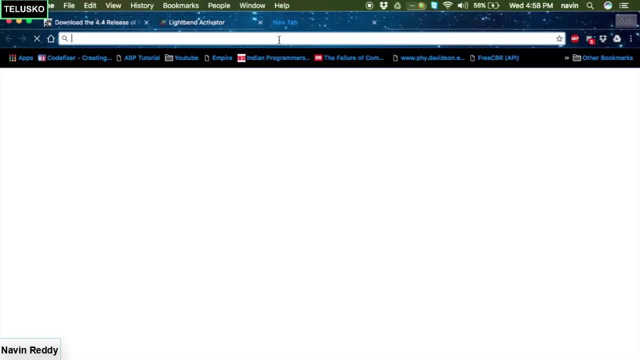 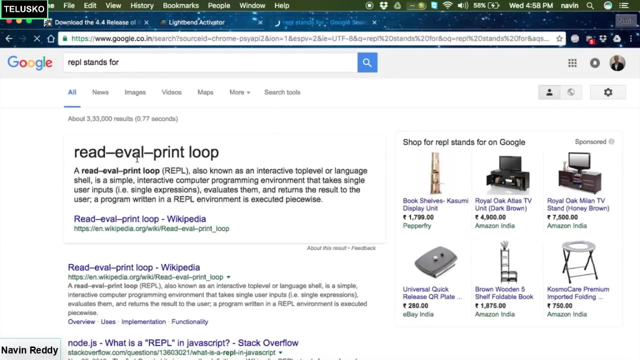 Now, Okay, So your Scala provides you something called as REPL. Okay, I again forgot the full form of that. let me just check it. the full form of REPL: REPL stands for it is read eval. yeah, so it is read eval. print loop. 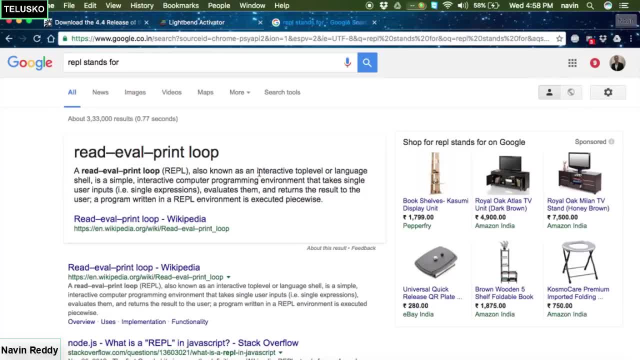 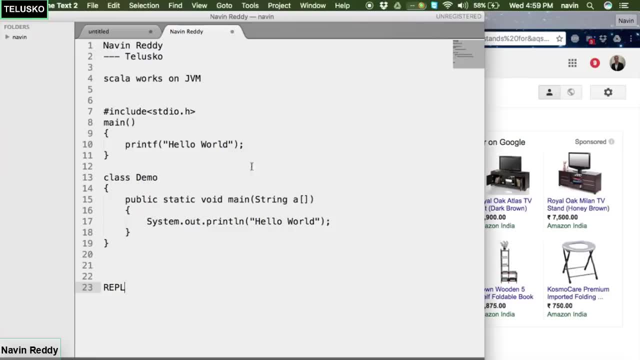 So it is something where you just have to type the lines, because it is normally used for interactive top level languages. Example: if you type a line, it will give you the output instantly. Okay, So let me joke. let me just go back to my Eclipse. 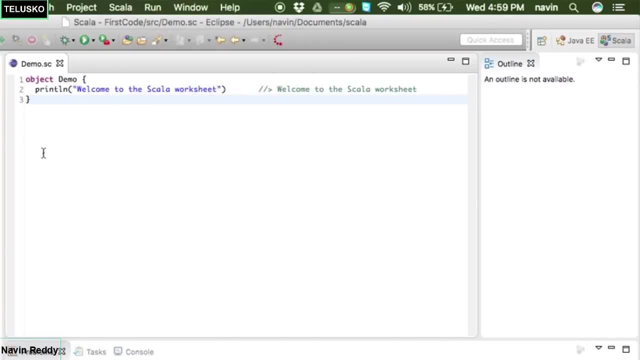 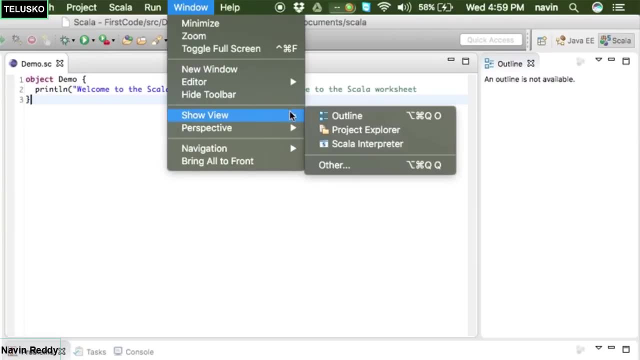 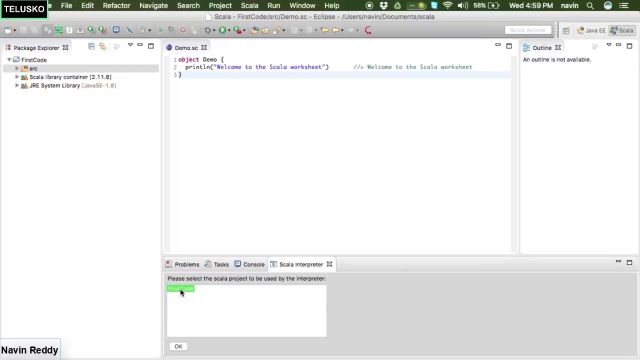 Now how to achieve that. For that we have to use again. we can do that here. there is no harm in that. What we can do is we can just go to window show view. we have an option of Scala interpreter. So if I click on Scala interpreter there, you can see it is asking you for the project. 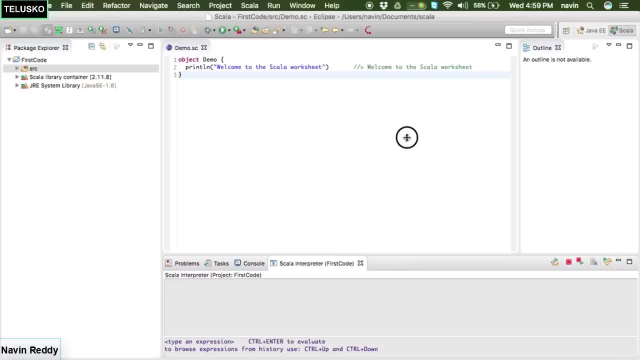 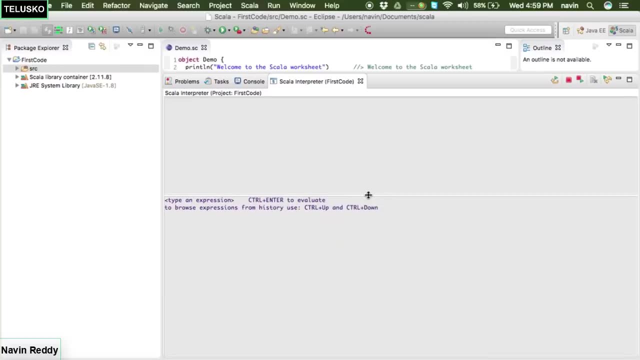 Okay, I am working with first project. click on: okay. Now, this thing here is a Scala interpreter. Okay, I will not use the worksheet which is provided. Let me use the interpreter. Now, how do we use it? To use Scala interpreter, you just have to click on this area. 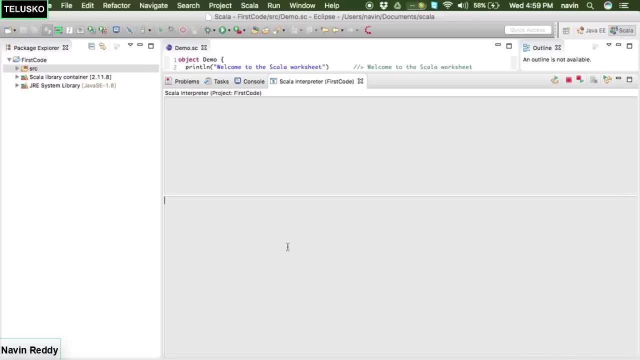 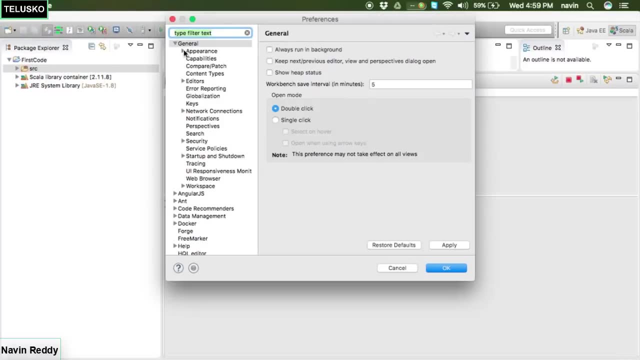 So this area is your typing area, where you will type your code. I don't know how to increase the font size of this. let me just increase the font size a bit. That's very. you know, this is the only thing which I hate about Eclipse. 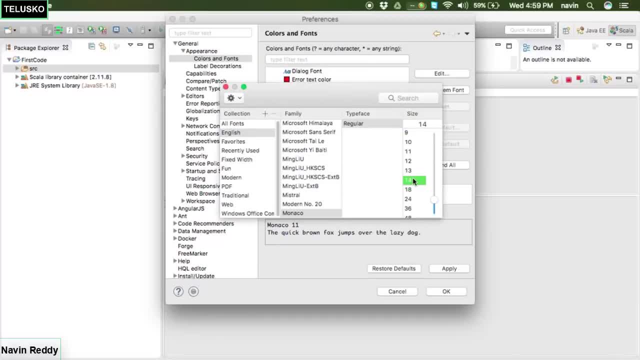 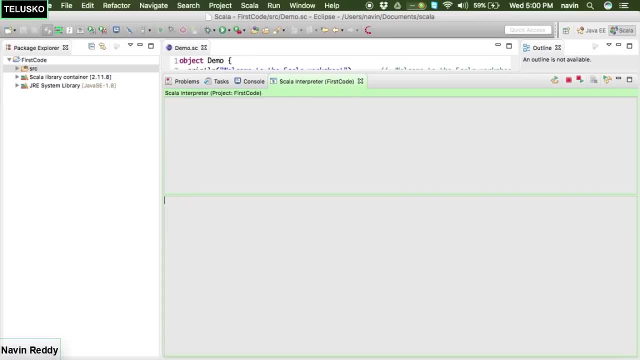 We have to just to edit the font size. you have to do lots of stuff, Okay, Okay. Okay. Okay, We got the same size. I don't know how to increase the font size of this. That's weird. I just hope you can see this font here. 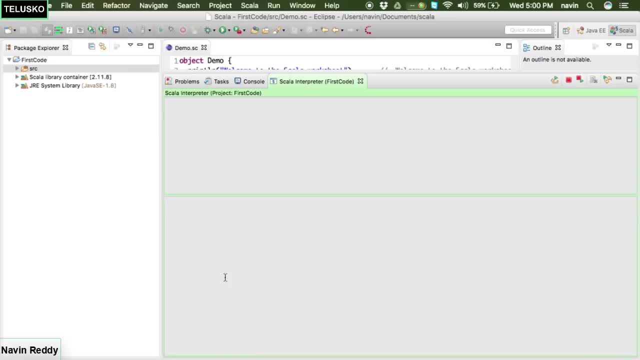 Let's. I am assuming that you can see the font. So what we will do now is: let's create, let's print hello world, or let's create a variable which prints hello world. So how do we do that in Scala? We simply say, okay, let me just print hello world. we will say hello world and once you 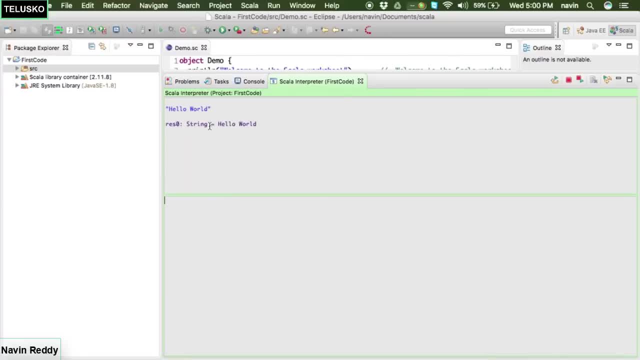 have typed it. just say control, enter. Can you see that? Just write hello world. you got your output here. You just have to type this stuff here and say control, enter. It will give you the output. We got our first code of hello world. 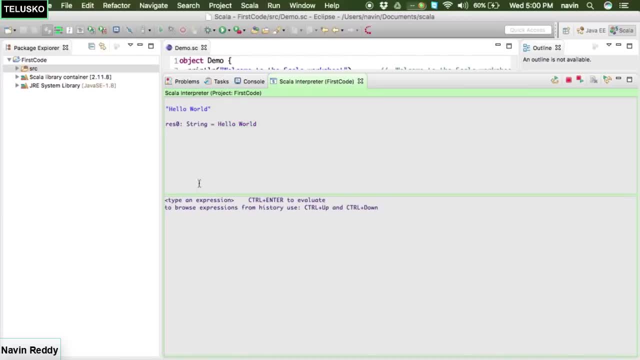 It is that simple in Scala: Just write hello world in double quotes. you will get your thing. If you write the hello world in single quote, will it work? Let's try. Yeah, you can see it is giving you error. So the only way to write hello world: 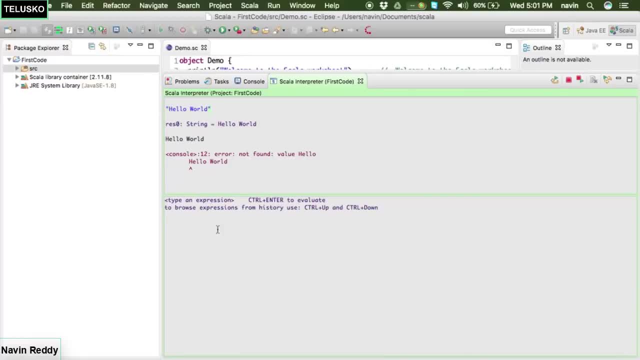 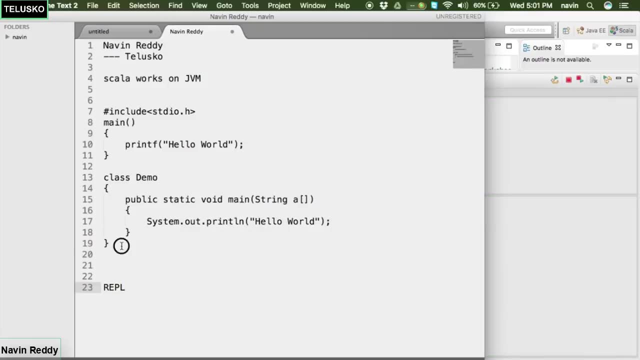 Is by using double quotes, and, as a Java programmer, we all know how to put string right. That's our first code. Can you believe it? We don't have to write any bullshit code which you write in Java. I mean all this thing. sorry for those words, but you don't have to write any of this boilerplate. 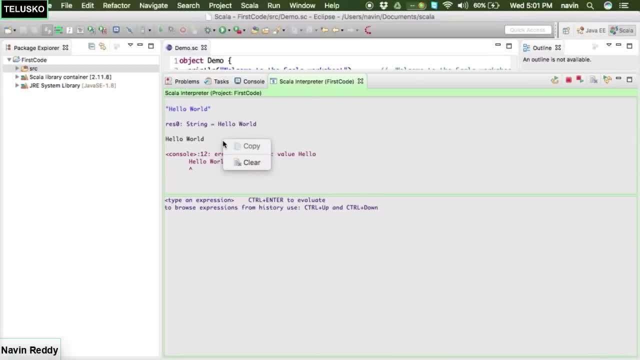 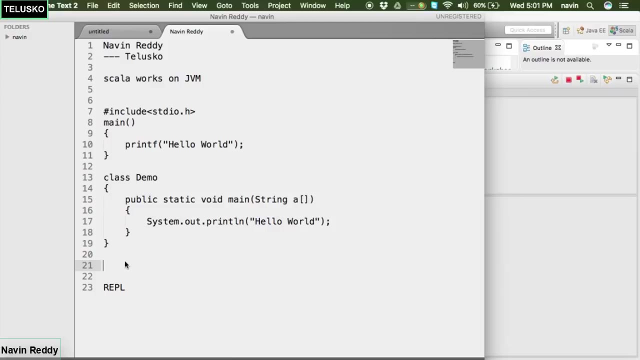 code here, right? So that's the awesomeness about Scala here. And how do we create variables in Scala now? So to create a variable normally when it comes to Java world, how do we create variables in Java? So by no mean, especially for Java people, by no mean I am saying Java is not good. 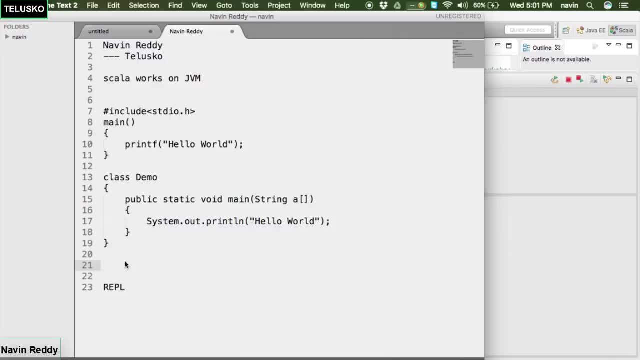 Come on, I am a Java developer myself. I am a Java trainer. I love Java. The only thing is, Scala has lots of features. It's just that I am showing you the importance of Scala so that you will get motivated. By no mean I am saying Java is bad. 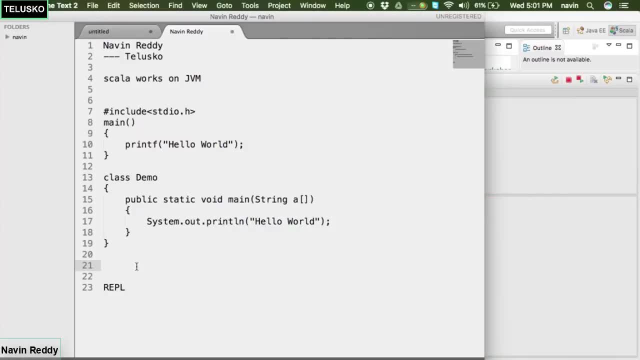 I love Java, So let me just come back to here. come back to this. So how do we create variables in Java? We say int i. If you want to create a variable in Java, we say int i. That's how we create a variable, right. 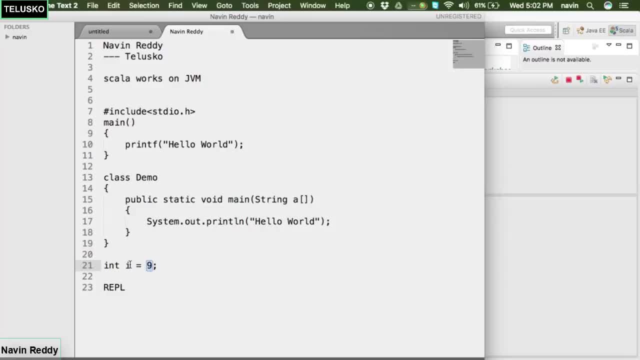 And that's how we assign a value. Now, when it comes to this i variable, you can see the first thing you are saying is int. You are not saying i. You can see that the first thing which we are saying is int, not i. 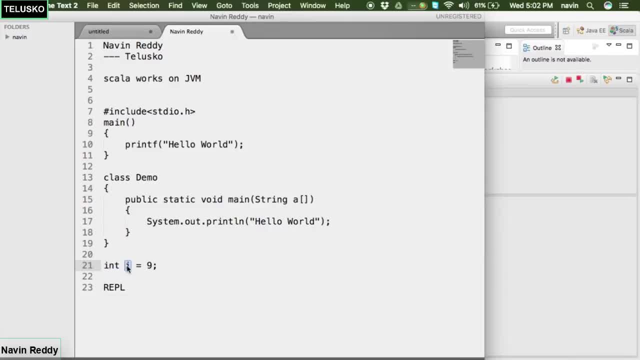 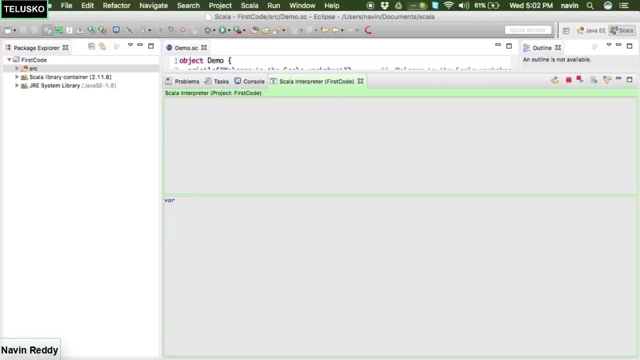 That means data type is more important than variable name. That is in Java, right In Scala, what it says. first you have to mention var and then mention the variable name and simply assign the value. You don't have to specify the key. 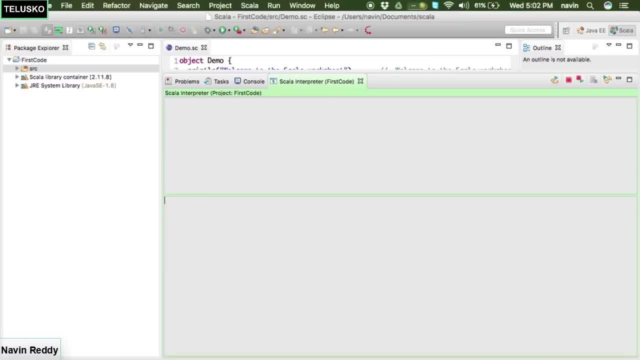 You don't have to specify the type. It is okay if you don't specify the type. If you say enter, you can see it will automatically detect the type of the variable which is int. So you can see we got 9 here, we got int. 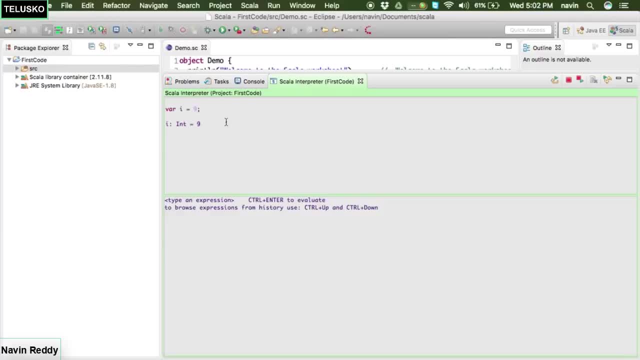 Okay, you don't have to specify the data type to work with it, But it's a good practice to specify data type, right? Because Java is strongly typed language or type safe language. We want Scala to be strongly safe. What I am saying. 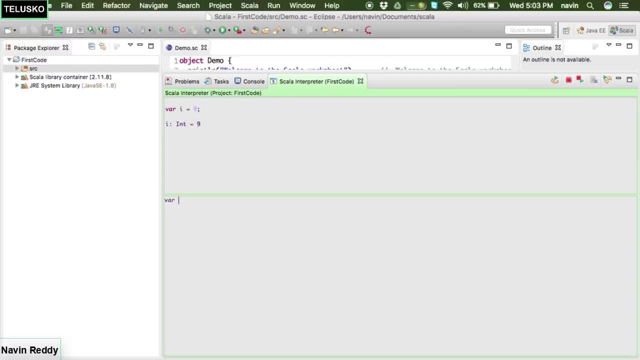 Strongly typed language. So what we can do, that is, let's say: let me get one more variable. we will say var j. Now how do we specify the type? Let's say num. How do we specify the type here? We will say colon. 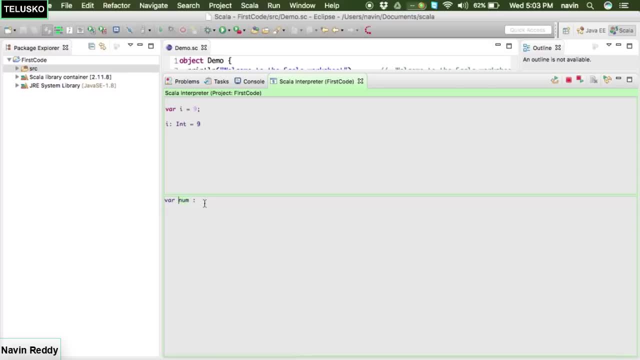 So I have to specify the var keyword and then we have to specify the variable name, Then we have to provide a colon where we specify the type of the variable, which is int, and then we will say 7.. Now again, you might find it bit difficult initially, but trust me, once you write 2 or 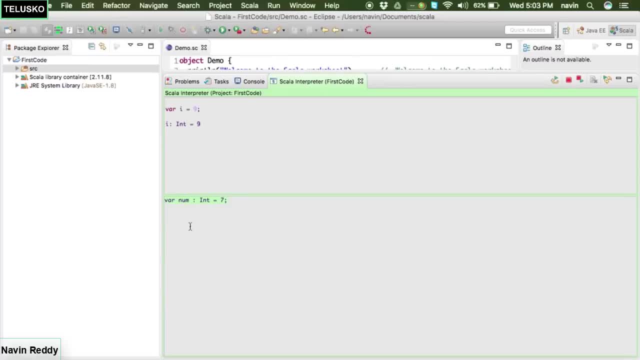 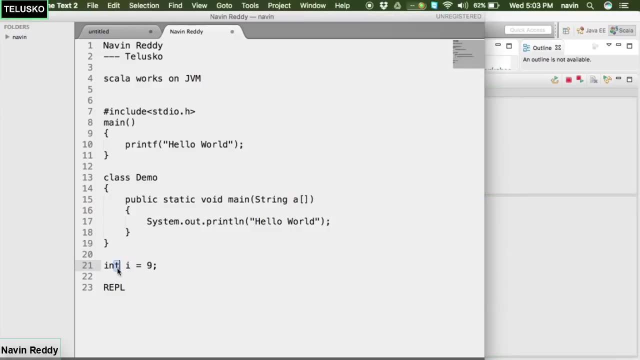 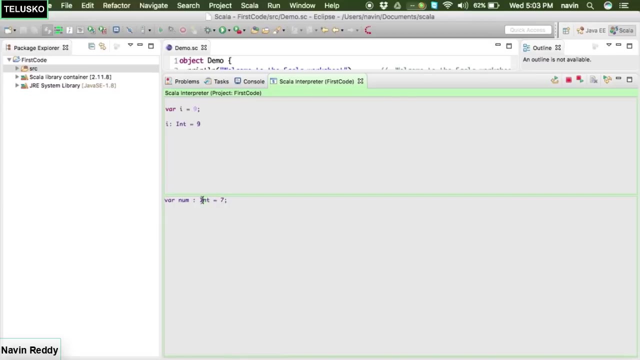 3 quotes. you will be very comfortable with this, Because Scala believes that variable name is more important than the data type. Java, data type is more important than variable name. In Scala, variable name is more important than the data type. That's why we write data type on the right side and variable name on the left side. 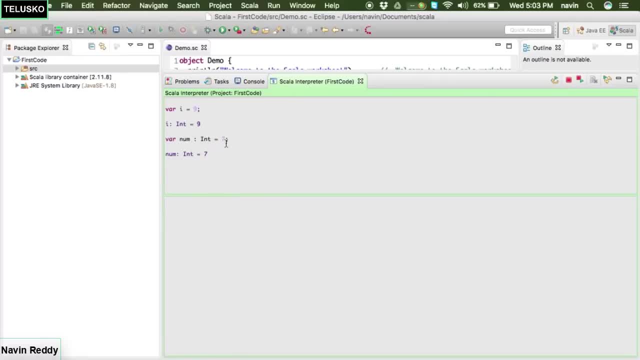 And to execute this, simply say control, enter. you get your output. So this is the statement and that's your output. So we got num int 7.. Now how do you perform actions here? Let's see how to perform action. So what we can simply do is now we have 2 variables. 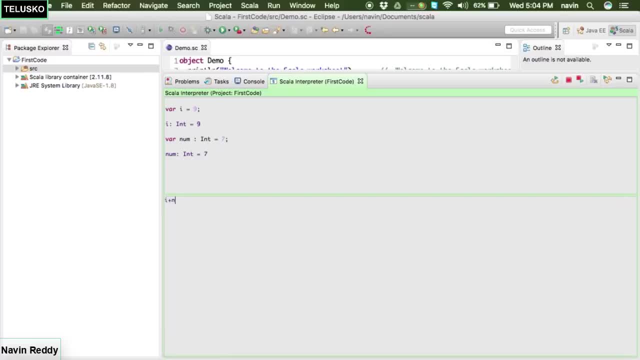 We have i and num So we can say i plus num. So when I say i plus num and control enter, you can see it has added both the elements. So we got 9 plus 7, which is 16.. This is REPL. 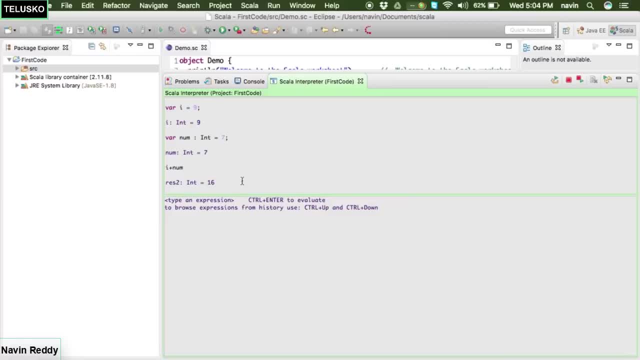 You can write statement by statement. it will give you the output like an interpret language. Ok, Ok, But later on we'll see how to create classes because, see, somewhere in your mind we have the concept of classes, object variables. We'll come back to that, but I want to show you some advanced thing. 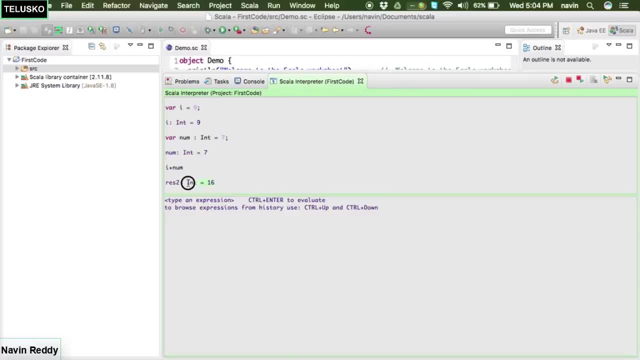 That's why I'm showing all this stuff to you. That's how you create, that's how you add 2 values. Ok, We can perform multiple operations here. We can also say i into num. It will give you the multiplication of it. 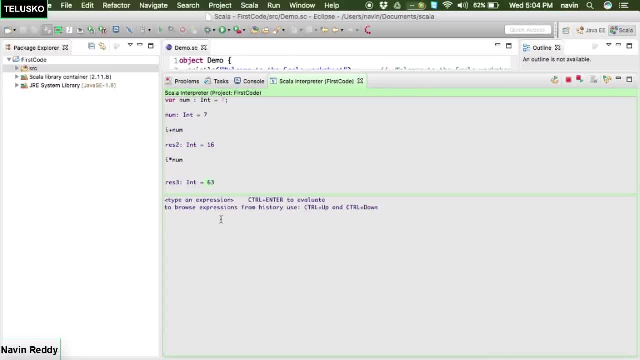 How to print control enter. we got the multiplication, which is 63. What else we can do here? That's how we can perform the operation. Now we can also create a string variable. Let's say I want to create a string variable as my name. 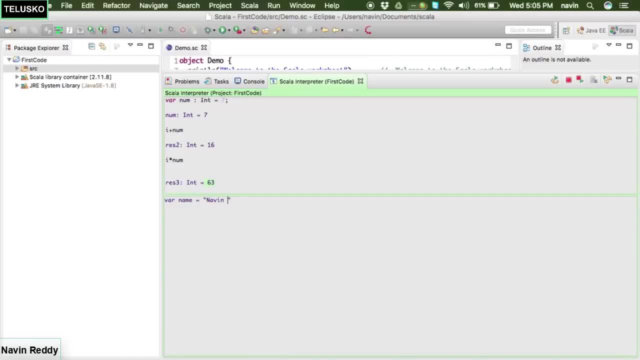 So we'll say var name equal to navin ready. Ok, we can also specify the type of it. So we can say: after name we can specify string. So that's how you specify the data type. we'll say control enter. So you can see we got a string which is navin ready here. 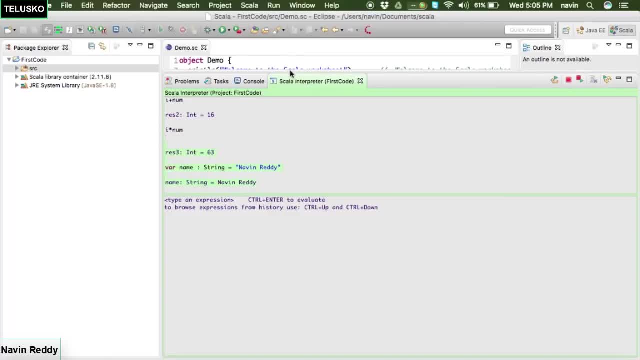 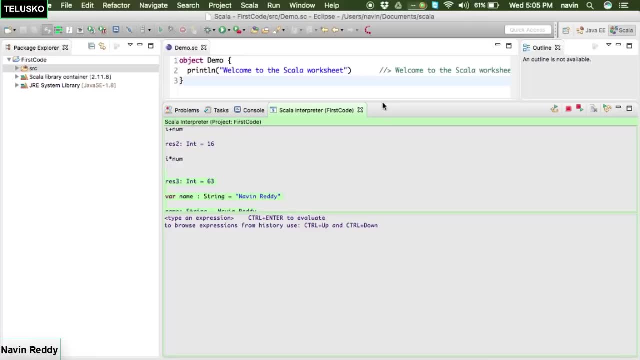 Again, if you cannot see the font size here, that's ok. After this, After this video, we'll type all our code in the worksheet above. So yeah, that's how you assign the value to a variable. So that's how you create a variable. 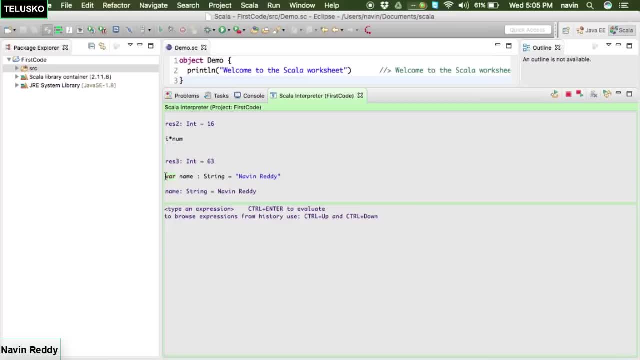 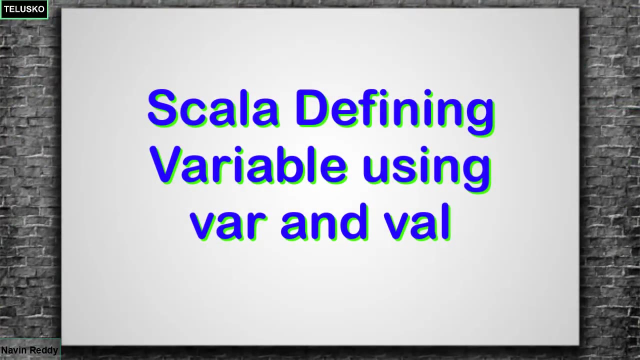 And yeah, that's your second coding video, where we talked about how to use worksheet, how to create variables, how to perform action. In the next video, We'll try to explore some more features in Scala, like constants and all those stuff. So that's it. 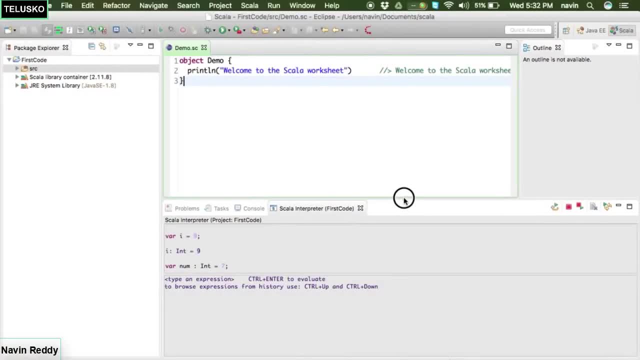 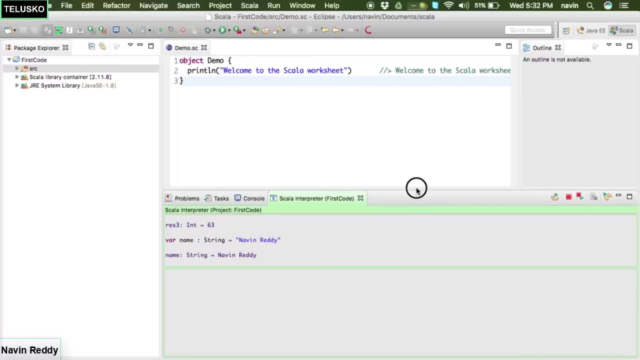 So in the last video we have talked about Scala interpret to write where we have, where we just have to write a line and then when you say control, enter, it will give you the output instantly. You don't have to write the full bunch of code to get the output. 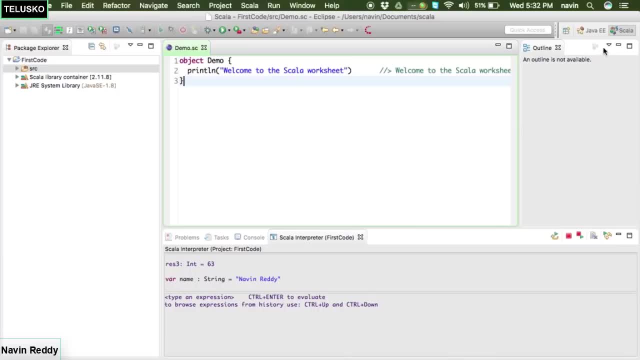 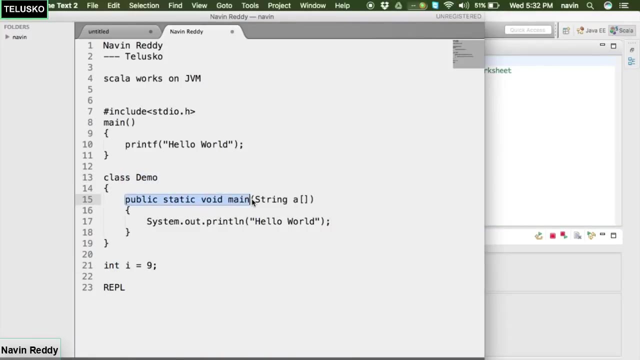 Now let's try to understand how to work with worksheet. Now, as you can see, We got a worksheet here, We got object demo. Now, why we have to do this is because you know, when it comes to Java, we have to write a class demo and then we have to mention the public static void main and the reason why. 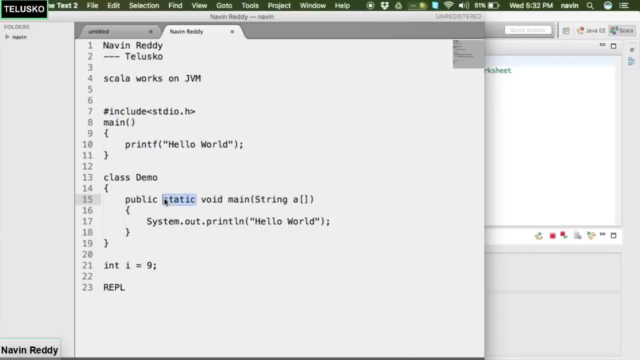 we do. why we use static main is because we don't need object to call main. because we don't. we cannot create object of main without calling main, So that's why we make it static. right Now, Scala says we don't need all those stuff. 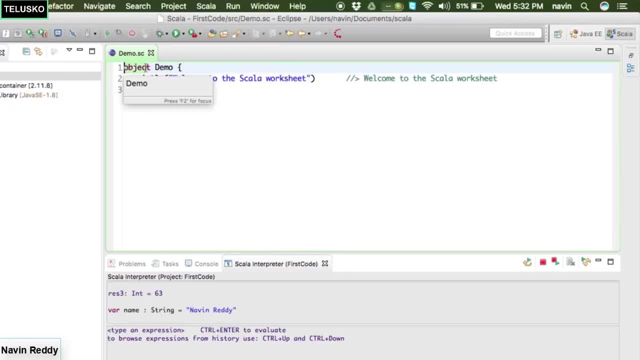 You simply say demo. I mean create object, OBJ, object demo. It's a real instance which we can directly use it. Okay, Again, we'll talk about this later, once we talk about the classes object concept. But here, whatever you type here, you will get instant answer here itself. 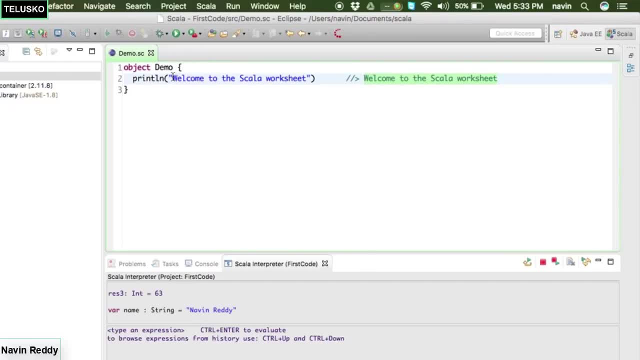 I mean, you don't have to go to console to see the output Example. let's say, if I say welcome to Scala worksheet, let's say this is hello world, and as soon as I say save it, you can see the output instantly there itself. You don't have to go to console and see the output. 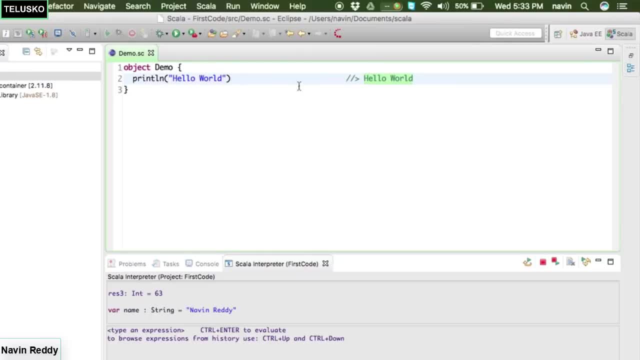 Okay, It is that awesome. Okay, now, what else? Let's say, I want to create a variable now. So the way we can create a variable is by saying var. Okay, var is used to create a variable and we can specify the variable name as num and. 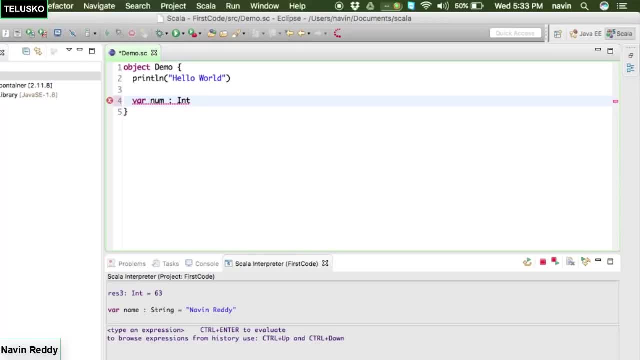 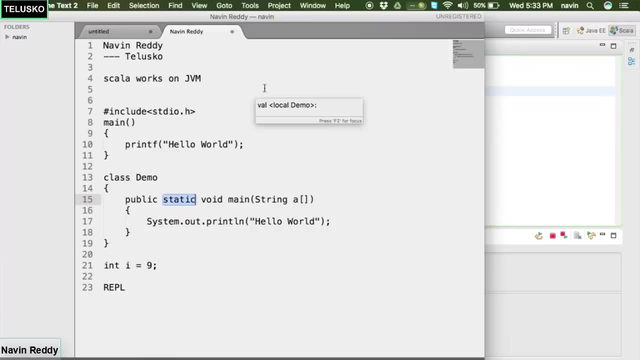 we have to provide the data type, using colon, and the type, which is int, and let's say 8.. Now, if you're thinking about Java, where we use int float, so normally what happens is in Java we have int, We have float, We have double. 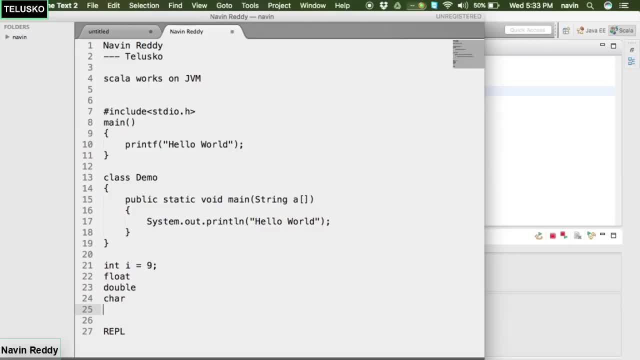 Now all these types, I mean in total we have 8, right, we have 8 types. We have short int, We have long, We have boolean. So if you talk about all this, this are called as, so this stuff are called as primitive data. 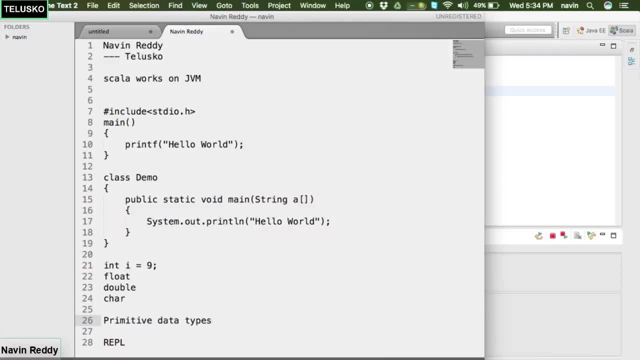 types and that's why Java is not purely object oriented. right, because in Java we still write int, float, which are coming from C programming. So Java is somewhere. you know, Because of data types, I mean because of primitive types, Java is not fully object oriented and 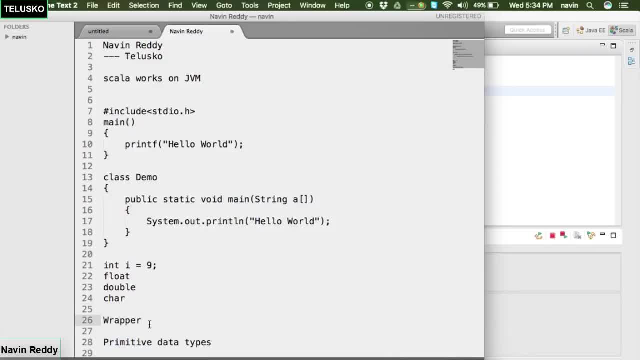 we still have VAPA classes to cover it. cover it up, right. So VAPA classes are like covers to this. So instead of using int in VAPA class, we write integer instead of float type, we write float class. instead of char, we write character class. 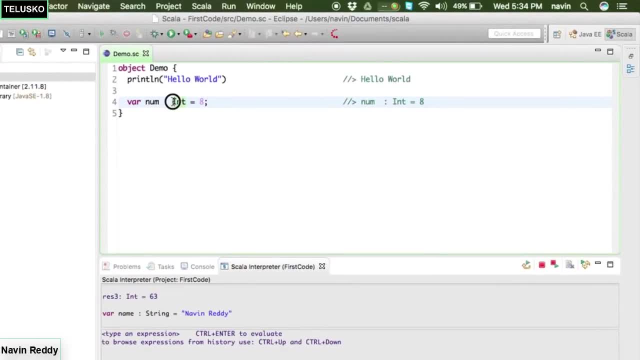 But in Scala everything is a class. in fact this int is also a class. so in Scala we don't have primitive variables. So this int is a class itself and this num is an object. okay, if you think that this is a primitive, no, it's a class. and this 8 is also an object in Scala. again, we will see. 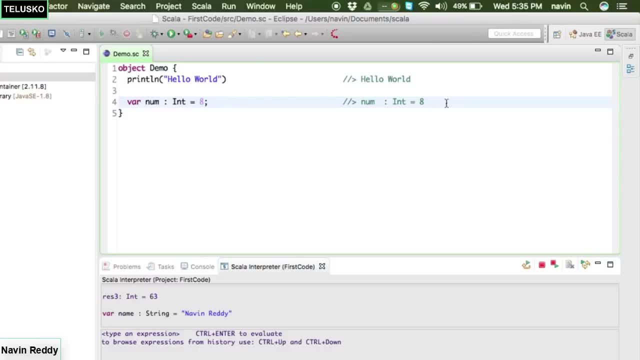 that how. that is an object and if you, if you can see that we are getting instant reply here and now we can print, we can say: print the value of num, let's see is it like working? and it works. You can see. we got the output as 8.. 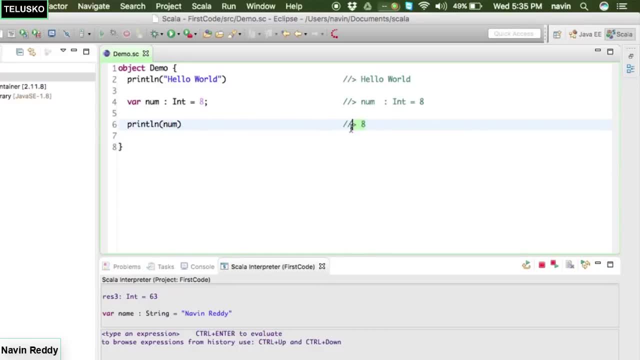 So when you print the value Of num, we got the output as 8.. Now what else we can do here? let's perform some operation. we will create one more variable. let's say time bin. let's say this is num1 and this is. we are printing num1 here. let's 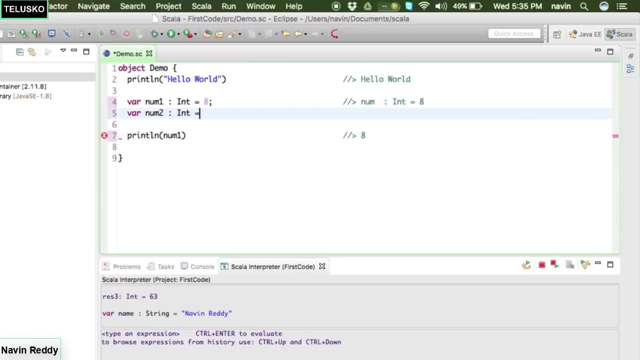 say, we are getting one more variable which is num2, colon int equal to 7 and we can perform the operation as num1 plus num2. again, we have seen this in the last video, right, but still, I want to do this Now. why I want to do this is because, even if I remove this semicolon, it works okay there. 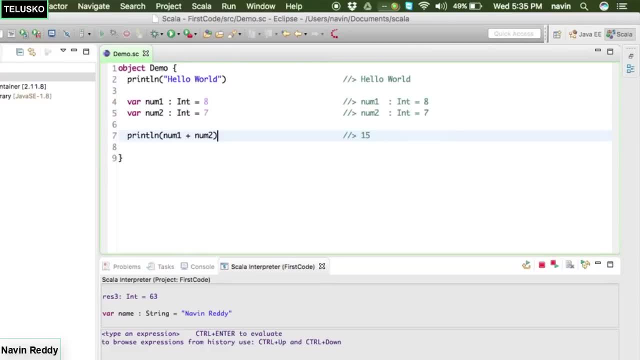 is no harm. you can see if I run this code now you are getting the output. that means in Scala we don't need semicolon as soon as your line ends, as soon as you can see there is no line, I mean there is no statement, I mean there is no characters or words ahead. 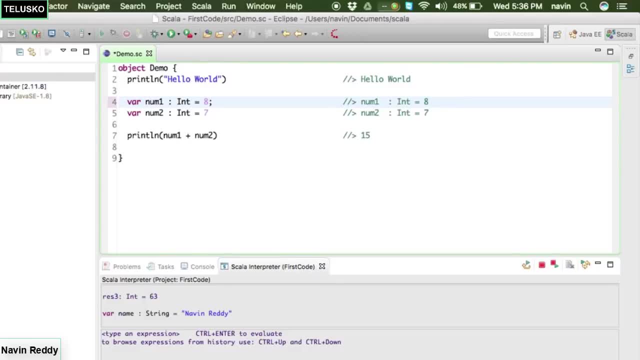 it will end the statement there itself. again, you can write, you can write semicolon or that is not composite right, because you don't have to give lots of pressure to your little finger Right to type that semicolon. so we just, we can simply say num1 plus num2 and you got. 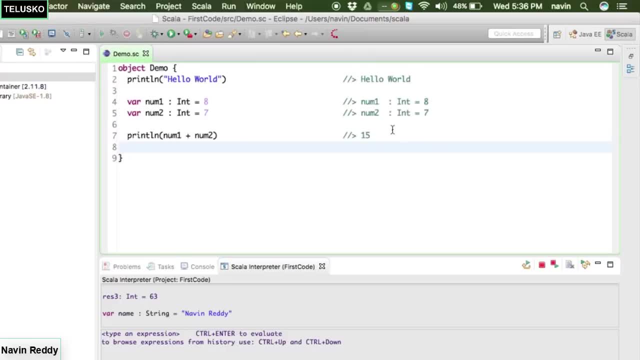 the output, simply say save. it will give you the output here itself. now what else we can do? in fact, I think Scala has copied this concept from Swift. I am not sure. okay, I am just guessing it, because if you learn Apple programming, Swift programming or in Swift, it will give. 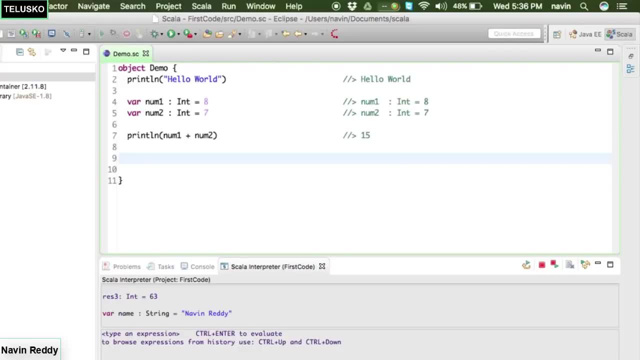 you output instantly. I guess it is called as workbook in Swift. I am not sure I forgot the point, But anyway, so we can add those two values. what else we can do here? we can define a string, we can define all the stuff. but let's say, if I can, I change the value of num1 if I assign. 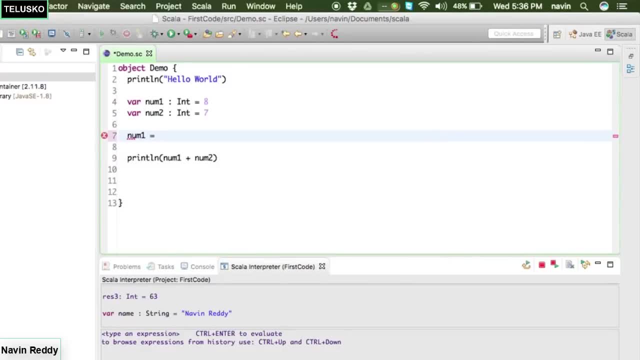 let's say, if I say num1, if I say num1 equal to 23, will it work? yes, you can change the value. right, you can see, we are able to change the value here. but what happens is in Scala. Scala believes that there should not be any mutation. now, what is mutation? means changing. 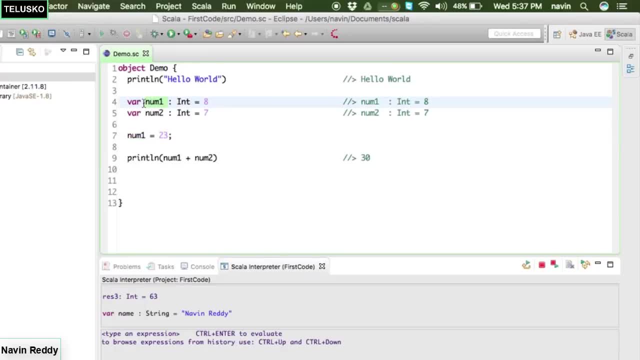 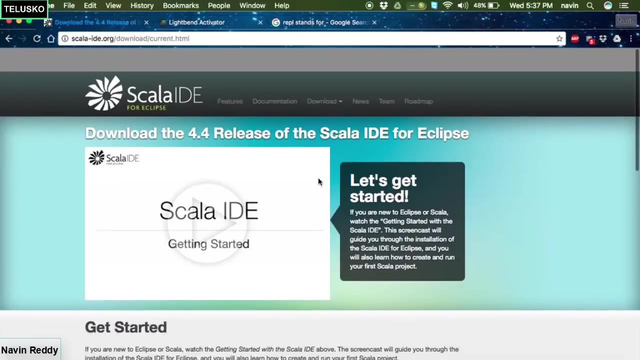 the variable value or changing the value of a type- I mean changing the value- is called as mutation and we should not do. mutation is because Scala believes in concurrency, as we have seen in the okay. so, as we have seen in the introduction of Scala, Scala believes: 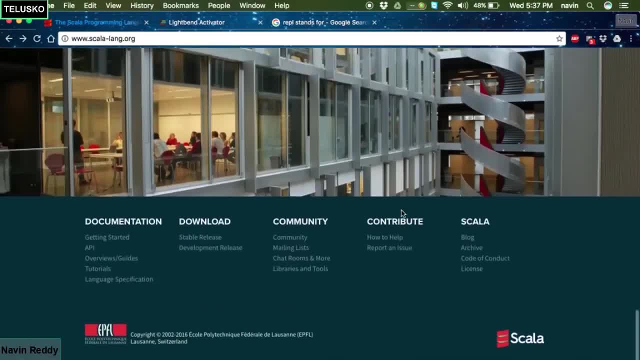 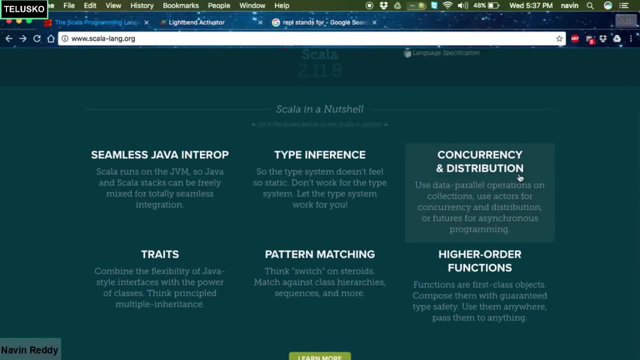 in. where is that? where is that? yeah, so Scala believes in concurrency. right, where it is, it goes here. So Scala believes in concurrency. So Scala believes in concurrency. So how to achieve concurrency when you have multiple threads working on the same variable? what happens is if one thread is changing the value, the other thread value will change. 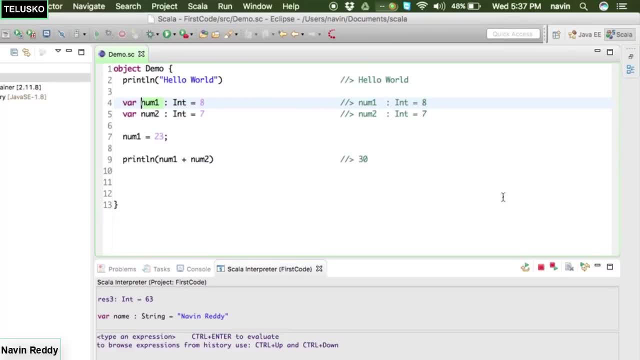 right and we don't do, we don't want to do that if there are multiple threads working on the same variable. we should not change the value of a variable. there should not be any mutation, because, see, change is good. right, change is good because the only thing which 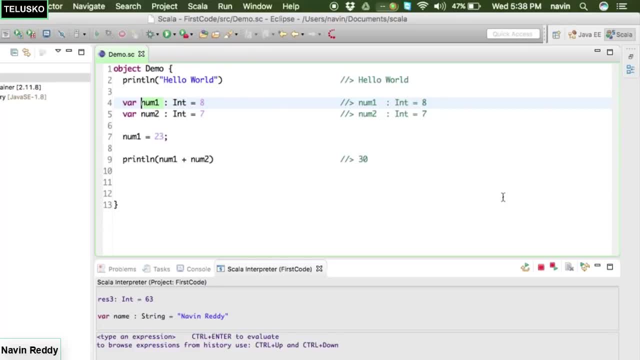 is constant is change, and sharing is good, Because sharing is scaring. so when there are multiple threads they can share with same variable. but changing and sharing, that is the real problem. So you should not create a variable which is changing and sharing at the same time, right? 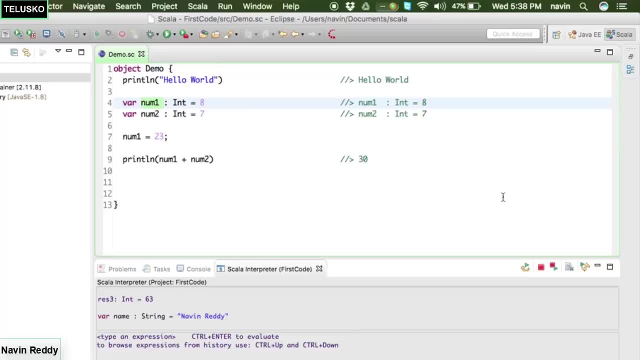 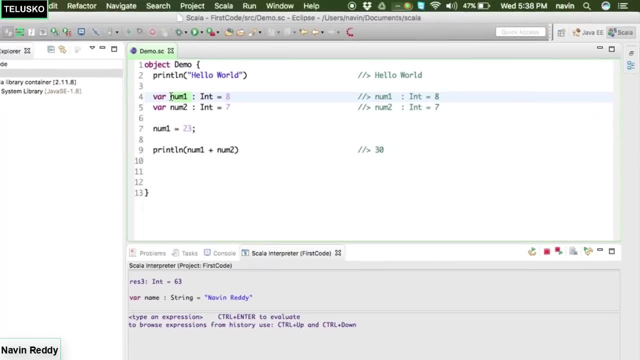 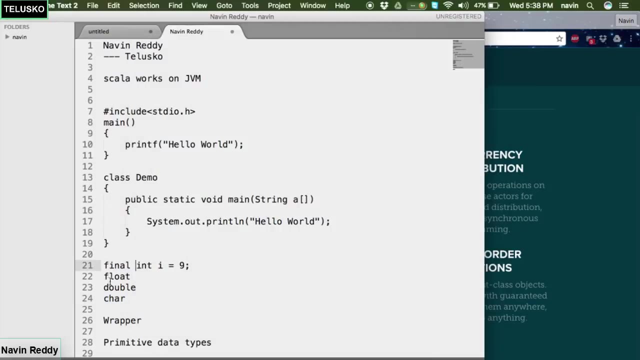 so Scala believes in concurrency. so how to achieve a constant value? I don't want, I don't want anyone to change the value of num1. now, how do we do that in Java? so we in Java, what we do is We simply say I want to create a final variable. so when you make a variable final, it means 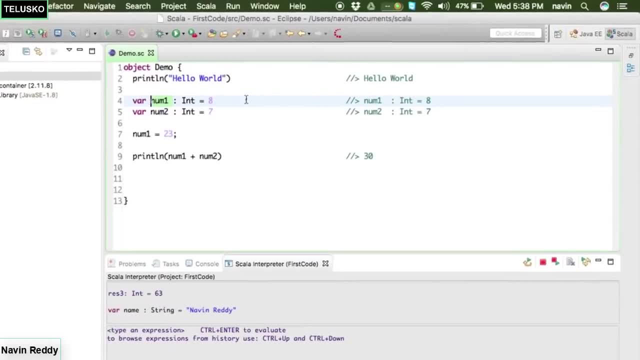 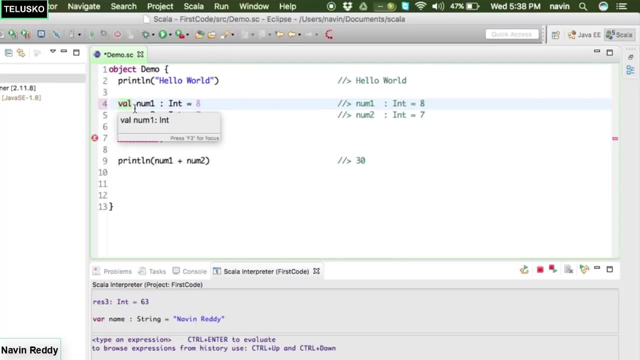 you cannot change the value of it in Scala, Scala goes ahead and say: okay, the only way to do that is by using val. so when you use a val to create a variable, it becomes a constant and you can see, once you specify val, you cannot change the value. so if I go to the error now, 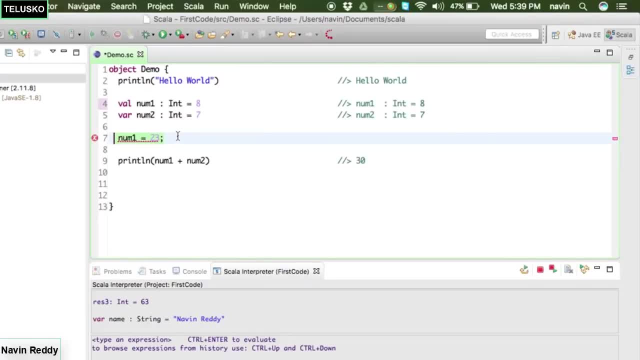 it says reassigning to val. it is not allowed. so if you say val, that means you can change the value. If you say val, you cannot change the value. so if you say val, it creates a constant and in future if you want to create any variable, always make it val again. you cannot change. 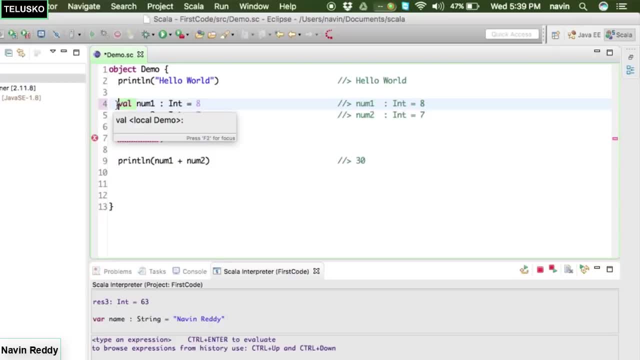 the value. but that's not the intention of Scala, right, Scala believes all the data should be constant, because we want to achieve concurrency. okay, but time being, since we are in the learning stage, we'll go for val. so if you say val, it gives you the instant output there and you. 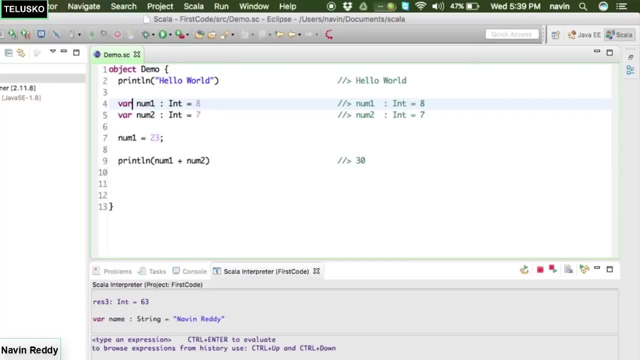 can see we got the output as 80. now what else? okay, so can I perform some operations. now, if you say, if you are performing this operation, you might be thinking: let me create a new variable for that. let me say: val result is equal to num1 plus num2. now, by any mean, let 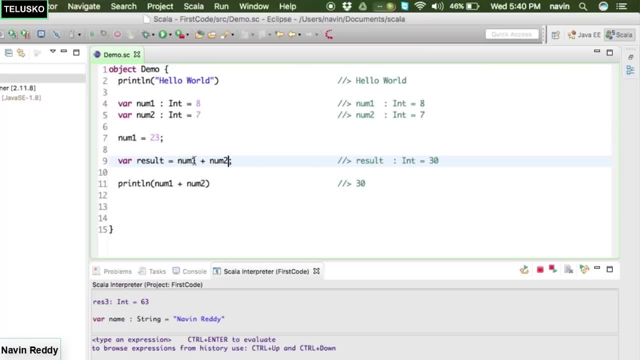 me just simplify it. I mean by any mean, if you are thinking that we are able to create two, okay, let me remove this stuff, let me, let me just make it very easy. initially, let's, let's do that. so if you are thinking that we are doing 8 plus 7, that means this: 8 is 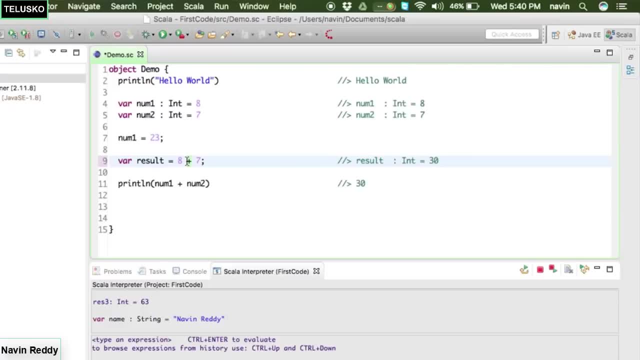 a value and this 7 is a operator, and that's not the case in Scala. everything is object. in Scala, everything is object and everything is a method. so this plus here is not a operator. okay, can you see that? there is a popup there, If you can see. 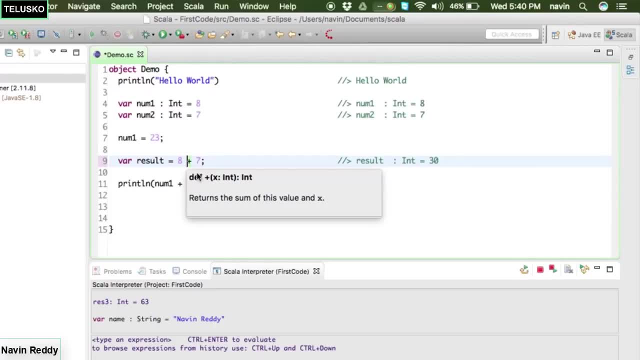 Def is the way you define a method or a function. so def is the way you define a function and the function name is plus. it is accepting a variable which is int. I mean it is accepting a int variable and it returns a int variable. now, if you are familiar with C++ programming, 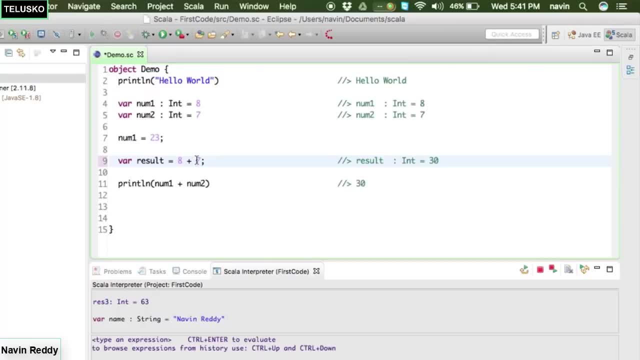 where we have operator overloading. this is what we are doing here. this plus here is not a operator, It's a function. let me repeat: plus is a function. I know you, you are in a bit of a shock now. it's because we don't have operator overloading in Java. and if you are comfortable with Java, 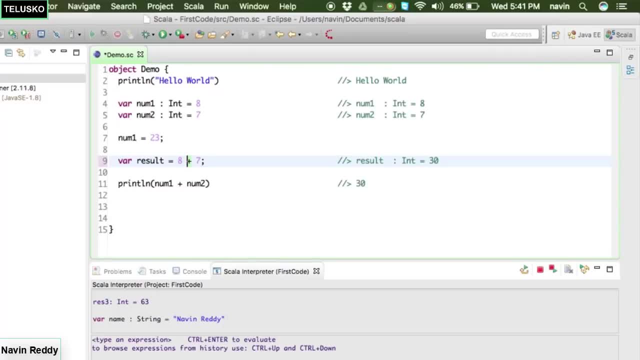 that means you know that in Java we don't use operator overloading, but in Scala we do, because Scala is also a functional programming. so this plus looks like an operator, but that's a method or a function- how it works. so imagine: 8 is an object and we are using a dot operator. 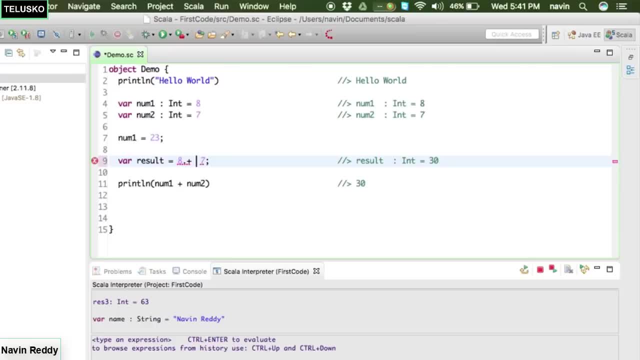 and the function name is plus and the addition operator, which is the addition operator, and this 7 we are passing as a parameter and you can see we are still getting the output. so we can see we got the output as 15. that means this 8 is an object, this dot is the operator. 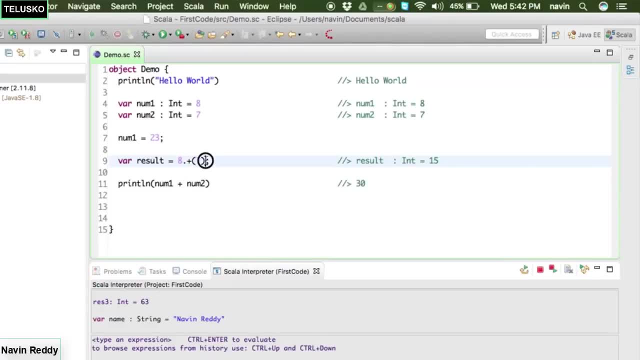 this plus is the function and this 7 is the parameter which you are passing in the function, and we are getting the value, which is 15.. Okay, So that is something awesome about Scala like it is this: this is both object oriented and a functional programming. 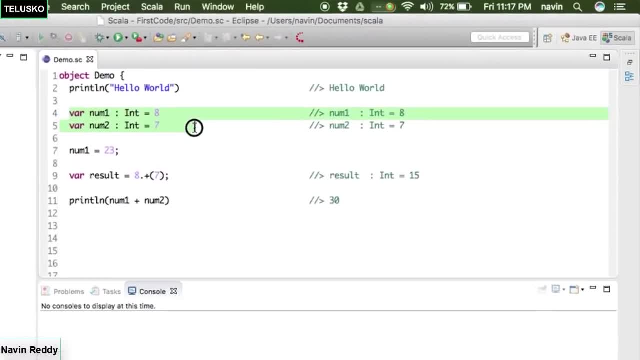 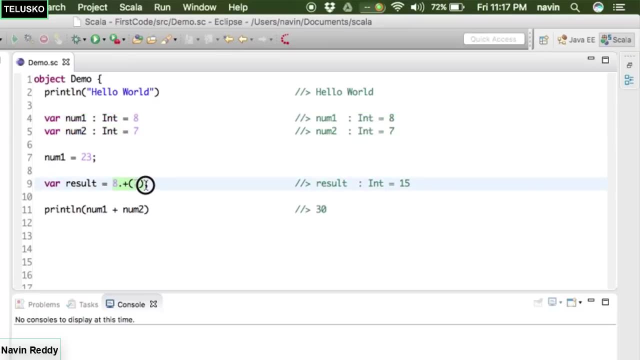 So the last video. we have talked about how to assign variables. I mean also how to create a variable, how to assign the values and how to add, to add to objects. now, when you say you are performing in some operation here, so when you thinking that, when you say 8 plus, 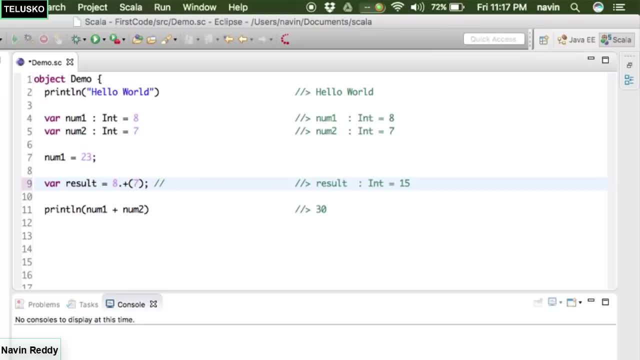 7.. So when you are saying 8, 8 plus 7, so that's not exactly 8 plus 7. what we are doing is so we don't have any plus operator. you know in Scala. so everything you will use is an method. so example: if you use plus there, that's a function. again, when I use method method, 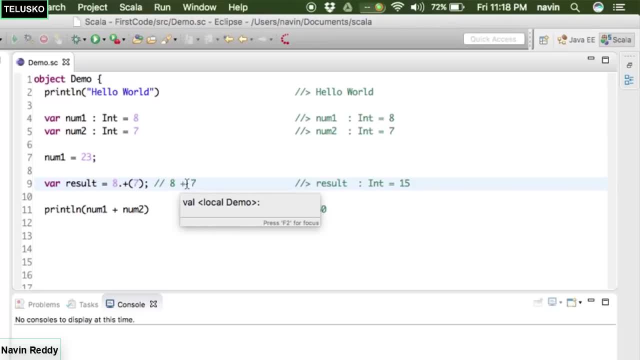 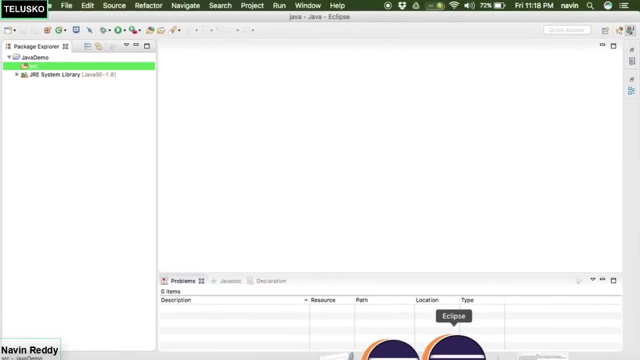 and function. that means the same right, not exactly same, but this is a function. so this plus operator here is a plus. I mean it's a function because Scala is also a functional programming. So that's how you, that's how it looks. So in this video we will let's talk about classes. so just to define that, I will open. 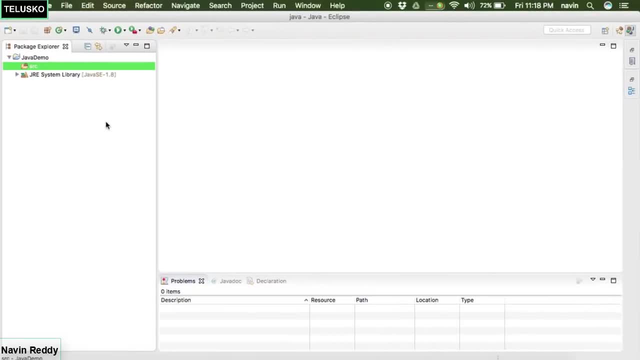 a Java. so I have two Eclipse in which I have, so in one I have Java, in another in another we have Scala. so in this Java part what I will do is I will create a class, because normally, as a Java programmer, we have this habit of creating a class right, and we'll go for typical. 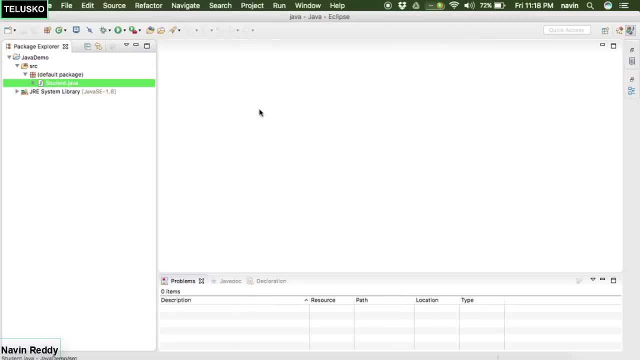 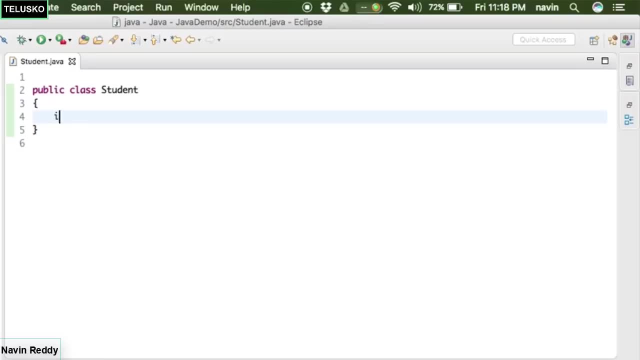 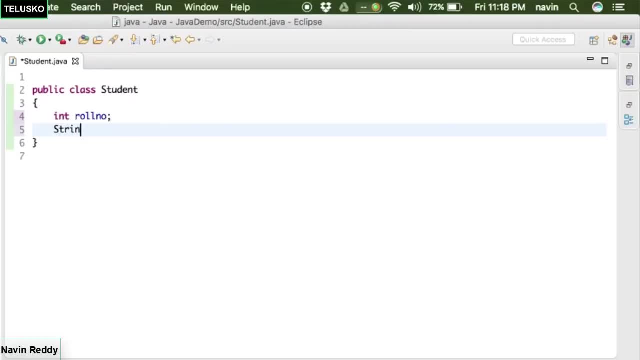 let's say only int roll number, then we have string name and then we have the last one as int marks. okay, so I just have this three variables here, and so normally if you don't mention the type of the access here, that means it's a, it's a package, private right. that means. 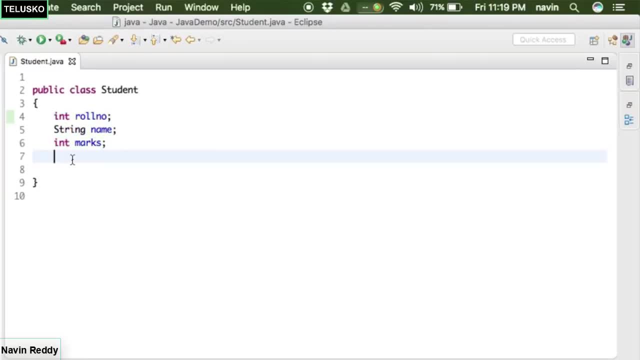 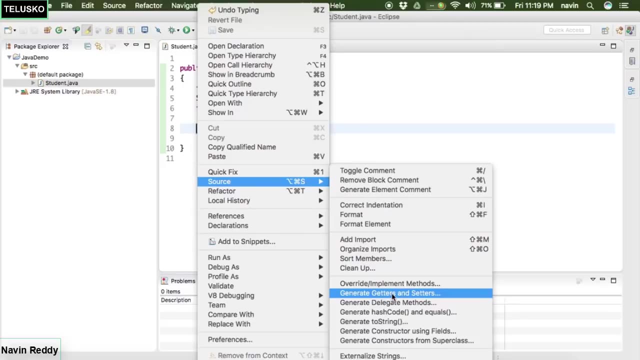 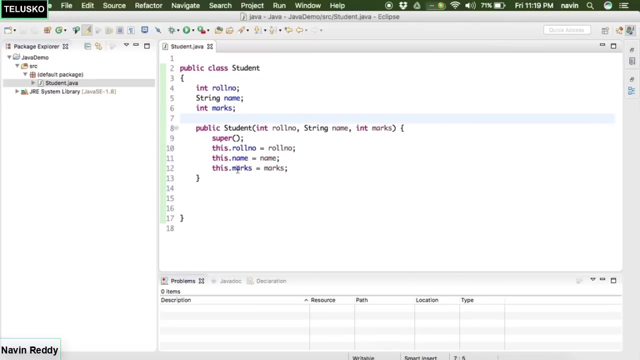 it is, it can be accessible inside the package itself. now, if I, if I want to construct a here, so I can say, right, like so, generate constructors with field, let's fetch all and okay, you got a constructor here, we can also assign. you know, we normally also use two other methods. 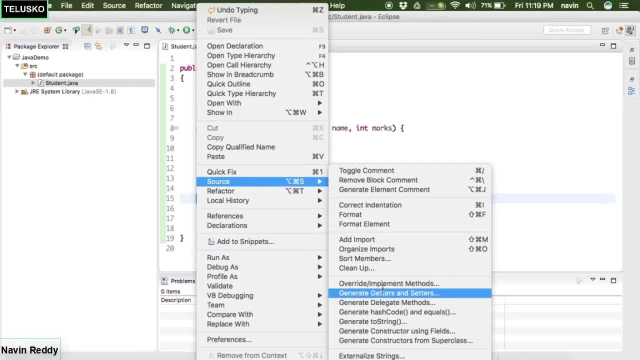 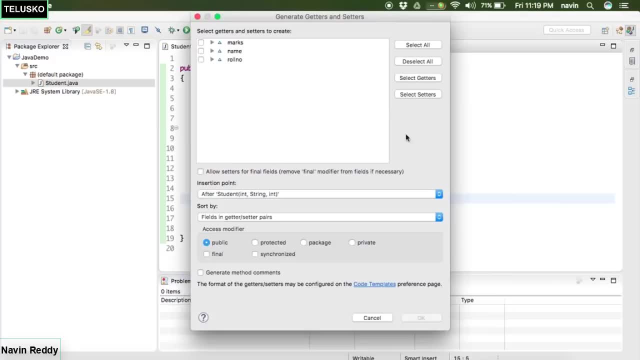 which is hash. I mean because we in Java we follow the concept of Java beans right. so in Java beans we have to make sure that you have getter and setter for that. so we have to use getters and setters because we want to implement Java beans here and what else. 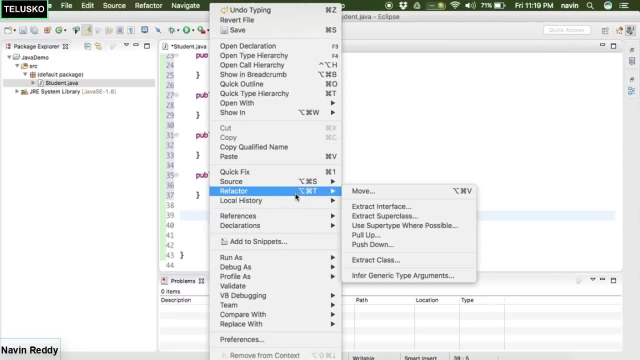 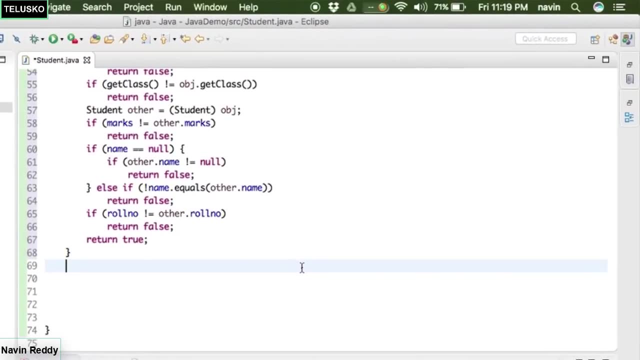 we need. we need one more thing, which is a hash function. I mean the hash code method. so we'll say: generate hash code and equals. so this is what we implement in Java, right? so if you want to achieve all this thing in Scala, you don't have to write all this line. 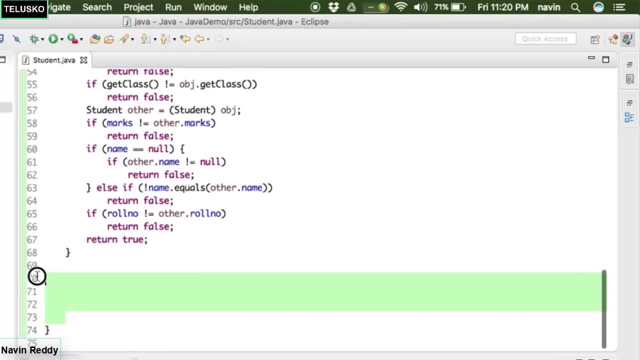 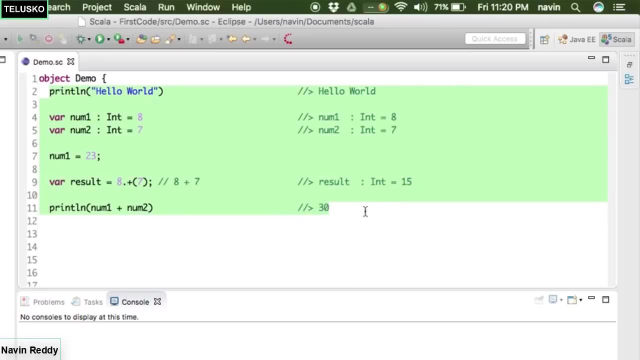 can you imagine how many lines of code we are writing here? we are writing approximately 70 lines of code. you can see that: 70 lines of code. let's do that in Scala how we create a class. so I will remove all this code here. let me get a class here. 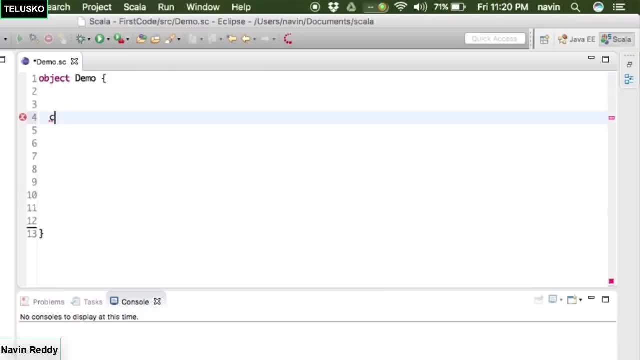 So, in order to create a class in Scala, we simply use a special keyword called as case and we use a class and we'll say: student and that's it, you got your class ready. okay, that's your class. I mean, of course, you will not trust me, right, but that's a class. now, this thing. 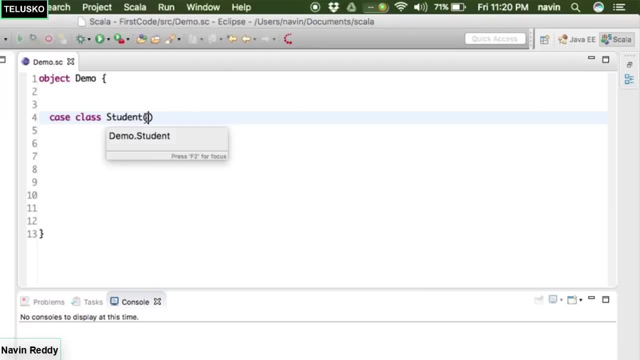 here, this round bracket, specify the constructor, so you don't have to create a class and then create a constructor. you can create a constructor as soon as you get a class. so you can specify the variables here. So I can say: I have the first variable. 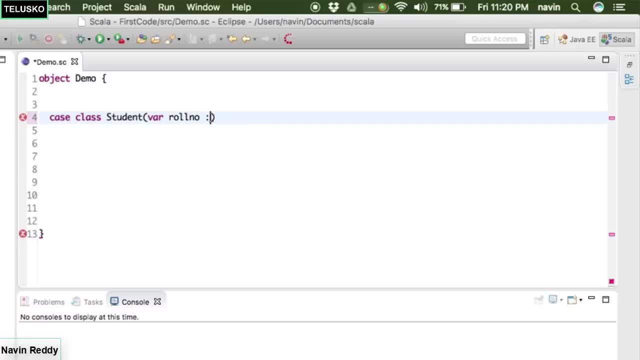 As var, I will say this is row number of type int. then I can say I have a var which is name of type string and I have a int. I mean I have a var which is marks and it is int. so you can, you can compare this thing with your Java code. so if you can compare your Java code, 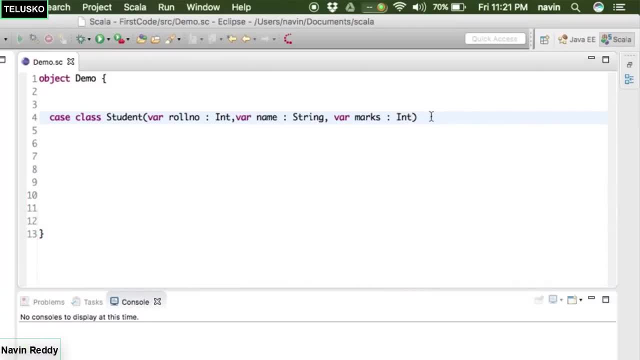 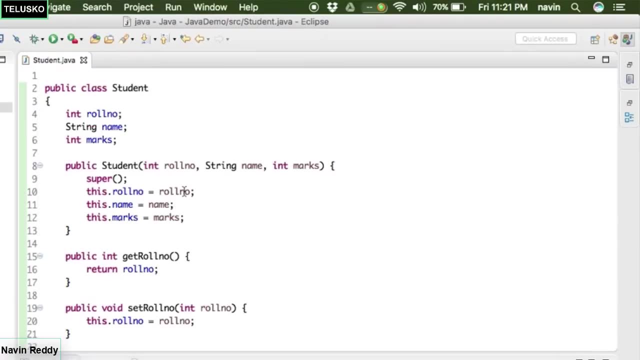 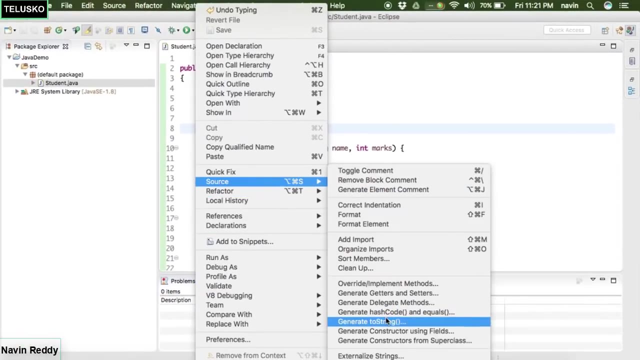 here. that's your Java code, right, so you can compare this with this one line. and you can also specify, So I can create a default value. so let's say in this constructor itself if we can create a default constructor here, so I can create a default constructor. I will say source and 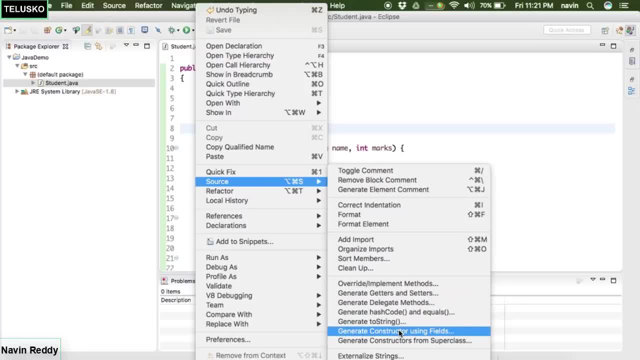 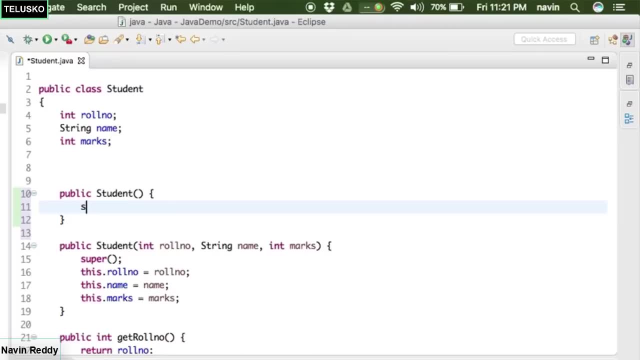 a default constructor, so a constructor with no fields, and okay, so I got a default constructor here and I can assign some values. right, I can say by default: if you, if a student is not specifying row number, row number will be one if it's not specifying the name, name. 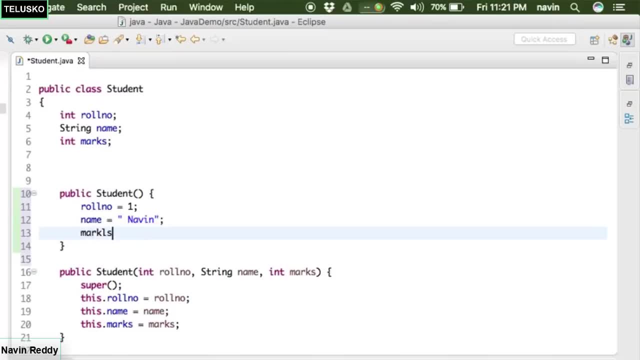 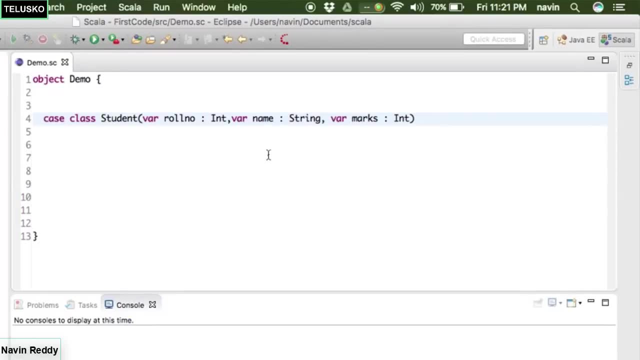 default, let's say navin, and it's not specifying the marks. marks by default will be, let's say, 90. that's default values. we can achieve the same thing in in student by specifying the values here itself. we can say the default value for row number, let's say this is one. 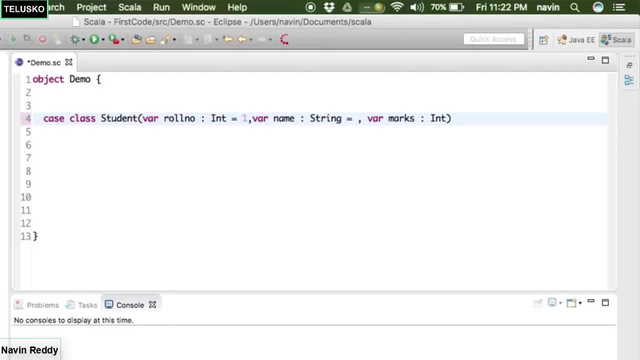 the default value for name is, let's say, navin, and the default value for marks, let's say this, is 90. So we can achieve the same stuff here in one line. You can see that it's that amazing. and if you want to provide some definition here, if 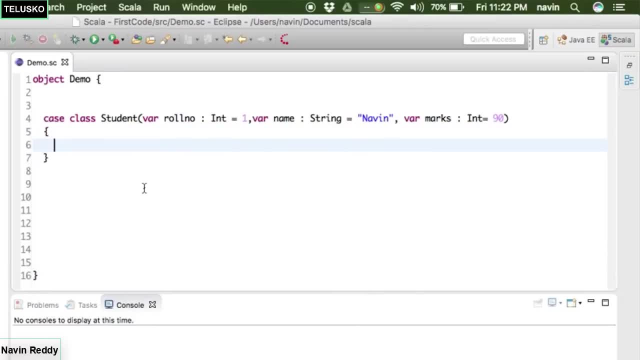 you want to provide some methods? we just have to open the brackets and you have to close the brackets. So, with this three lines of code, we have actually created a class with a constructor with which accepts multiple parameters. awesome, right. so now let's create an object of it. 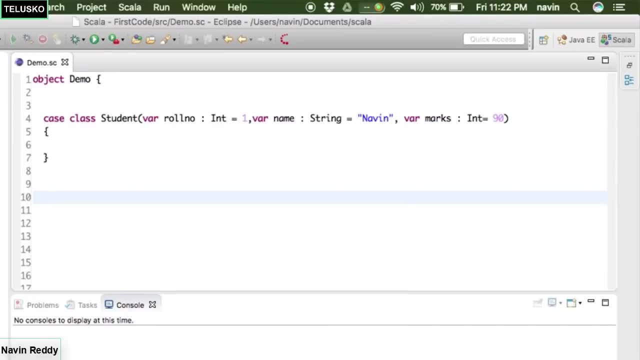 now, how do we create an object? it's very simple. we can simply say I want to create an object like: okay, hold on, how will you create an object here? So it's very simple. It's very simple. You have to say var will say s1, equal to student around bracket, and that's it. we got our first. 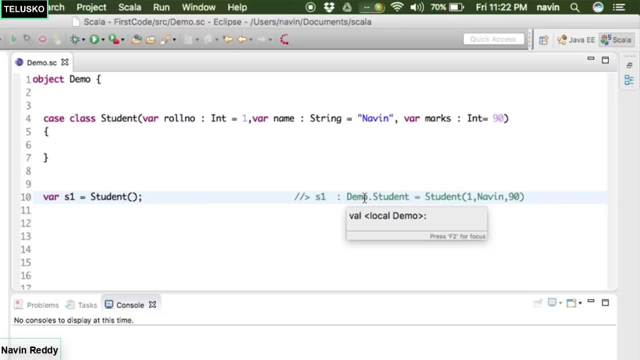 object here and you can see we got we also we are getting some instant output. we got one. we got a student object with the default values. even if you don't mention any value here, it will take the default values, but we can change it right. I can say I want the row. 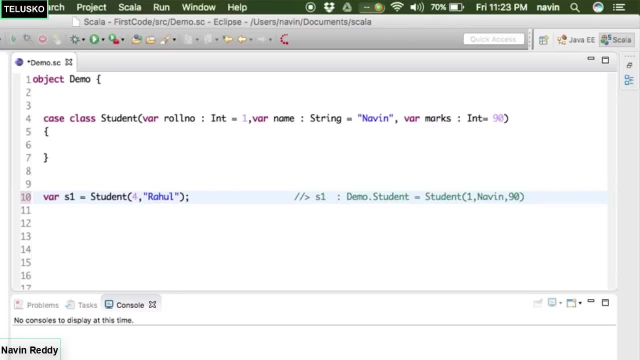 number as 4, I want the name as Rahul and I want the marks as 75. now, if I create the object, we got the object with those values. In fact, we can also specify only 4. if I specify only 4, it will take. it will take 4 as a value. 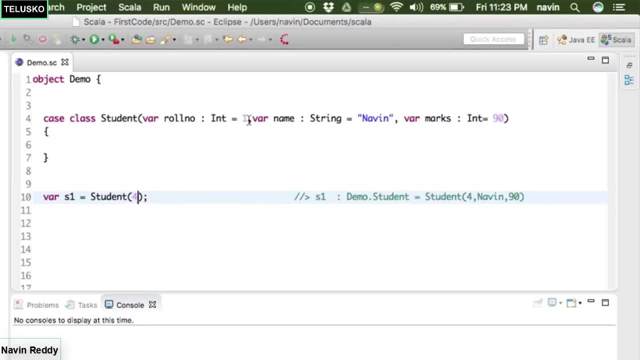 and the remaining part will be taken from the default value. so it was taking the row number as 4. that's the element. but this too is taking as I mean is it taking as default. so that also means that it we are also achieving constructor overloading here automatically. 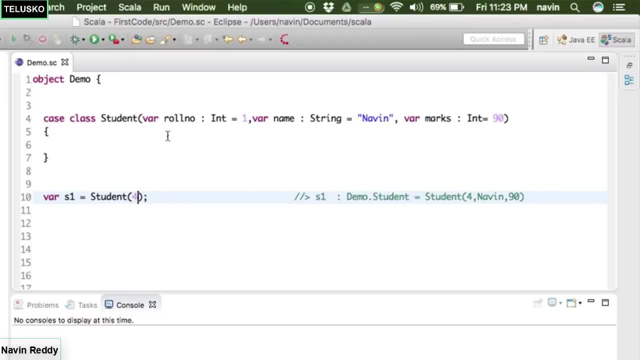 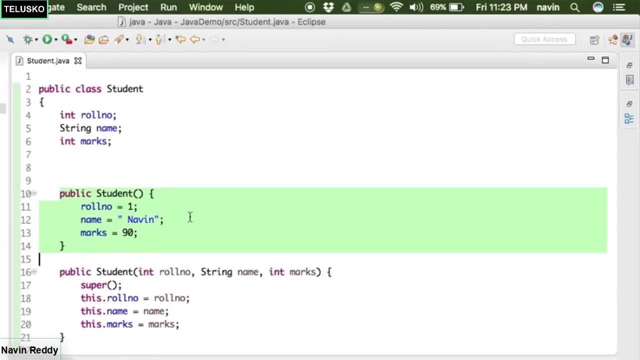 you don't have to do any stuff there. So we are achieving constructor overloading by default. it is that awesome, because in Java you have to create an object, You have to create multiple constructors. so this constructor which takes nothing, then this constructor which takes everything, then one more constructor which takes only one. 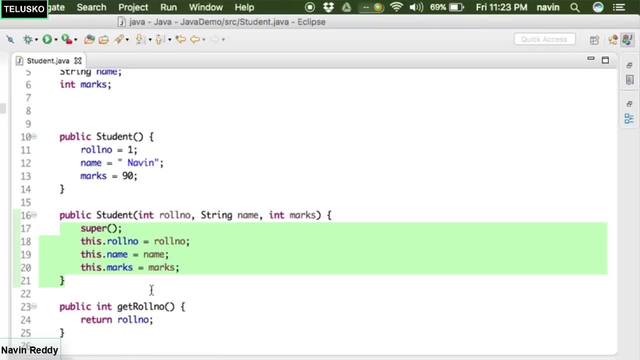 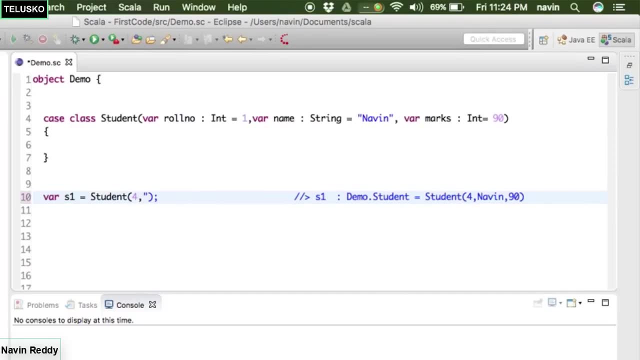 parameter. next constructor, which takes only one parameter, which is name one. next constructor, which takes only one parameter, marks. it is very hectic, right? so we can specify. we can pass two parameters here. I can say: this is, let's say, this is Rahul, so I am not specifying. 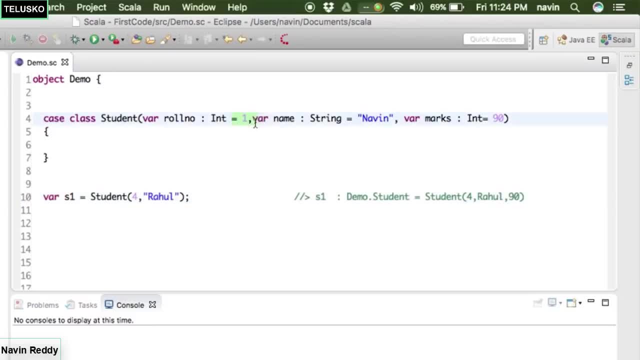 the third parameter. so I am specifying only 1, 2. so I am specifying this is 4. I am specifying this is Rahul, so this will be taken as default. But what happens if I pass only Rahul here? So it will get confused, right? because the 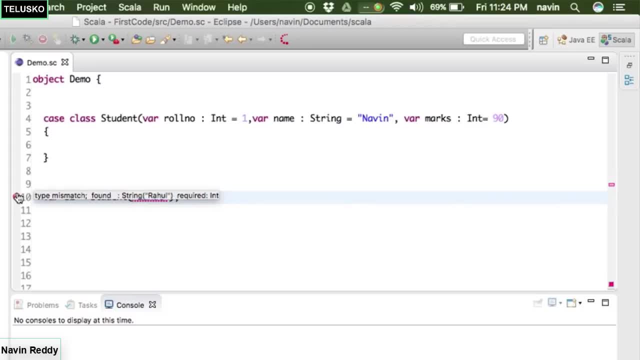 confusion is: how will you know that? which method- I mean which variable- you assign the value? So in case, if you are first, if you are passing, the variable is not matching with the first variable, it will give you error At that time. I specifically have to mention: 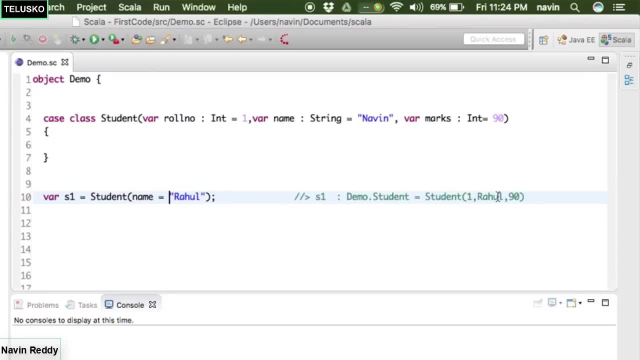 that we assign the name and you can see the name is changed, but remaining thing, which is row number and marks, is same. So that's how you create a class, you create a constructor and you create an object. But the thing which we do here, we have to write lots of stuff. 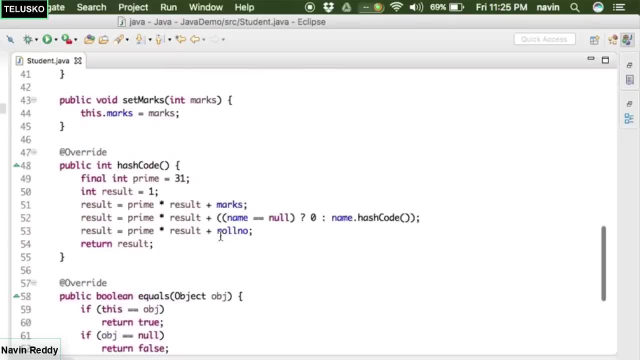 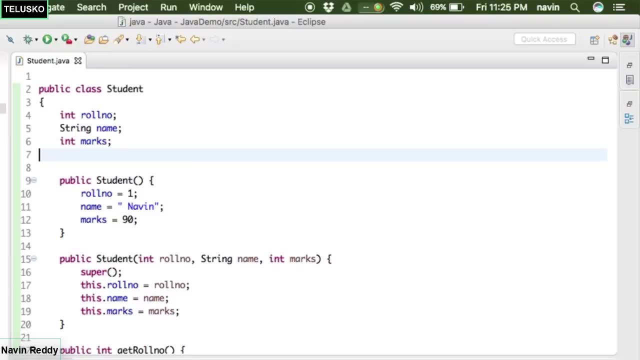 right, we have to write lots of lines of code. You can see that. So this is the difference between Java and Scala. So if you are from Java background, if you have, if you have done this, you know what I am talking about. right, In Scala, we can write in those things in two. 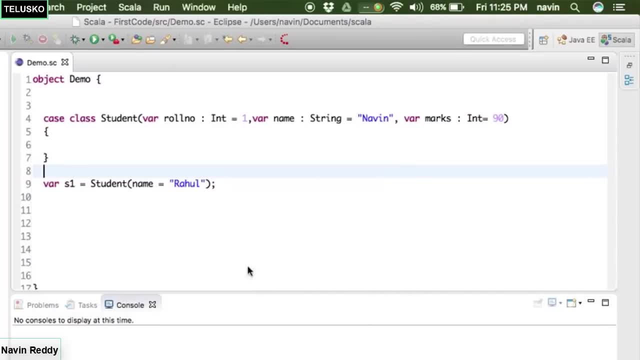 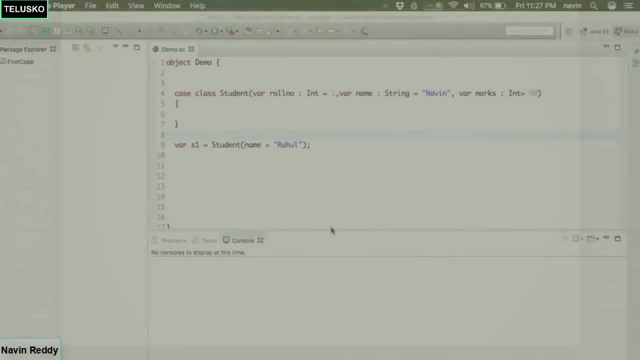 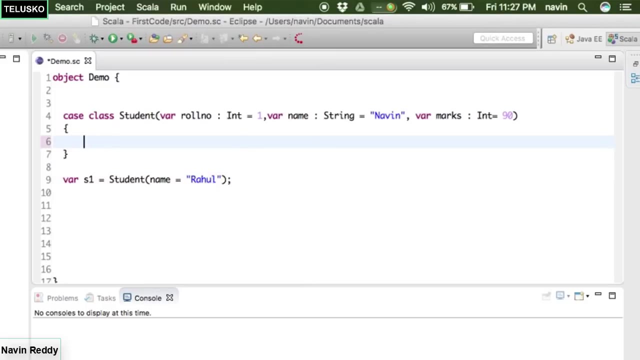 lines. Again, there is a learning curve here, but the only thing is it is worth learning, right. So now let's see how do we define method in Scala? So it's very simple now. So let's say: I want to define a method. I mean a function or a method in 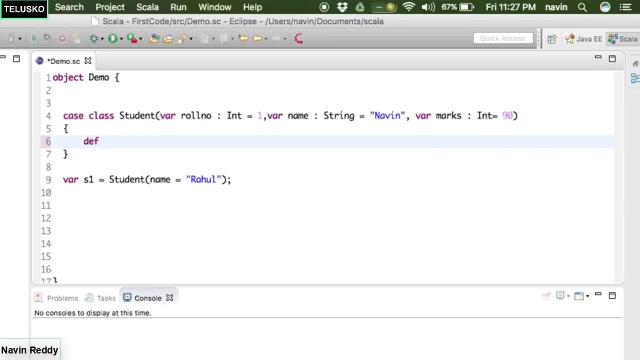 Scala name as show, So I can say def- that's the key word we use to define a function, and I can mention a function name as, let's say, show, And so we just have to say define function, show. And now we can- in fact we don't have- to provide- yeah, we can provide the brackets. 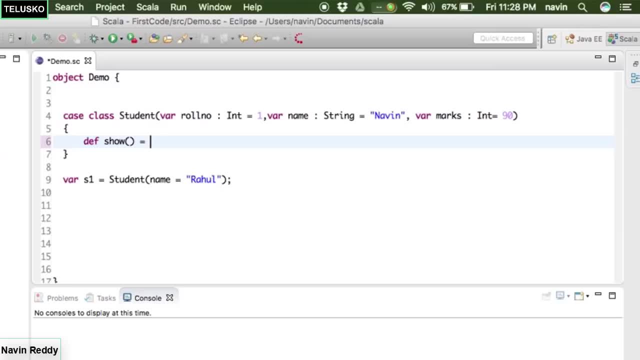 there and we have to mention the equal to sign and we can do whatever you want. We can say print ln, it will print. let's say hi, Okay, that's it. That's how you define a function. The only thing you have to remember is we use equal to operator when you define a function. 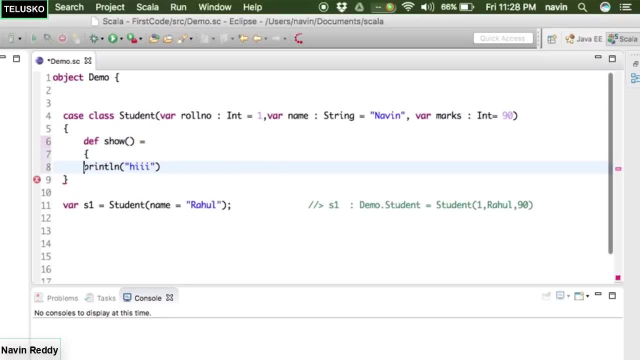 Again, if you have multiple lines of code, then we have to use that curly brackets, which we use in Java. So we have to. So is that? So we have to use curly brackets only when you have more than one line, But if you have only one line, you don't even need curly brackets. Okay, Now how do we call the? 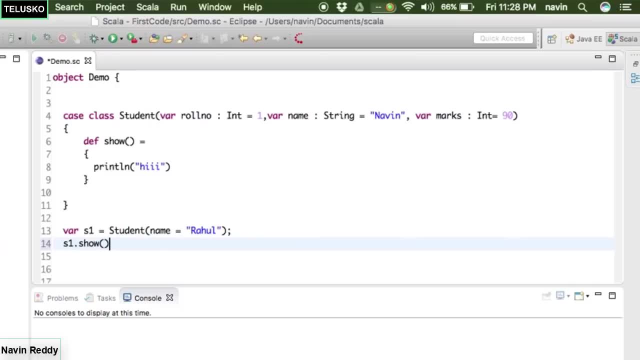 method we can. It's very simple, as we have done in the in Java itself. We can simply say show and you can see we should be getting the output here. We're taking lots of time. You know there's something, there's, there is some bug in the system. you know it takes lots. 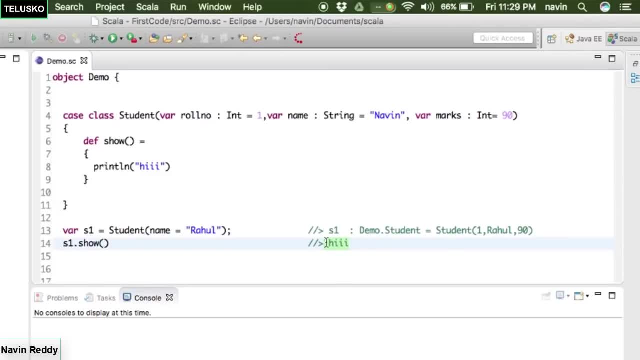 of time to iterate anywhere. So you can see. We got the output as hi. So we can define the function by using a def keyword and we can specify show. We have to use a equal to symbol and we can write all our statements here. Now, if you have only one statement, you don't have to even mention the curly brackets. 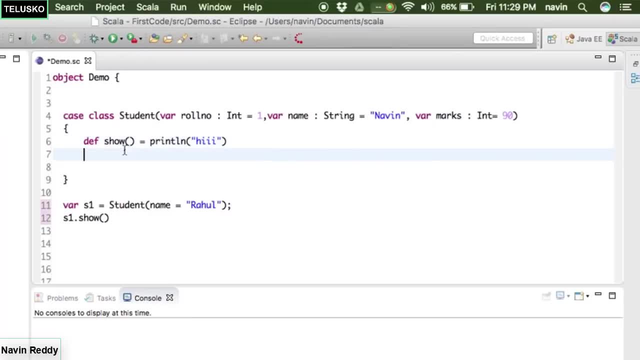 We can mention equal to print ln. and now, even even now, it will work. You can. if you can see, we got the output which is hi Right, So that's how we can define a function. Now, What, What, What else? 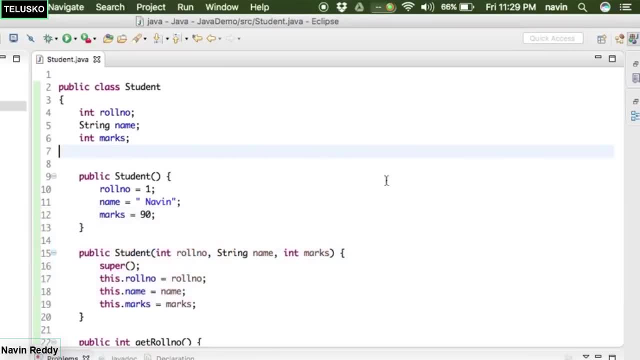 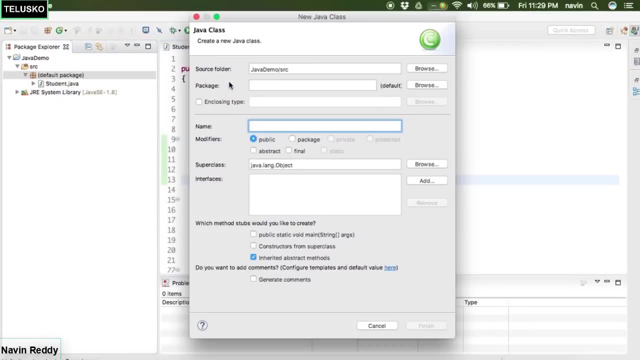 Now let's say: let's go back to Java, Let me see what what else we can do here. So let's say: I want to. I have a main main class here. I will say: this is a class- Let's name this as a demo class- which has a main function, And from this main function I want to create: 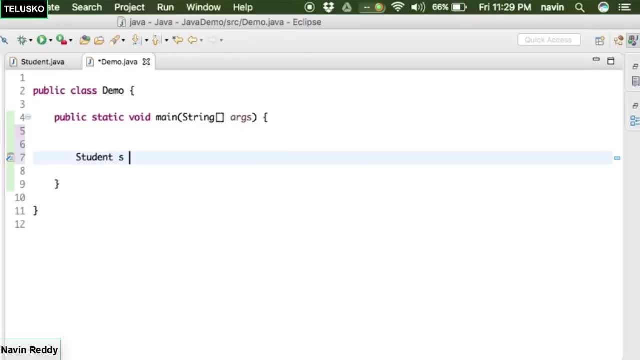 two student object. I will say student s1, equal to new student. I want to pass some values here. Okay, let me pass 1, Navigate- Okay. Okay, This is 20, comma. Let's see this is just 80. okay, that's 1.. Let me just copy this: and this is s2 and this is 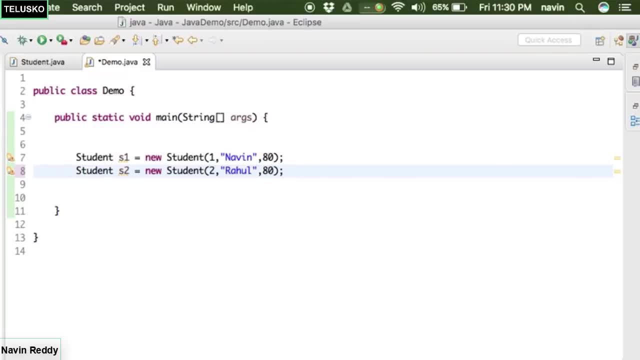 second, This is Rahul, and let's say this is 90. So what I want to do now is I want to perform an operation here, which is which will compare this two objects. So if I say, if I, if I try to print, If I try to print s2.. 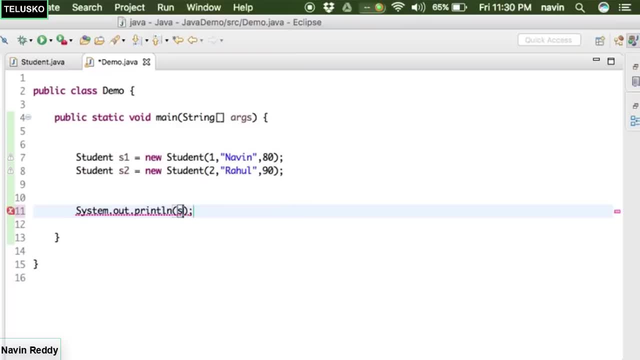 S1, if I try to print S1 dot greater, I mean is greater. that's how we do it right. So we can say: is greater and we can pass S2.. So now in normal, in Java, normally we use methods right. 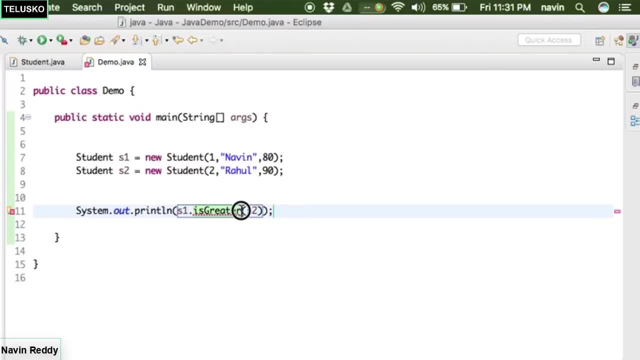 So if we want to compare two objects, we always use a function, I mean a method: like is greater. So if it is greater, then it will return true, otherwise it will return false. But unfortunately I don't have any method called as is greater. 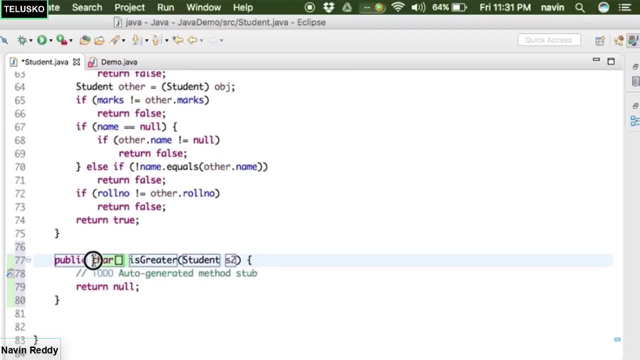 So I'm creating that method here inside my student class, which will have inside this method will return a Boolean value and will return. Now, how do we compare this two? We can simply say this row number, I mean this marks. how will you compare this greater? 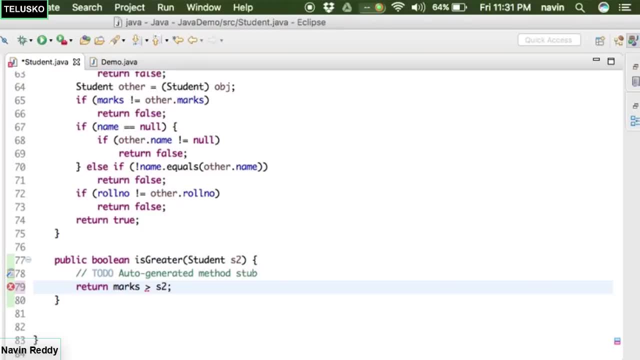 We'll simply use marks, So if this marks is greater than S2.. S2 dot marks, let's say I want to sort all the students based on their marks, So we can we use this, we can use this method which is greater. 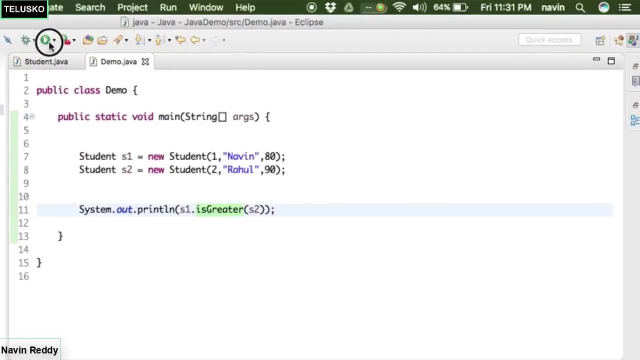 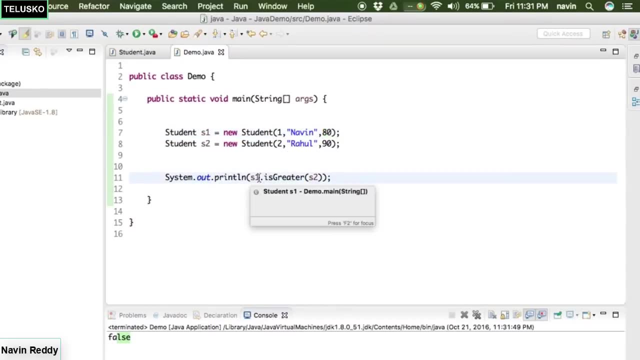 And if you can run this code- I mean not this one- if you run this code, you can see we are getting the output as false, because this is not greater right. And if I replace this, if I change this value to 99.. 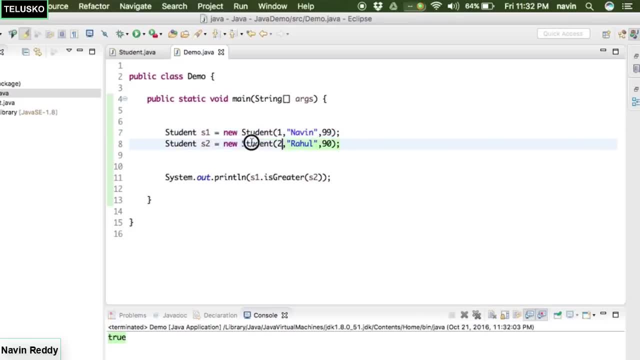 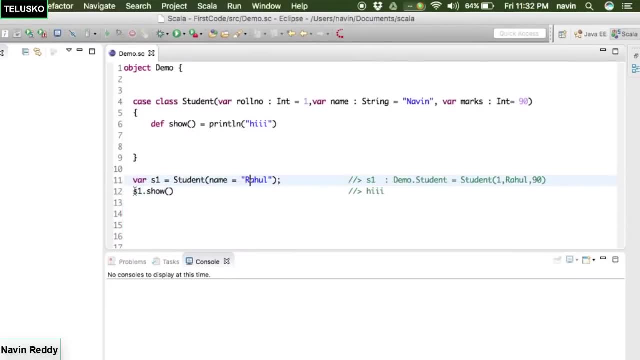 And if you run this you can see we got true. That means We can compare two objects with the help of a method. But how do we do that in Scala? So in Scala what we can do is Scala supports operator overloading. 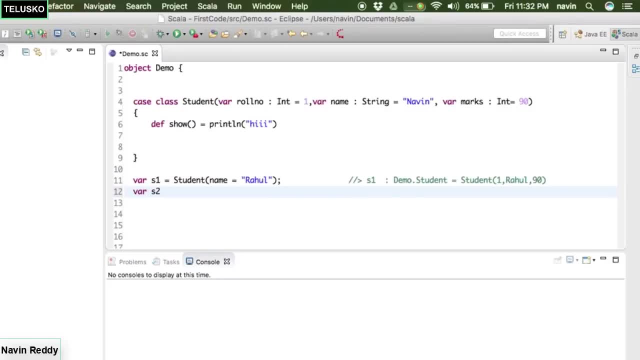 What it means is I can compare two objects. I can say this is S2 and this is student, And you can see the object- Rahul got the values, which is one Rahul. I mean I will remove this stuff. That means the object which we'll be getting is one Navin 90.. 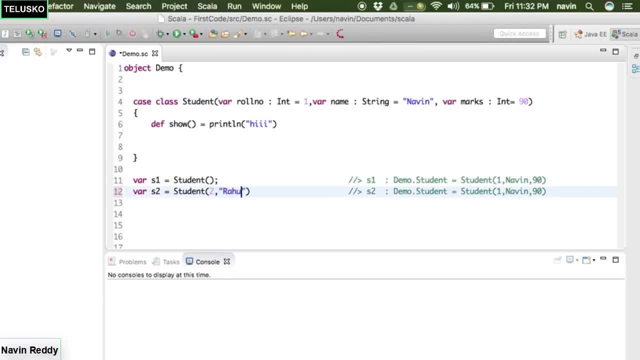 The second object. I will say two, Uh, Rahul, and let's say 80,, 88,, okay, And you can see, we got the. we got two objects: One is 90 and one is 88. And how do we compare here? 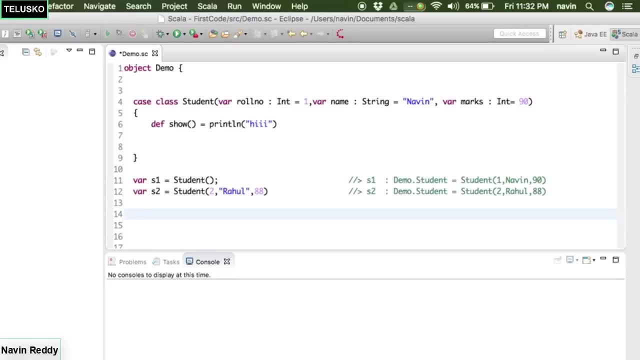 So we don't use. I mean, we can use methods, but we can also use something else. What are what? is that something else? I can say S1 greater than S2.. So we can actually use a greater than symbol here, but hold on. 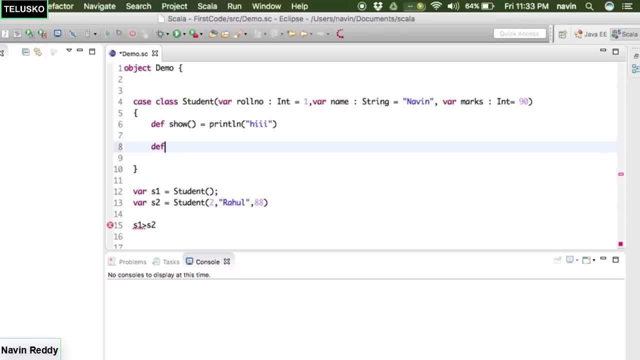 Before using that, we have to define that method here. So we can say def, we can define this function. I mean this, this method which is So function, which is greater than sign, and we can pass a parameter which is S2, because this is actually S1 dot. this is the function name and we are specifying the S2 as a parameter. 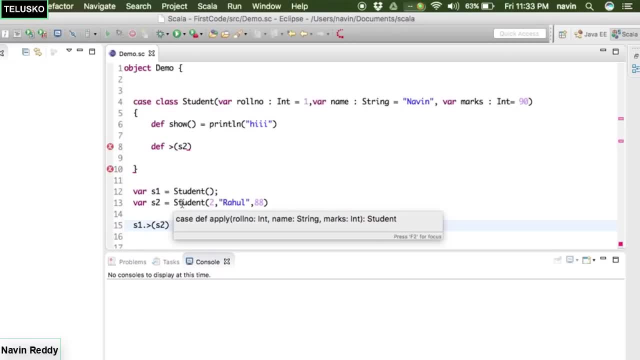 Again, we have done that earlier, right, With the help of a plus operator, And now we can define a function. It returns you a Boolean value, So I can say: this is Boolean. Now it is based on what? So it is returned. 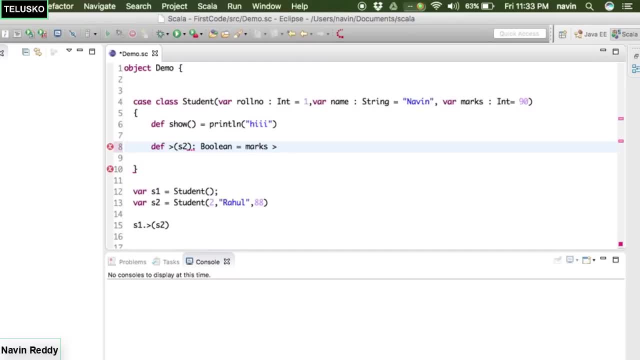 Mark Marks is greater than so marks is greater than what We'll compare S2 dot marks. That's it. Okay. There is something wrong here. It returned S2.. It's not working here. What's the issue? I missed something, I guess. 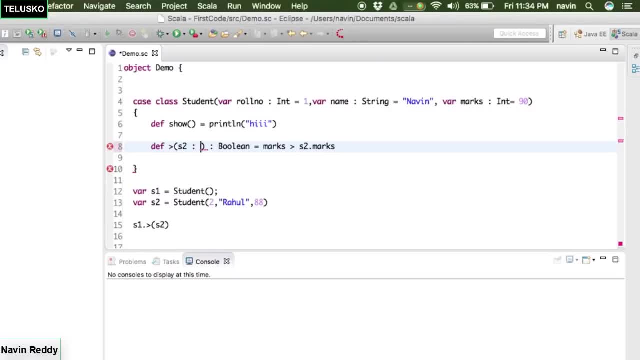 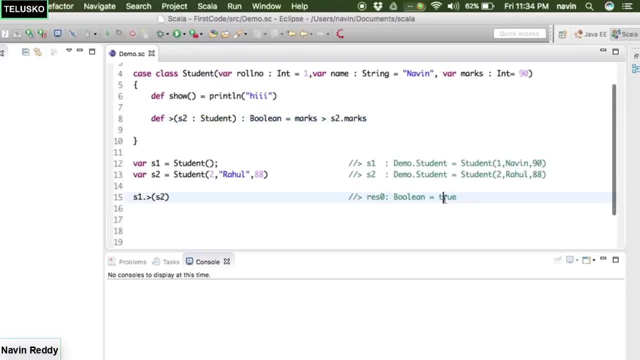 So we have, We have to mention the type of S2,, right? So S2 is of type student, My mistake? So when you define S2, we have to mention the type, right, And you can see we are getting the answer which is true, because S1 is greater than S2 because of their marks. 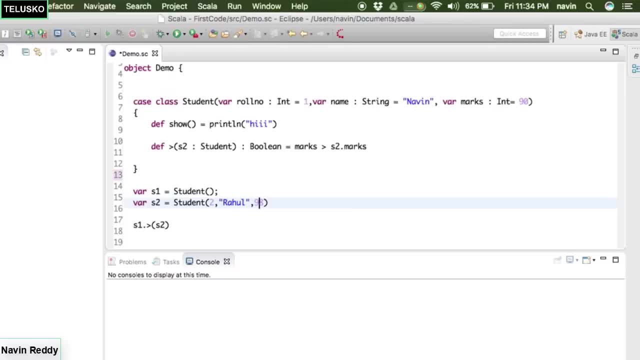 But if I change the value, if I change this to 98, and you can see, we got, we got false. Hold on, It is not yet Where is false. Come on, Come on, Come on, I want false as output there. 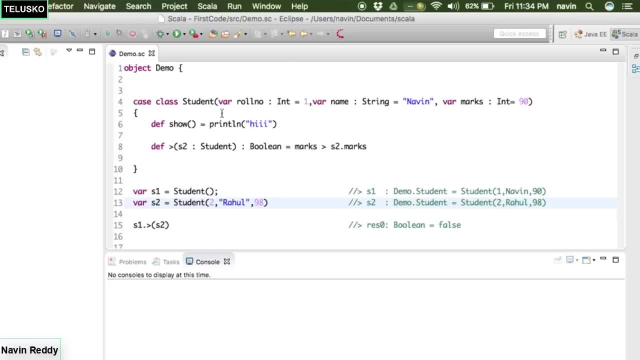 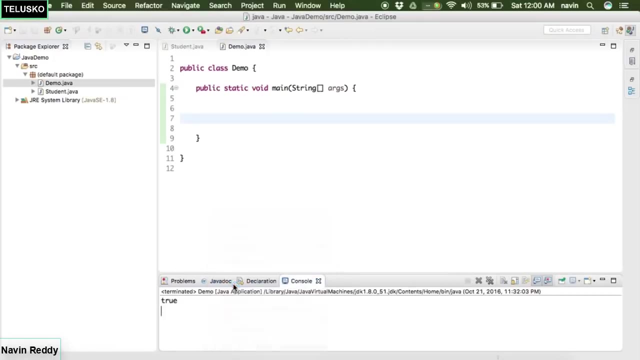 You can see we got false, So we can. So in In Scala we can. It supports fun, It supports functional, I mean function overloading. We can also use the operators as the function name. So once we have worked with objects and methods in Scala, let's see how do we use. 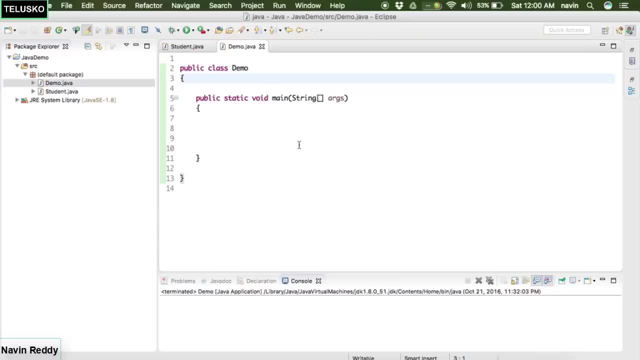 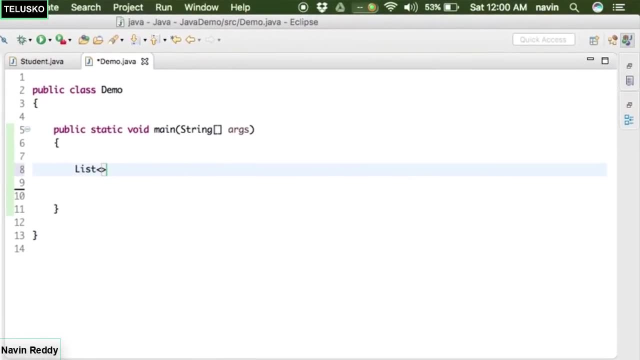 How do we use? What do you say List of values here? Okay, Now let's say, if you want to create a list in Java, So this is a Java console, here I'm creating a list, And normally to use a list we say list of integers. 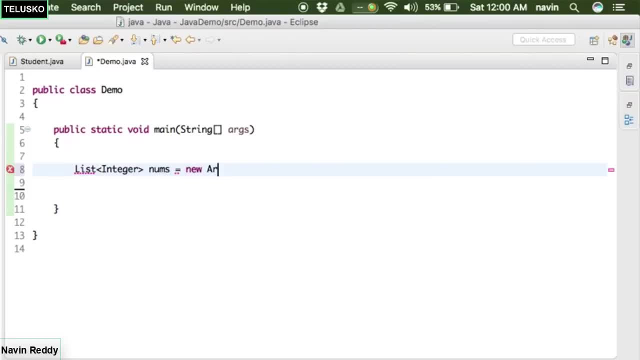 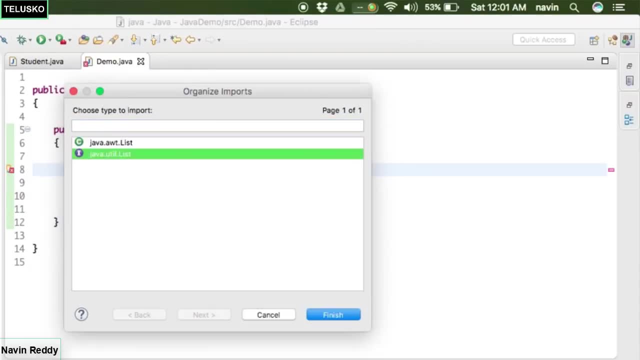 And we'll say this is nums, equal to. We say new, add a list, And then we can specify the values here. Right, So we can say let me put the package first, Which is util? Okay, So once we have got the package we can add the values by saying nums dot add. 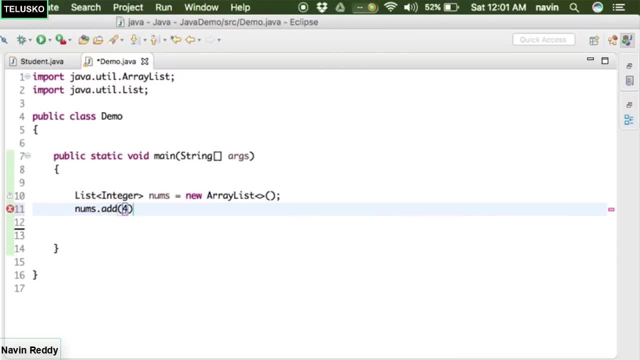 And we can say value four, And then we can add one more value below. We can say: this is, Let's say this is. We can say this is, Let's say eight. So we can do that Right. There is one way. 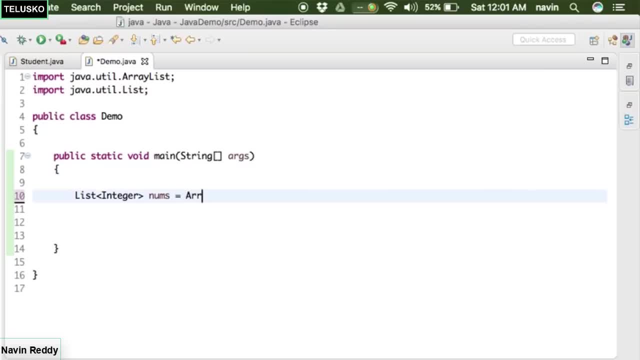 Another way is, if you already know the values, we can directly say: well, add this dot as list, Add this dot as list by passing some values. I can say: four comma, seven comma, two comma, three, Right, So we can pass the values like that. 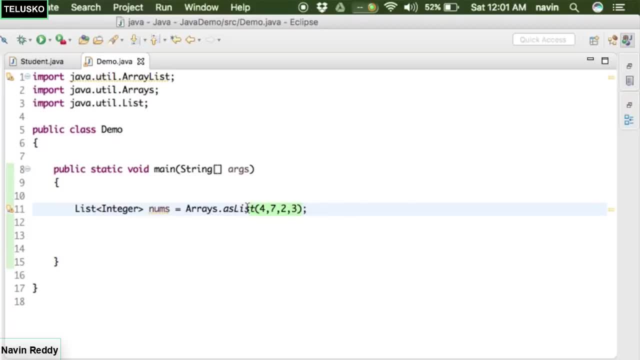 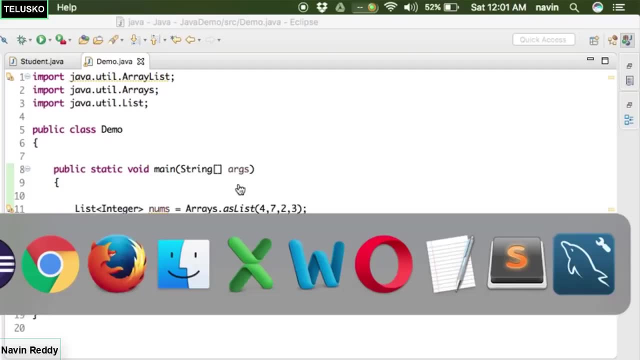 So we can use add this dot as list And we can mention the values here. Right, And how do we? So? this is how you do in Java Right Now, if we go to Scala, Let's see in Scala how we do it. 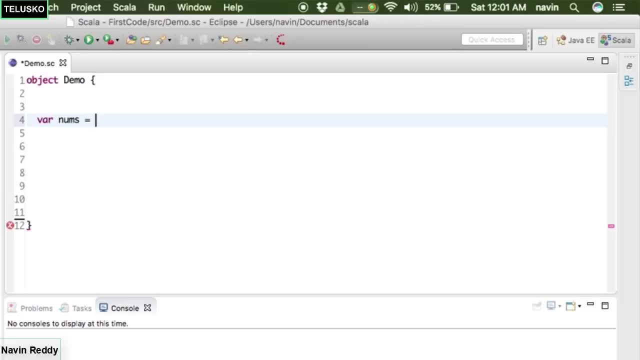 So in Scala we simply say var, nums equal to. We say list, We don't have to use any new keyword. We can simply say list And we can specify four, seven, two and three. So the thing we can do there is same as here. 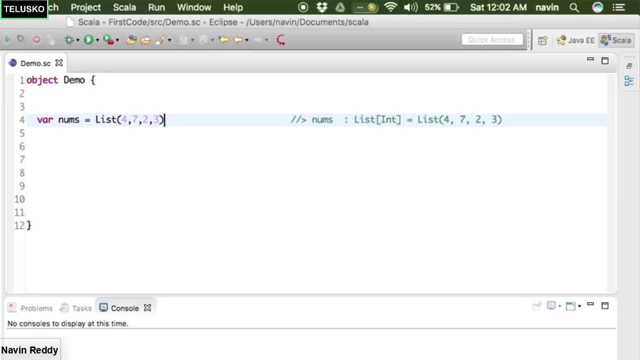 So we can write this stuff here. We can say list of values. So it is. You can see this nums. This nums is, by default, a list of int. Okay, So that's how we create a list here. Now, how do we print a list of elements in this Java? 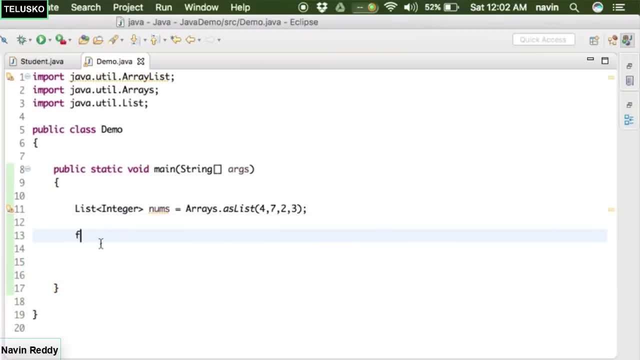 So to print a list of elements we can use a normal for loop or we can use enhanced for loop, Right? So normally in enhanced for loop we use int i, colon nums, And then we can print individual values. Right, So we can print i. 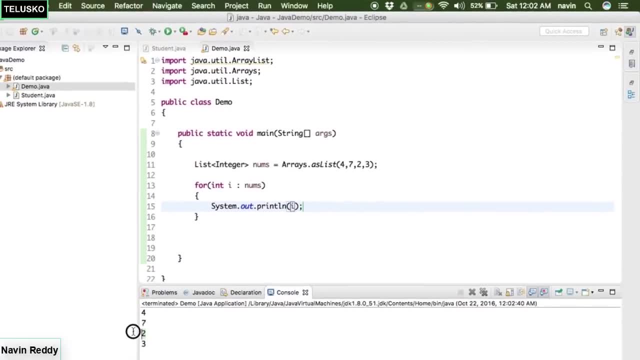 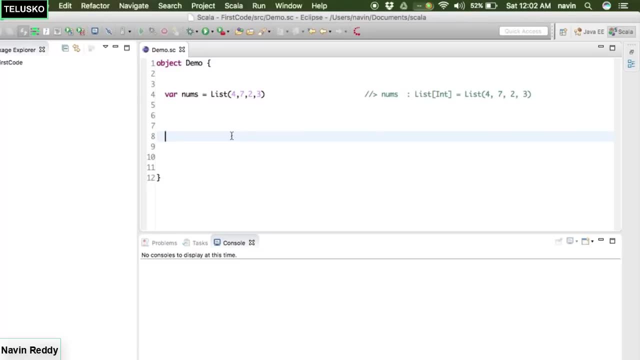 And if I run this code, we get- we got- all the values In Scala also. what we can do is we can use a list of elements, Right, We can use a enhanced for loop here. That is very simple to use: enhanced for loop here. 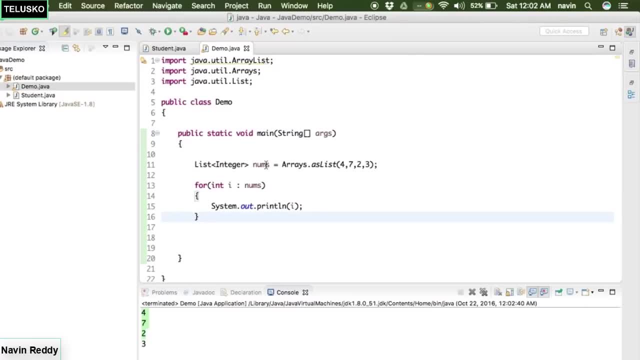 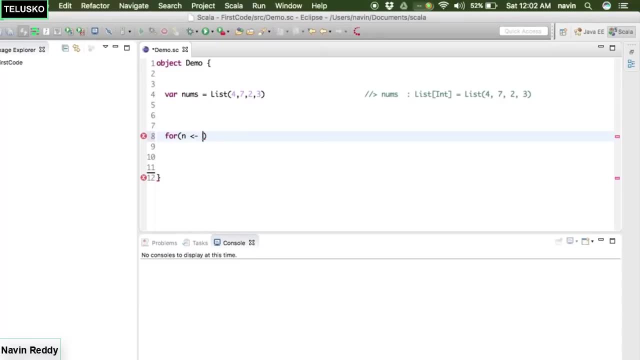 We can say a for And, but in Java we specify a colon Right. Here we don't have to specify a colon. We can use a arrow on the left hand side And we can say: this is nums And we can put a curly brackets here. 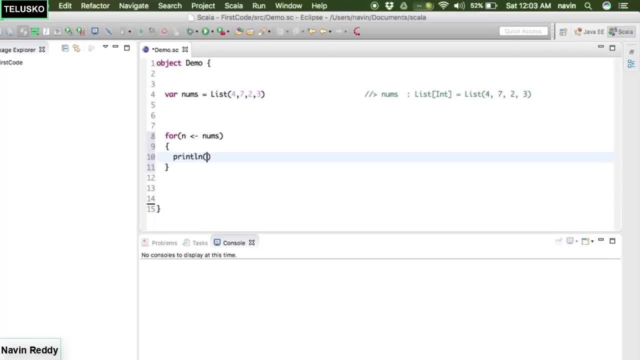 And instead of saying system, dot, dot, println, we only use println here And let's print n And you can see we'll be getting the output here. We can see we got the output as four, seven, two and three. In fact, we don't require this curly brackets when you have only one statement. 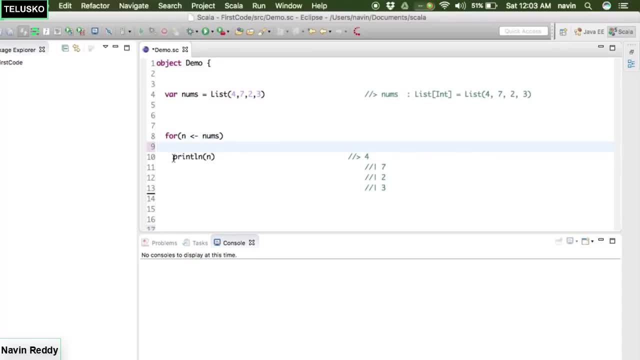 That will be because Scala believes in less number of lines, Right? So why to waste your number of lines just because of semicolon? So I can write that in one line And you can see we got the output as four, seven, two and three. 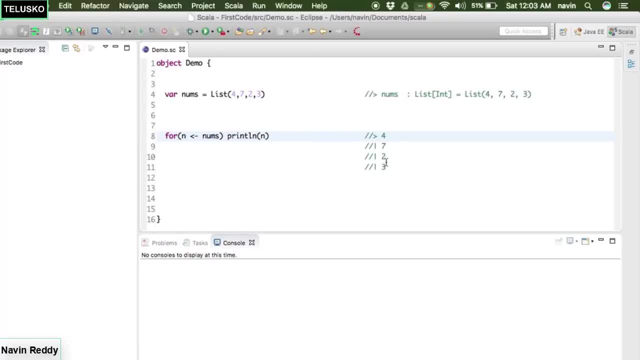 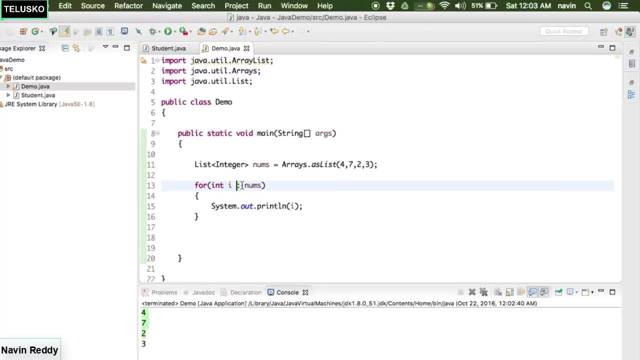 So that's how you use. that's how you use enhanced for loop in Scala. We use- we use a left arrow here. Okay, So in in Java we use colon, Here we use a left arrow. Now, I don't know if you are familiar with lambda expression in in Java. 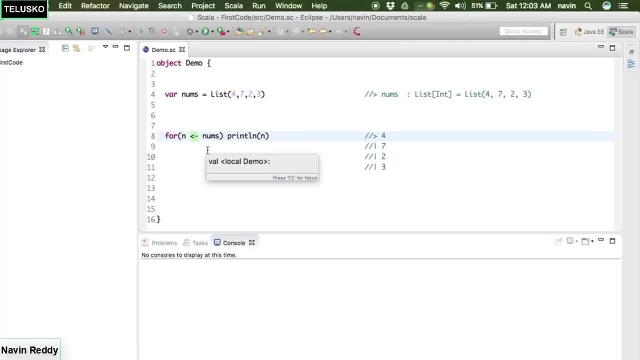 We can also use lambda expression here. So let me just do it in in Scala, in Java first, And then I will. I will show you how to do the same thing in Scala. So let's go back to. let's go back to my Eclipse in Java. 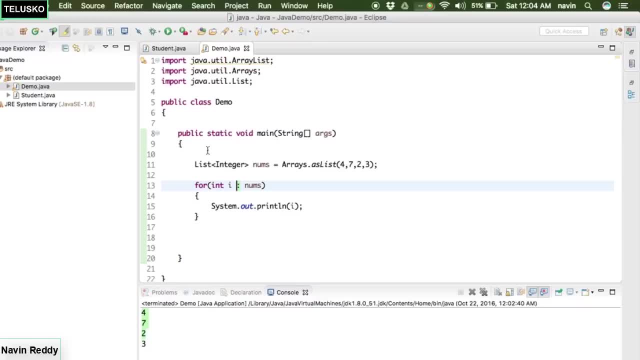 Now, how do we use? how do we use a lambda expression here? It is very simple. Now to know more about lambda expression, You can just go to. if you don't know lambda expression, That's okay, You can just go to the description in description. 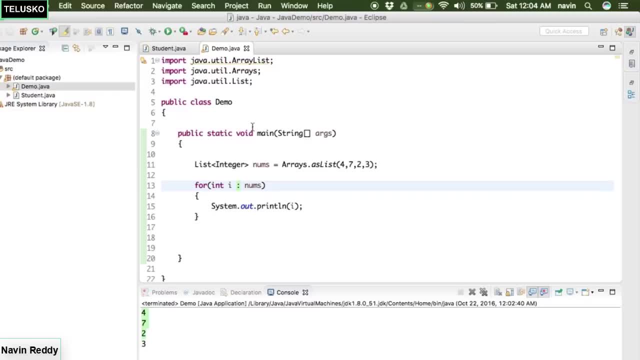 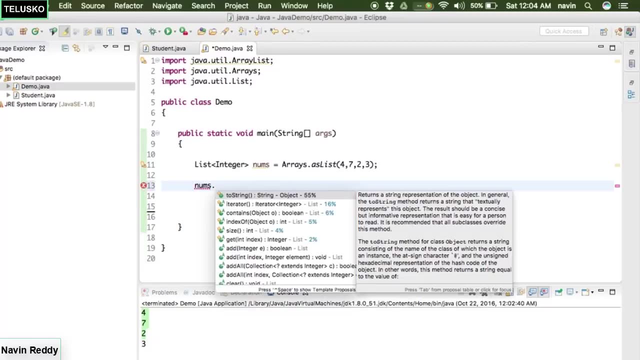 I have a link for the how to use lambda expression for, for, for list of values, So I will just remove this part. So in Java eight specially, we can use num start for each. Now, this: this only works in Java eight. Okay, It will not work in Java seven. 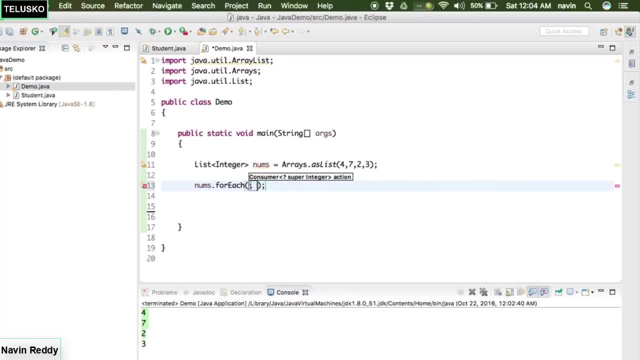 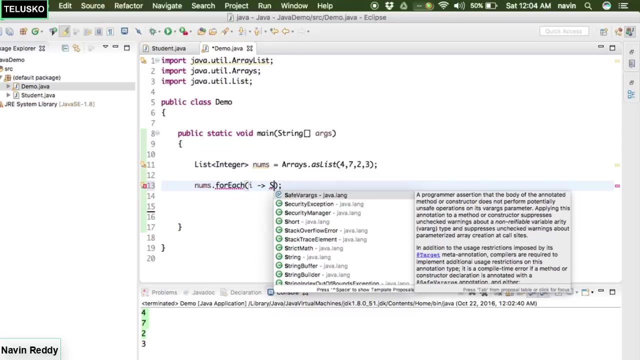 So I can use for each and I can specify I and we can use an arrow which is system, System. Oh, That's weird. So I and arrow And I can. I can specify system, dot out dot. Why the shortcut is not working here. 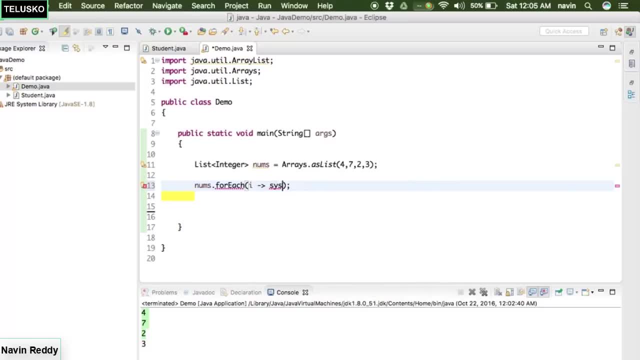 Okay, That's weird. System dot out dot. Okay, I think I should type it here. It's a system Dot out Dot, Print Ellen, And I can specify the value either. So even this thing works in Java. So if I run this code, you can see. we got the output. 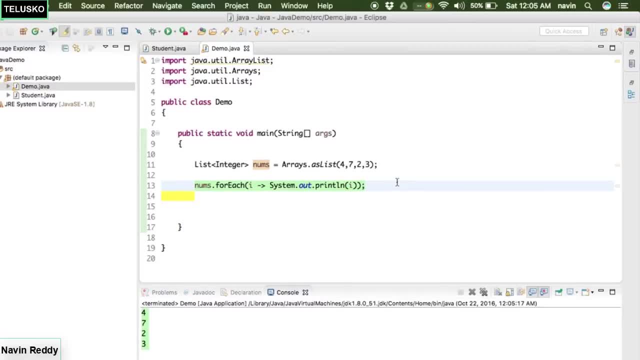 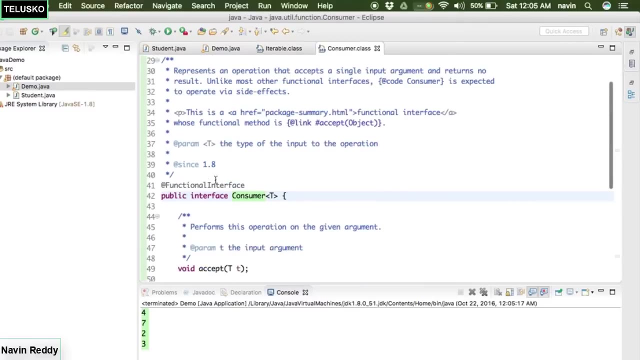 Now how exactly is working? You can just go to the comment section, I mean, you can go to description area and you can see that. But just to give you a glimpse, what happens is in Java, eight nums has a method which is for each, and for each takes the object of consumer and consumer is a interface. 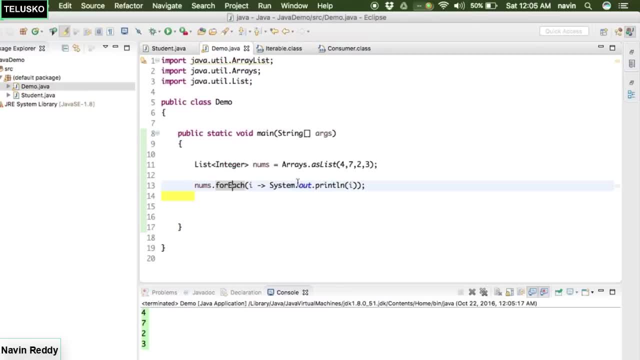 Okay, So what we can do is here in the code we can specify that we are passing the object of consumer. In fact, I think you should. you should watch the video, the description, you will get the complete idea and show wasting time here. So it is assumed that you can use lambda expression here. 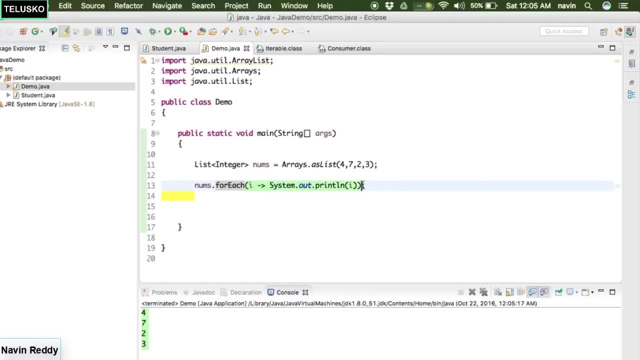 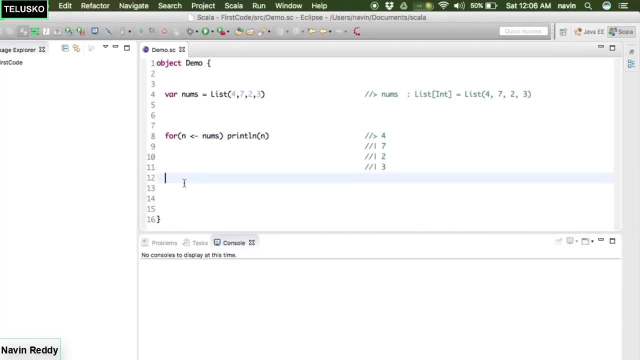 So in Java eight you can use lambda expression in. in Scala Also we can use lambda expression. So again, the lambda, the concept of lambda expression, came to, it came to, it came to Scala and it came to Java eight from Scala itself. So if you want to do the same thing in Scala we can use nums dot. again the method name. 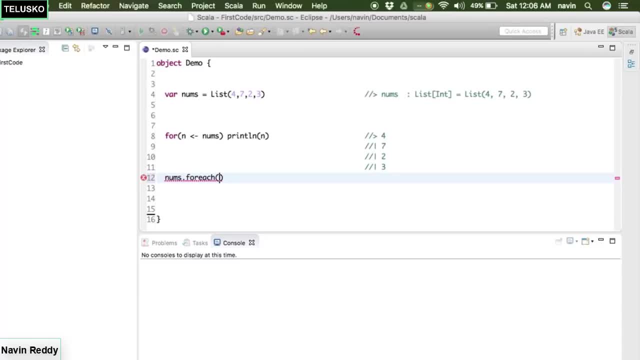 is for each itself, and we can use I as we have used in the, in the, in the, in Java. But we can specify the type of I here we can say int and then, instead of using so in Java we have used a single arrow right. 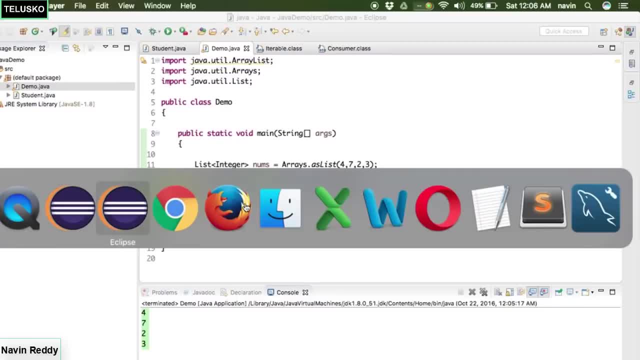 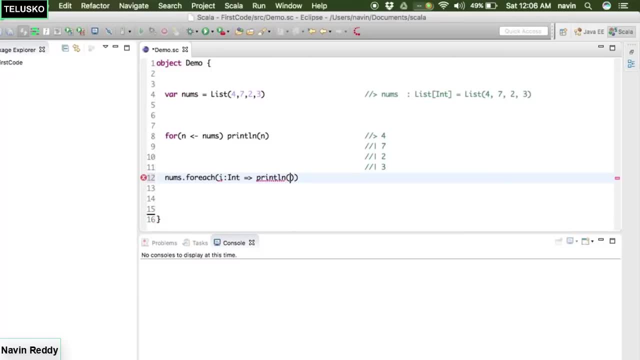 We have used a single arrow in in Scala we have to use double arrow. So we have to use a double arrow here And we can specify arrow. So I want to do print ln of I. That's it, So you can see we are getting an error here. 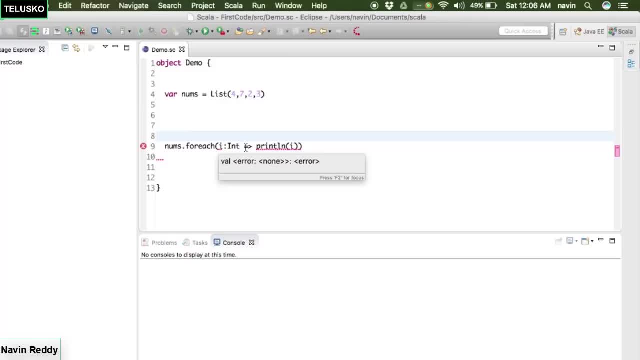 Why I'm getting error. That is weird. Oh, we have, instead of using- okay, I've used a wrong brackets, We have to use a curly brackets here. Yeah, so we have to use a curly brackets, not wrong, not wrong brackets. So you can see, we got the output. 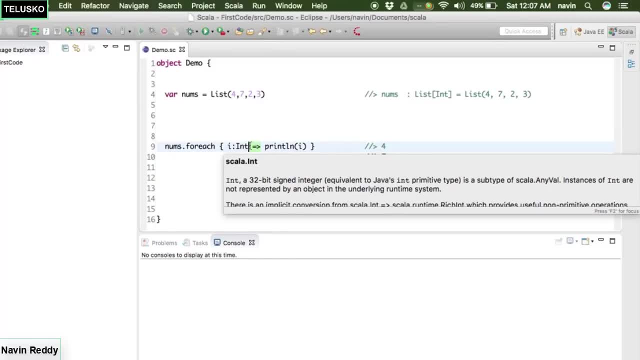 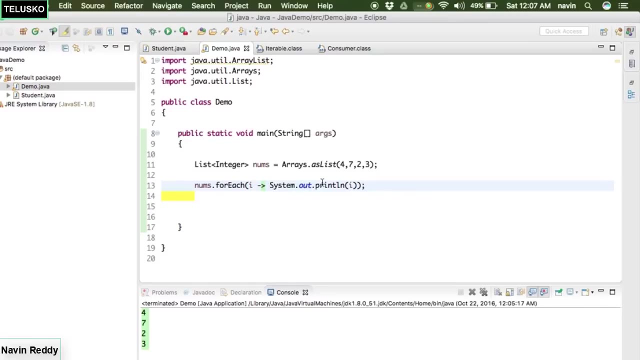 So we use lambda expression in Scala also, So I will. I would recommend you to Learn about lambda expression mode in Java 8 first, before jumping to Scala. So in Scala we use equal to and greater than sign. In Java we use a arrow, and I mean a hyphen and a greater than sign. 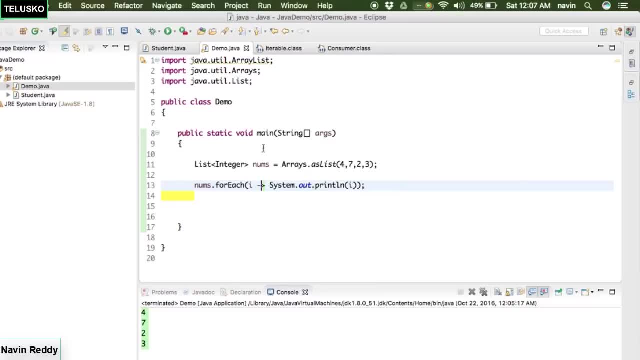 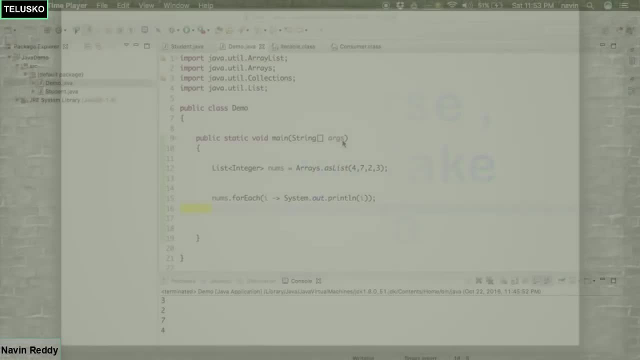 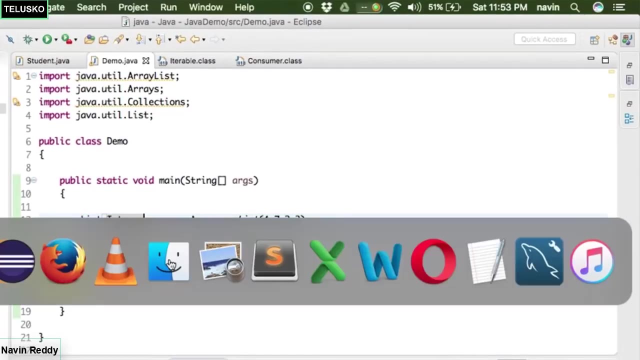 So that's how we use a list of values with lambda expression in Scala and Java. In the last video we have talked about list, right? So we have created a list of elements. So this is what we have done in Java code, And then the equivalent part is here. 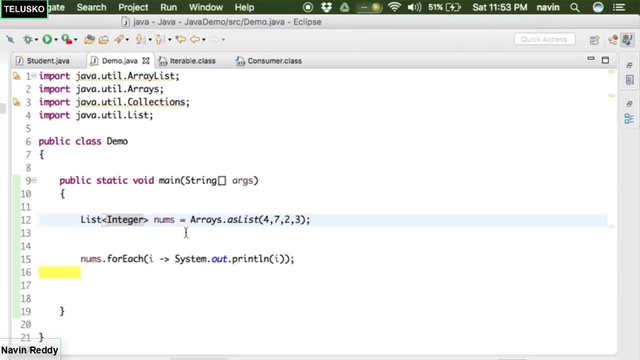 So this is what we have done in Scala. So we have used something called as lambda expression, right, So we can print the elements using lambda expression. Also, the only thing you have to remember is in Java, we use for each as a method, I mean a function. 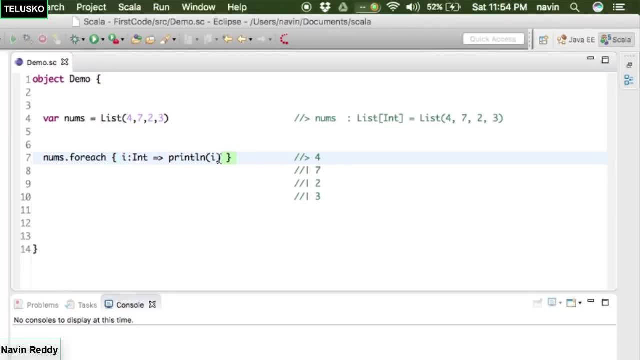 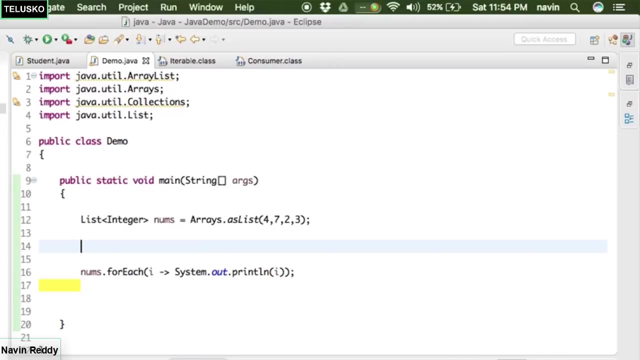 Here it is also a function, but we use a curly brackets to define a function here. So what I will do now is let's talk more about List here. just two more, I mean two more- examples here on list. So what normally happens is: you know, let's say I want to reverse all these elements. 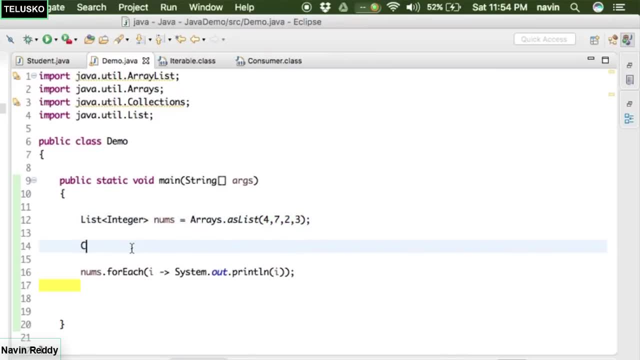 So now the way you can reverse all these elements is by: So in Java we have collections dot sort right, So we say collections dot sort nums. So when you say not sort but reverse, So let's say I want to say reverse, So we simply say collections dot reverse. 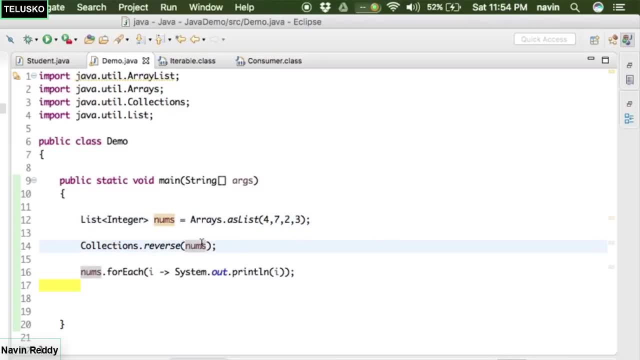 And we pass the nums here. So as soon as I pass nums and if I run this code, You can see we got the output in a reverse format. So we got three, two, seven, four. So that's the reverse order, right? So it is changing the actual values. 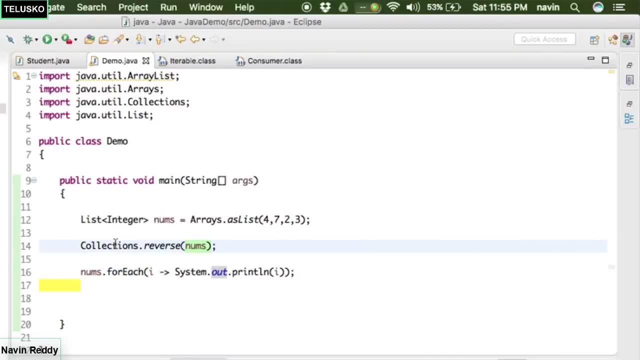 I mean when you say reverse, That means this collection is actually changing the values of the list. What it means is This nums is actually, I mean, initial value was four, seven, two, three. Later, when you say reverse, It is changing the values. 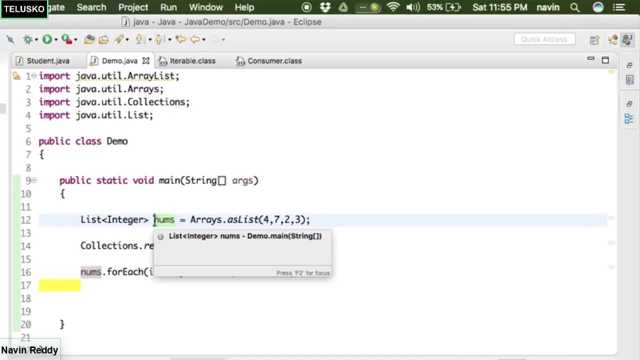 Of list itself. That means we are going for mutation. Now it is good, right, I mean we are changing the value. But the problem is If you have multiple threads working on the same list of elements. So let's say you have four threads. 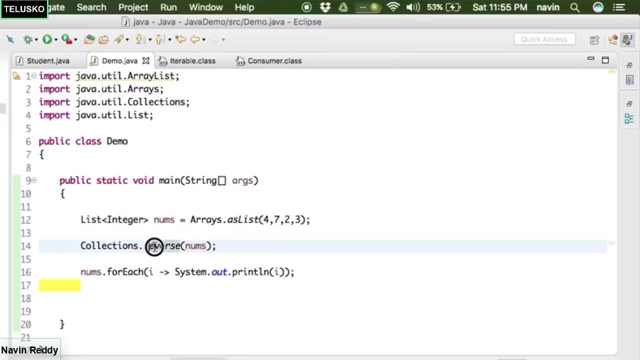 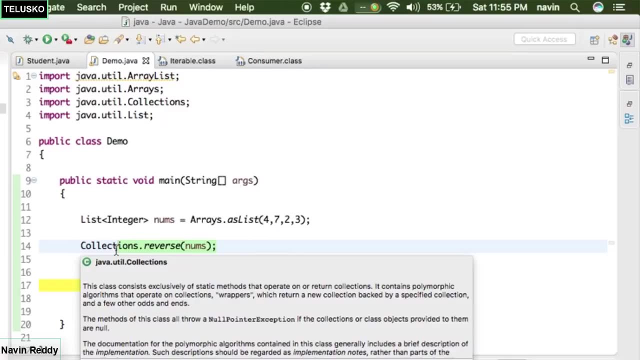 Working on the same list of elements And due to this, Due to this reverse, One thread is changing all the values, which is affecting The other threads, Right. So mutation is very bad thing when it comes to concurrency or using multiple threads. 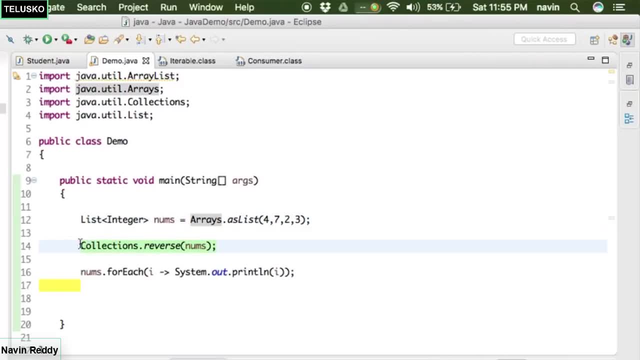 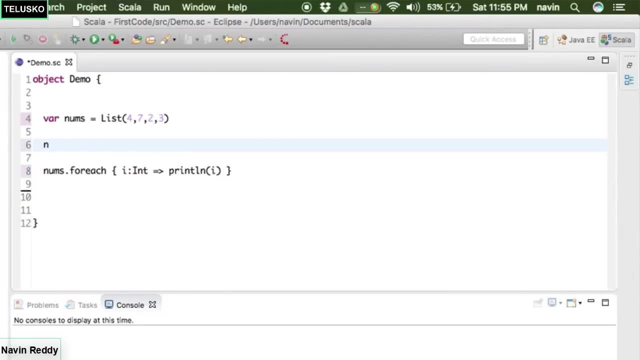 So I mean this feature is very good, It is very good, But the problem comes when you have multiple threads working with it. So in Scala what we do is We can also use reverse. here We can say: if I run this code without reversing it, 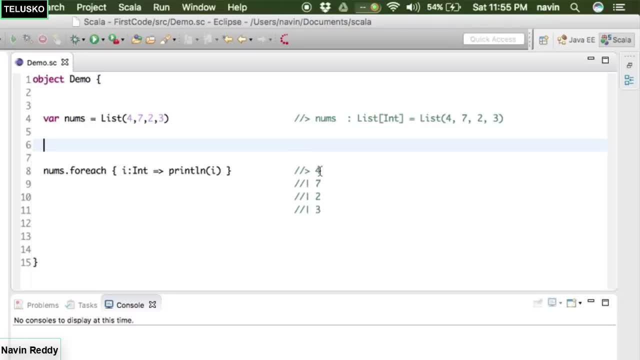 You can see everything. We are getting everything in proper sequence. We are getting. Okay, Let me just write, Let me remove that Println, Let me just give a space So that you can see in the one. You can see everything in one line. 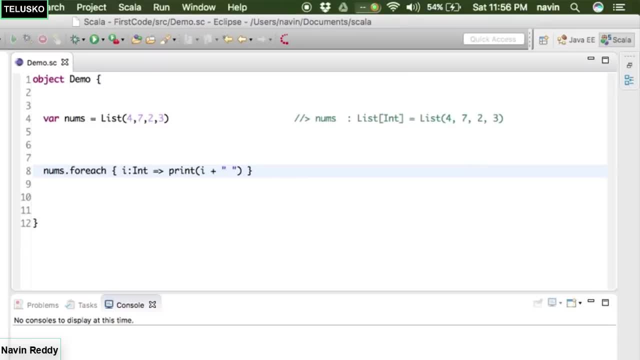 Is it not working? Okay, I think it is not working. Let me go for println itself: Okay, So you can see we are getting everything in proper format. Right. But let us say, If I: Okay, Is it println works or the space is not working? 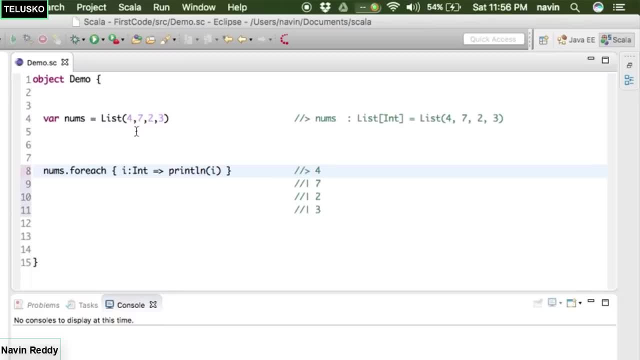 Let us go for println. So println, print everything in proper format, Right? What if I say reverse, If I say numsreverse? Okay, So if I say numsreverse, And numsreverse here returns the object of least, So it is not a void method. 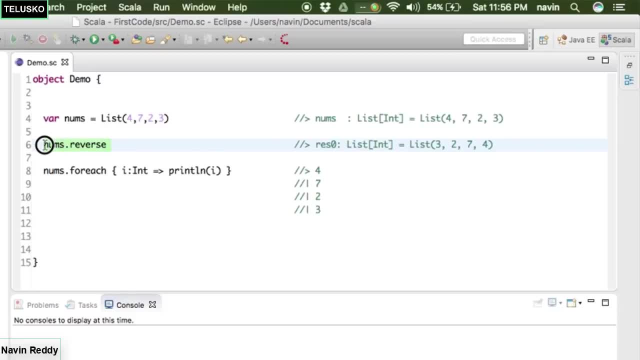 It is a third which returns a least, And that is why, if you only run this code, See the output, You are getting the output as 3274.. But after that, if I am running a for loop, You are getting the actual values. 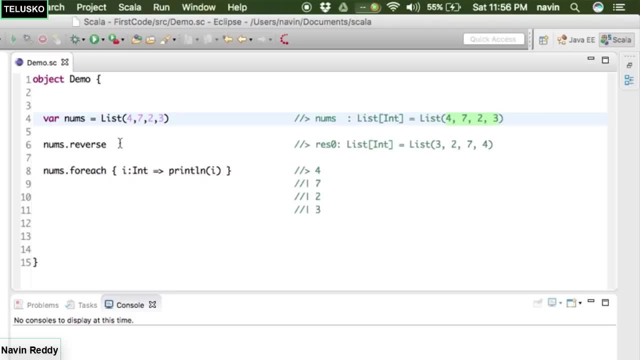 The original values, which is 4723.. That means when you say numsreverse, It is not changing the existing values of nums. That means we are not changing the existing value of least. We are creating a new least here. So what is happening behind this saying is: 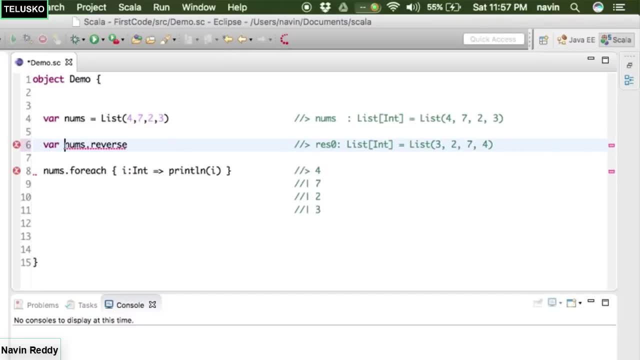 It is creating a new least for you. So if I say reverse nums, This is what it is doing. It is creating a new least of elements here. Okay, So we are not changing the existing values, It is creating a new list. 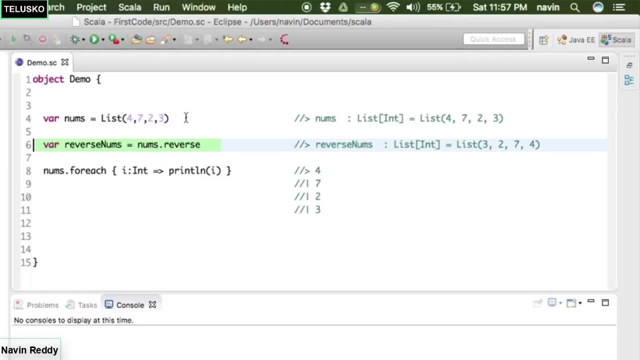 So, even if you are working with multiple threads, That is okay, because we are not changing the original list And that is why Scala is so powerful. We do not change the existing value. Okay, That is one of the advantages of using Scala over Java. 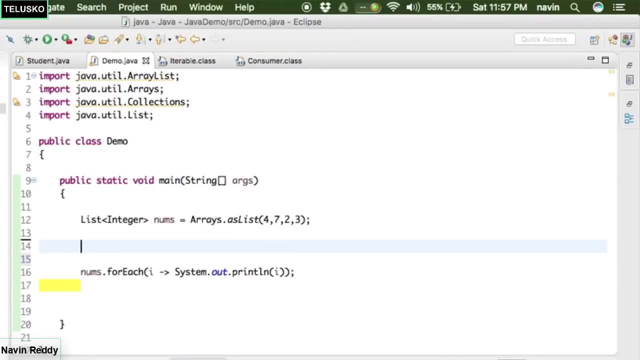 Okay, Let me remove this now. reverse: Now, what next? So let us say I have this four elements here And I want to remove top two elements. So what we normally do is We say nums. We have a method which is remove. 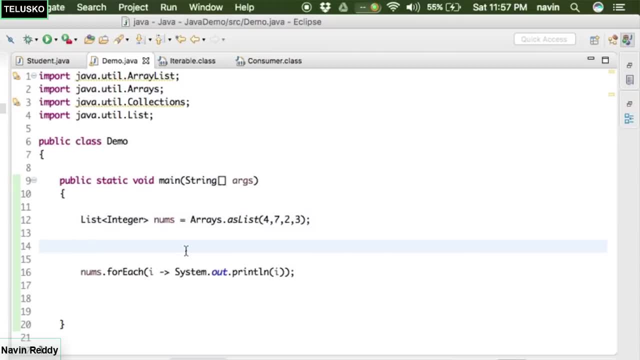 In which you have to mention the index. I can say one, I can say zero. It will remove the first element. And if I run this code, You can see it will remove. We are getting exception here. Is it because This one? 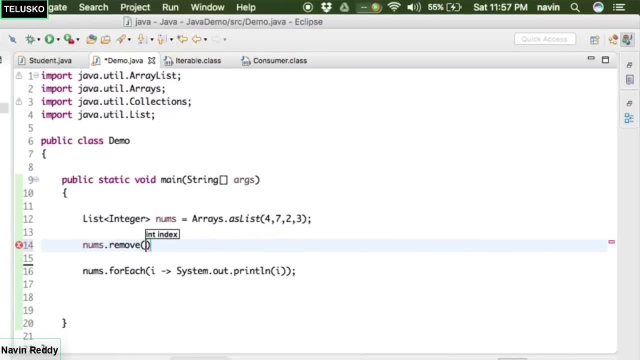 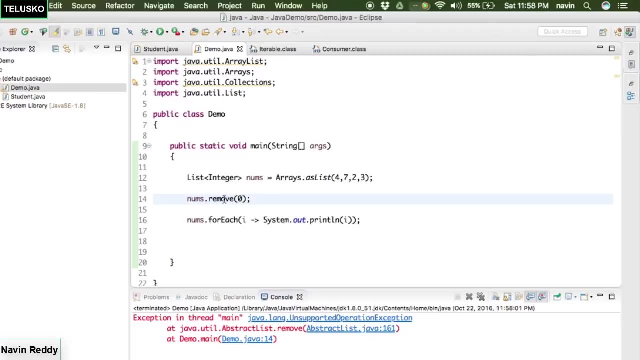 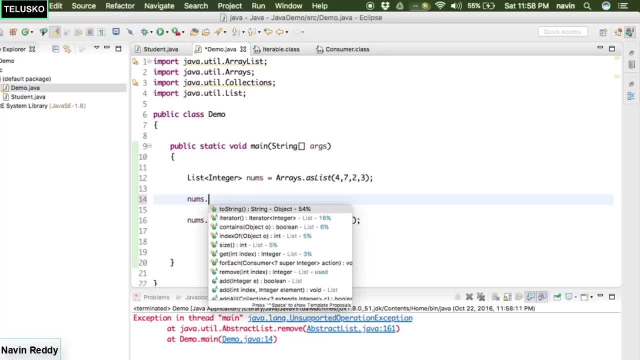 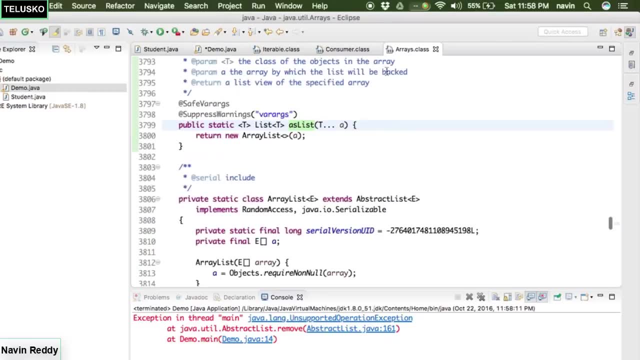 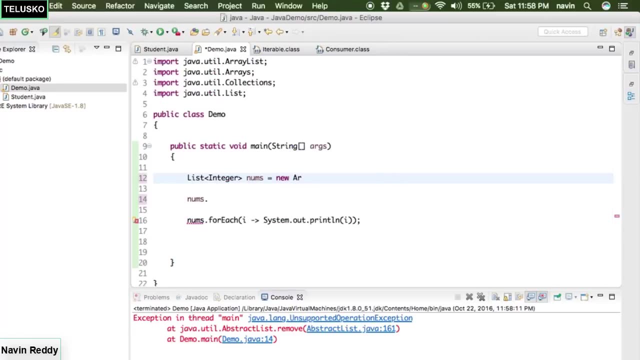 Oh, this is not working. Why is that? Is it because I am using arrays dot list. Okay, What arrays dot list gives you? Oh, It gives me the list object. So for that I have to Yes. to achieve that, we have to create the object of array list, the new array list. 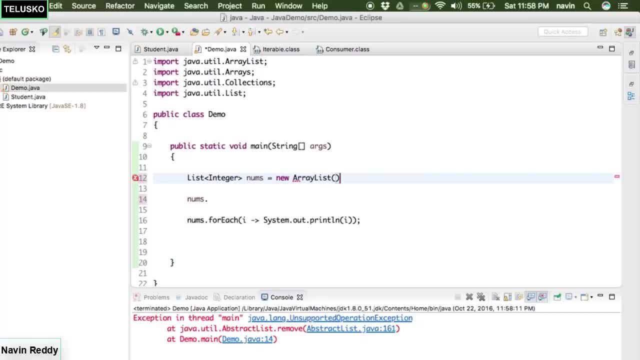 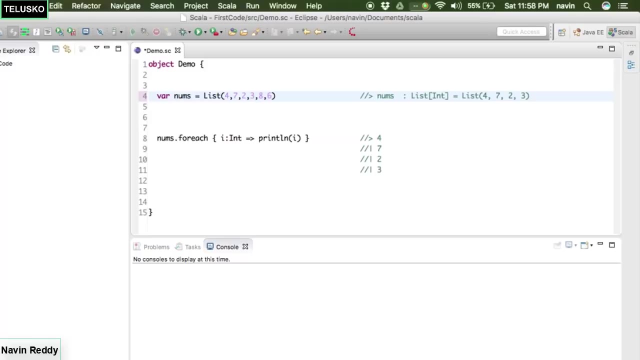 That is the way it will work Now, instead of going for the actual input values. Just imagine when you want to remove elements. we use that technique. But if you want to achieve the same thing in Scala, let's say I have these four elements or maybe some more elements here. 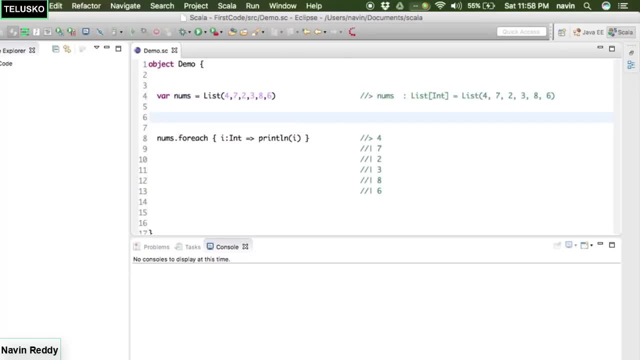 If I want to remove some elements here, we can simply say numsdrop2.. So what it will do is if I say numsdrop2, it will remove the first two elements. So if I remove first two elements, we can say drop2, it will remove 4 and 7.. 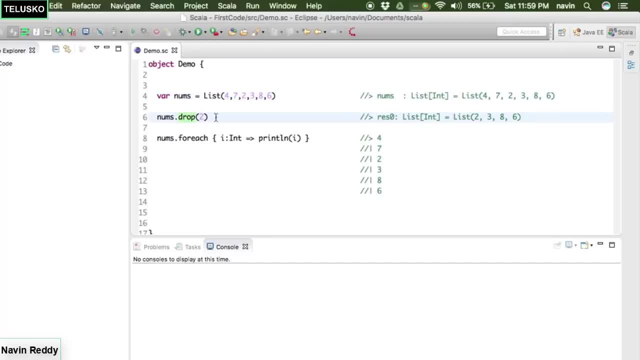 So you can simply use drop and we can pass 2, which will remove first and second. What we can also do is, let's say, I want to remove first two and I want to print next two. So I want to remove first two and then I want to print next two. 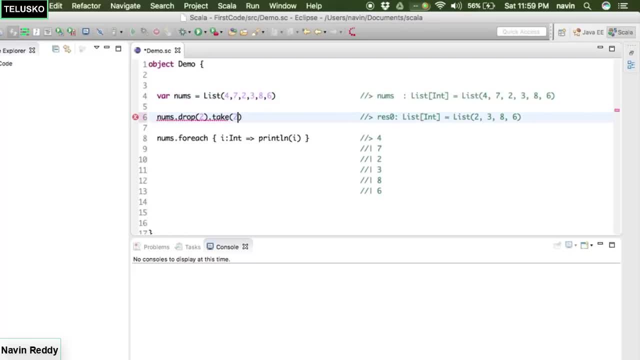 So what we can do is we can say take2.. So what it will do, it will drop first two and it will take next two. But again, we are not changing the original nums here. Every time you use any of this method, it will return you the object of at least, or it will return you the object of least. 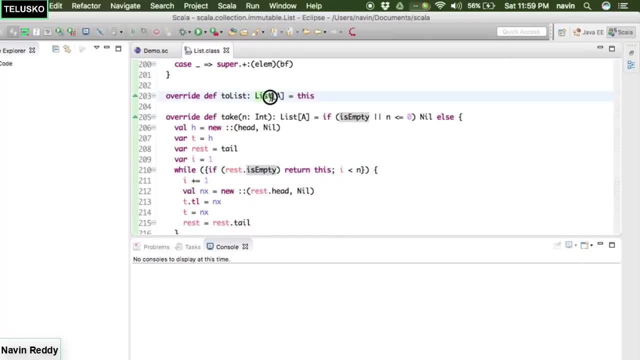 So you can see there is a definition here. It returns you the object of least here. Okay, And so that means nums is the complete values. Drop2 will remove the first two elements and then the remaining elements will be taken by take. So 2,, 3,, 8, 6 will be taken as an input. 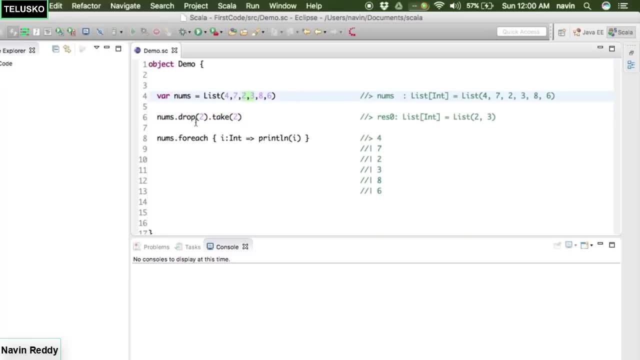 For take and take will take out only two values, which is 2 and 3.. Okay Now, since, since Scala has some syntactic sugar, which means that you don't have to use the dot operator there, You can simply use the English-like sentence. 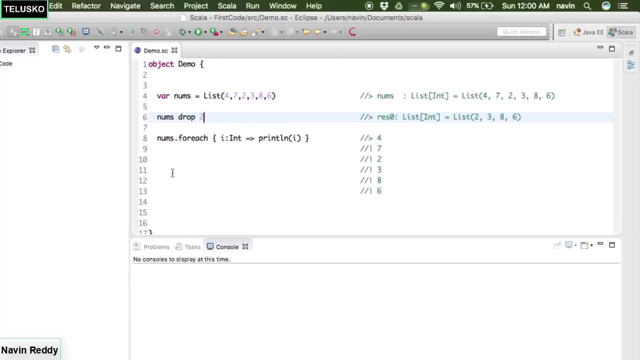 You can say nums drop2.. So what it will do is it will act like an English-like language, So drop will act as an operator between these two. Okay, So numsdrops in bracket 2, we can write in an English format. 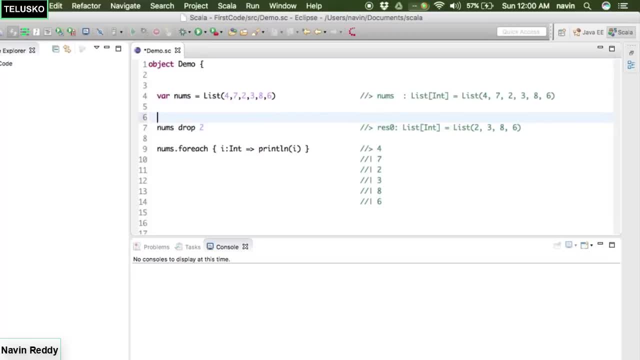 So nums drop2.. In fact we have seen earlier right when we say 7 plus 8.. So it looks like we have 7 and then operator, then 8, but actually it is a method, It's a function, right. 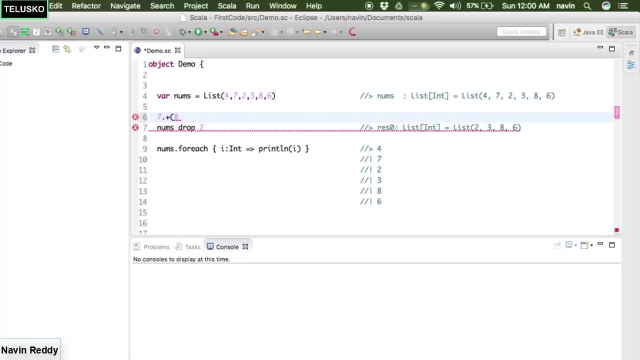 So we simply say 7.plus8.. Now why I'm repeating this same example multiple times? Because there is something very different in which is which is there in Scala, I mean, which is there which is not there in Java, right? 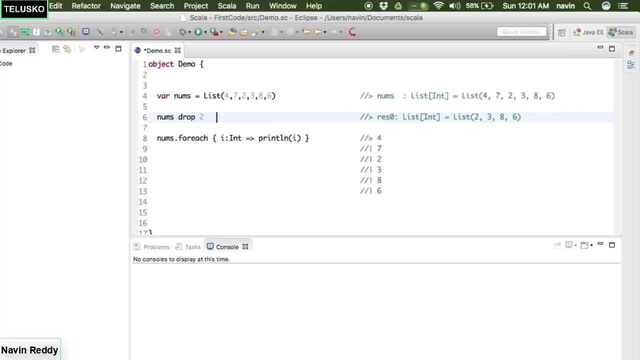 So we have to say nums drop2.. So it will take again. we can also write: take, take, 3.. It will take first three elements Now. I mean it will remove 4 and 7. Then it will take 2,, 3,, 8.. 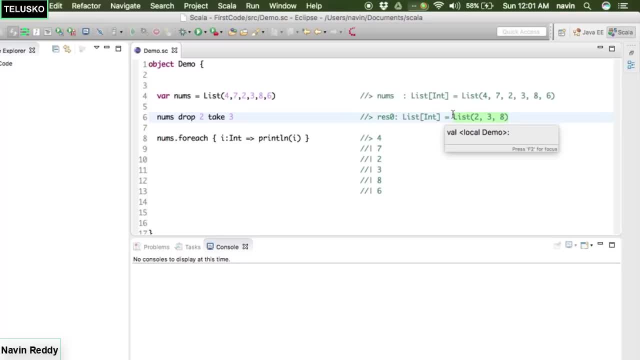 And that's what we are getting here, Right? So Scala is more like English language, It is. it has something called a syntactic sugar which we have used here. So, yeah, that's about Scala. That's how we can, that's how we can remove elements. 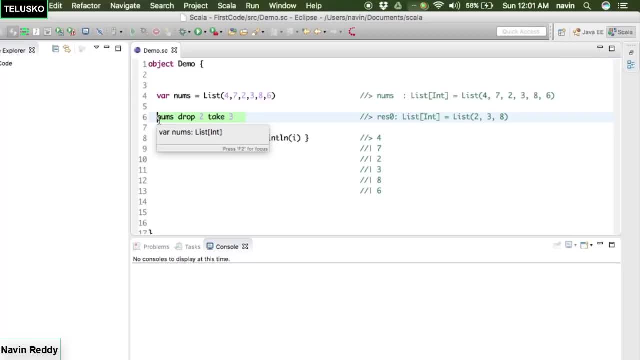 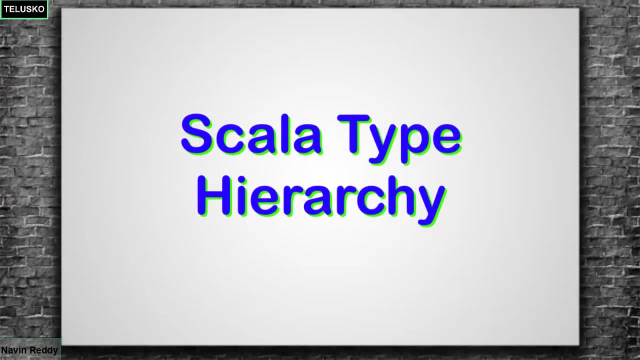 We can add elements and all that stuff. In fact, in the next video also we'll talk about Lists, But in I mean with a different, with a different intention of working with Lists. In this video we'll talk more about Lists. 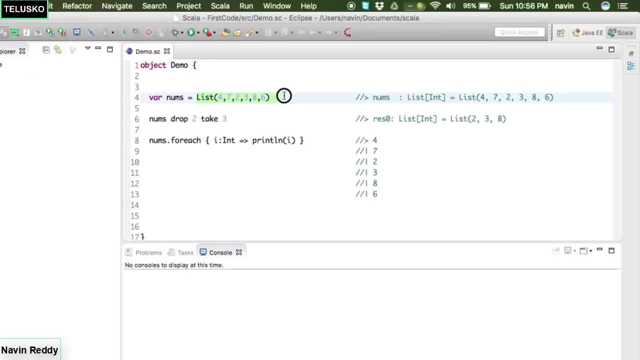 So in the last few videos we have talked about Lists a lot. right, We can add elements in that and we can perform some operations. So this is syntactic, syntactic sugar, which we have the syntax, where you can mention the method name without the dot operators, right? 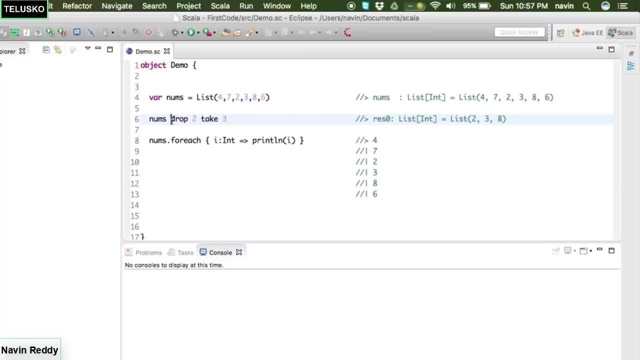 We have this object. here We are saying drop without using dot operators. That's fascinating for Java programmers, because we don't do that in Java, right? So what? what else we can do here, Right? So let's uh. so let's say, we have this list of uh, list of values, right where you have. 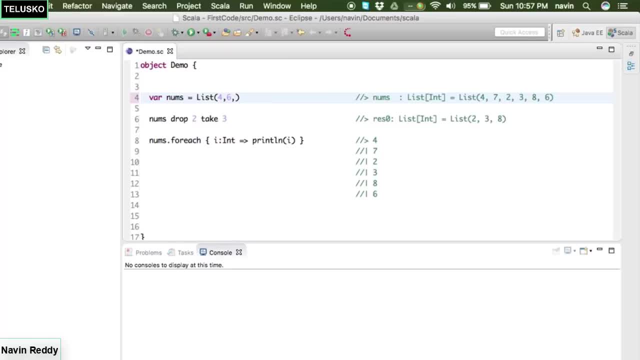 all integers. I mean, is it possible to put some values and a different type of value example: true. So now, true is not. uh, uh, it's not, uh. what do you say? It's not number right. 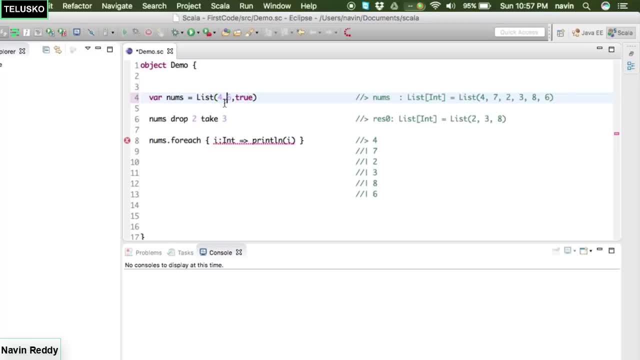 So four and six they're integers, but two is not an integer, Then how it will work? So if you run this code, you can see: uh okay, there's something wrong. I mean, there's lots of bugs here. 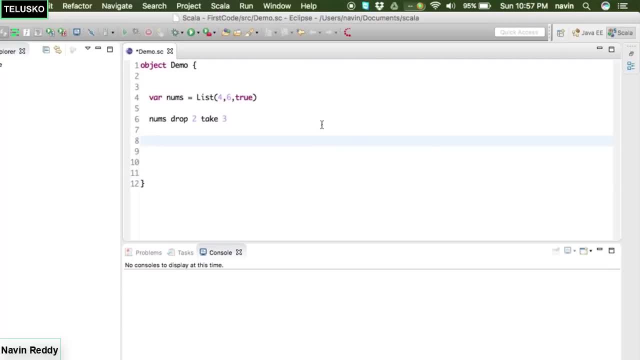 Let me remove this stuff, Okay, Yeah, So you can see we are getting a list, because if I mentioned a list of numbers, if I only use a list of numbers, it will return you a list which is eight, right, So it's detecting that you have all this: four, six, five. they are numbers. 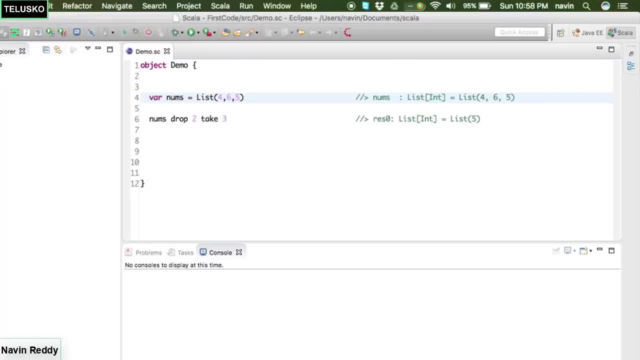 So it will return you the list of eight. But as soon as you add one more value here- which is true now, that's a Boolean type, right. So we have integer, integer, Boolean, So it creates an array of any value. 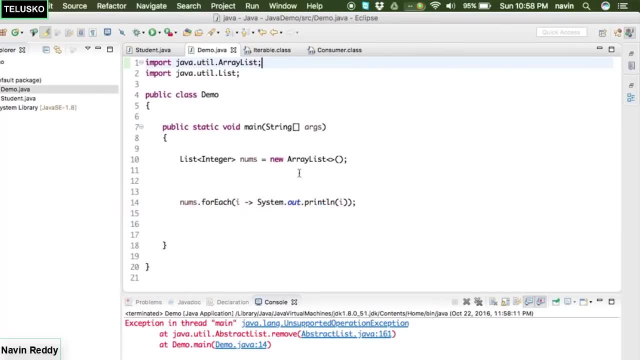 Now what exactly it means. because, when it comes to Java, what we normally do in Java is, let's say, if I create an array, when you say arrays dot as list, uh, you can be. you have to be very specific here. 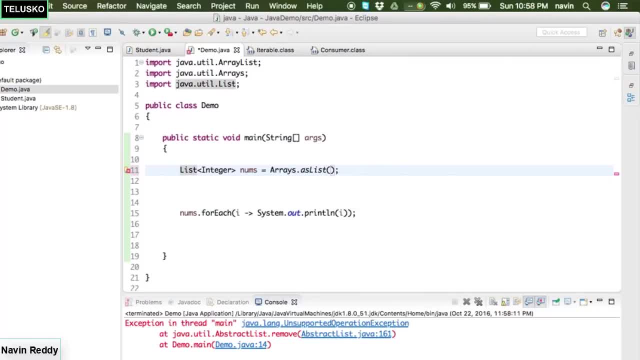 I mean you can have an array of numbers or you can have- uh, you're going to have an idea. Let's say, if I say four comma five comma eight, it will work right Because it is integer. but as soon as I write a true here now, there's something wrong, because 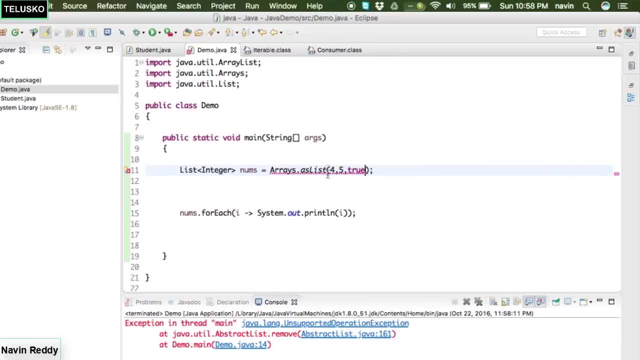 it returns, So it returns you the object. I mean it returns you the list of objects. You cannot put it integer here, so you have to put it object, right. That's what we have learned in uh uh in Java. 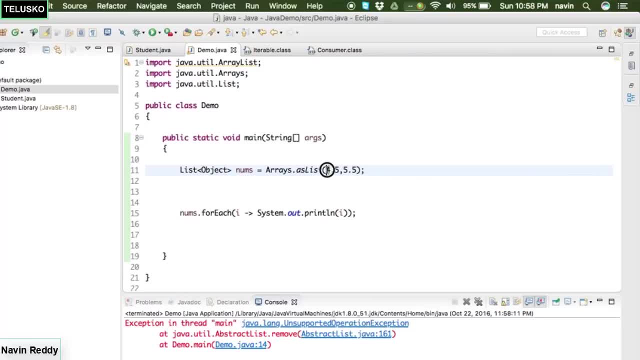 In fact, if you put 5.5 here, that's a double right. So this is this is integer, This is integer, This is double. So instead of having object, we can also write. I guess we can also write number, because yeah. 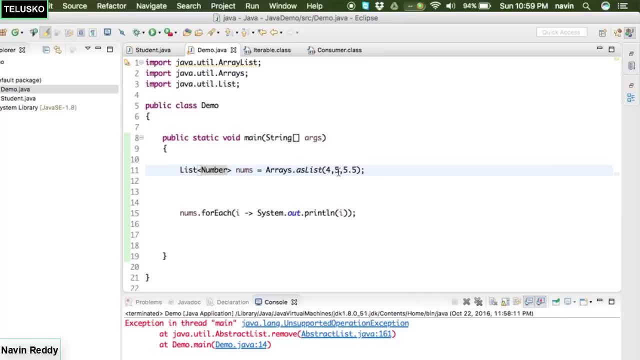 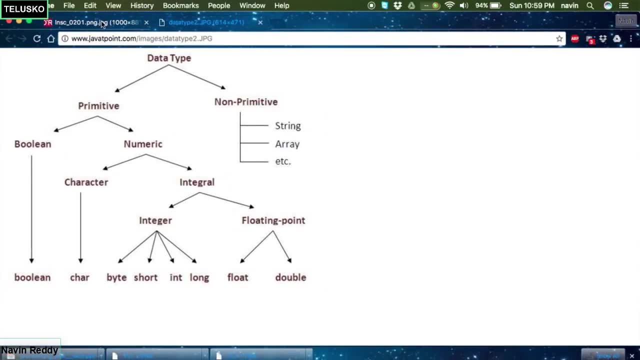 so because integer and double they both, they both, uh, are the subclass Of number class, right? So this isn't a hierarchy, right? So if you, if you look at the hierarchy here, so this is the Java hierarchy. 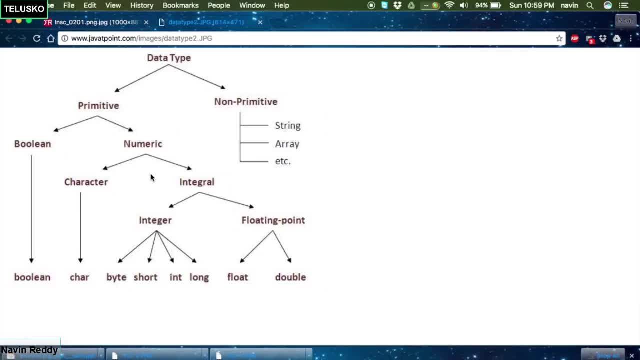 So we have data types. So on the top we have object and then we have primitive, We have non-primitive. So when it comes to string array, those are non-primitive, right, And all these classes, they actually extend an object class. 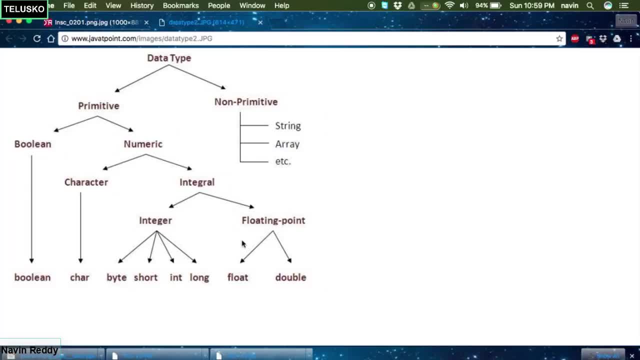 The same goes for Boolean character integer floating point. In fact, we use double class there. So these are the upper classes for you And then we have. So normally These are not the exact class names. uh, this is a different thing, but we have classes. 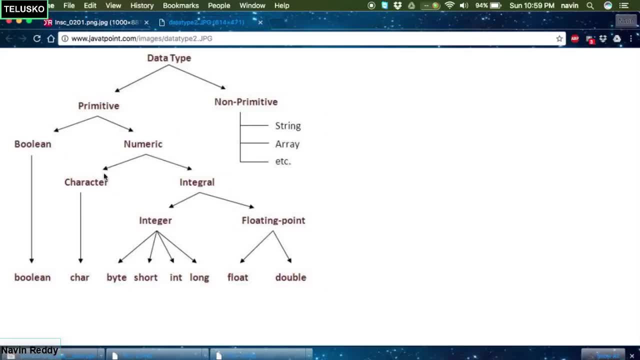 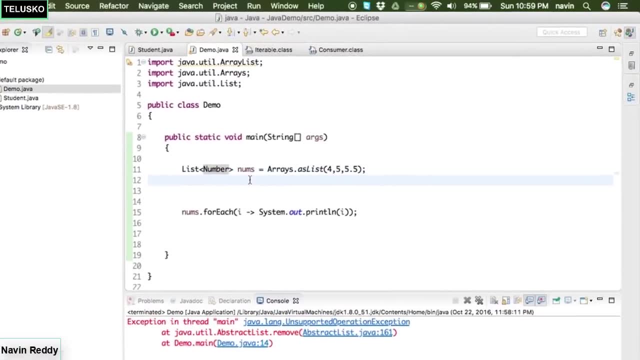 which extends object right. I hope you are getting what I'm trying to convey here. Example: when it comes to integer class and double class, both extends number right. So if I go to integer class, so if I go to integer and if I jumped to integer, you can. 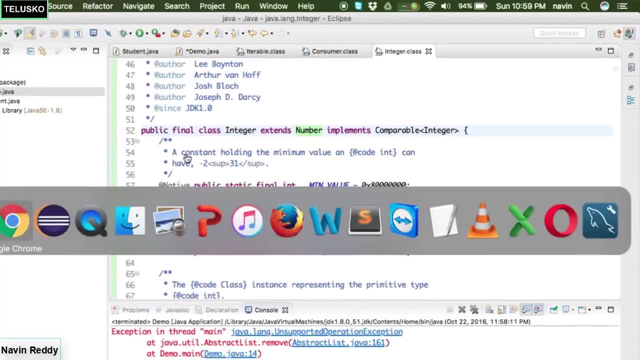 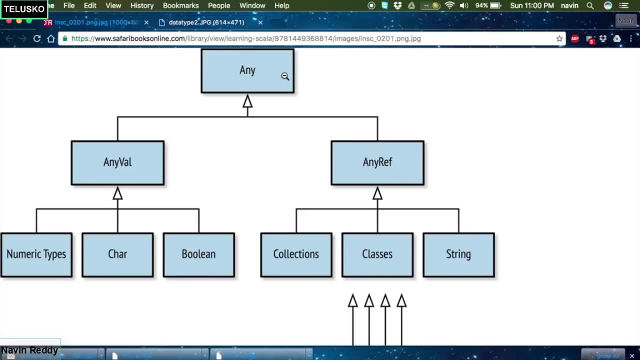 see it extends a number class. It same goes for double right. So that's the hierarchy for Java. But when it comes to hierarchy for Scala, we have the topmost hierarchy as any. So we don't have object that we have any. 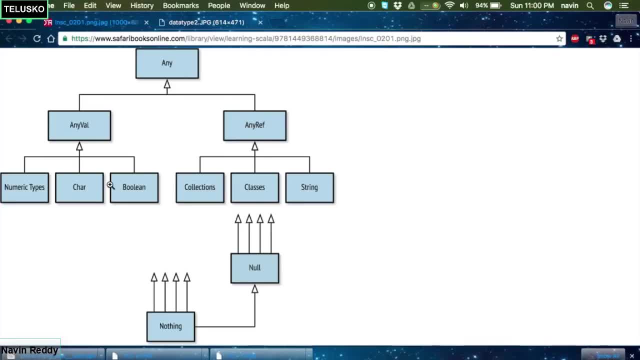 So any has two things: any val or any reference. So if you talk about primitive types or all the classes where you can store data, like Boolean, char, integer, all the stuff that belongs to any val, And when you have collections classes, when you have your own object, that's a part of. 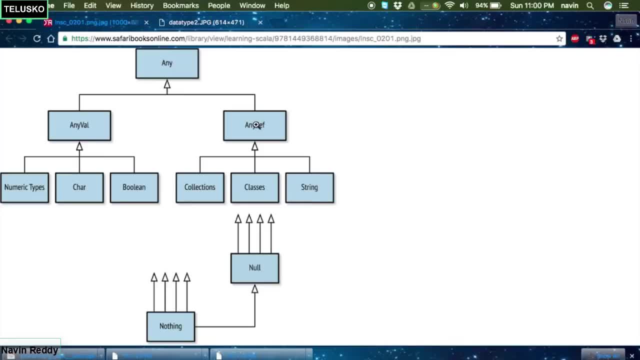 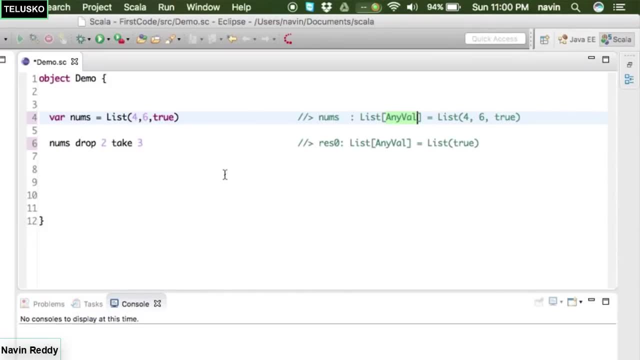 any ref. okay, So this, this is something different in Scala compared to Java. not very different, but it is something which is new. Okay, so that's how you specify the hierarchy here. So when you specify a number and a Boolean value, it will return you the value which. 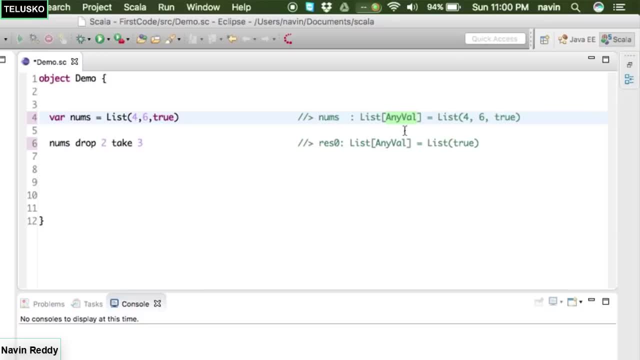 is, which is any value? But how about if I put a string here? So let's say, if, with this, true, I'm also putting a string like Naveen. Now what will happen is we have numbers, we have Boolean and we also have a string. 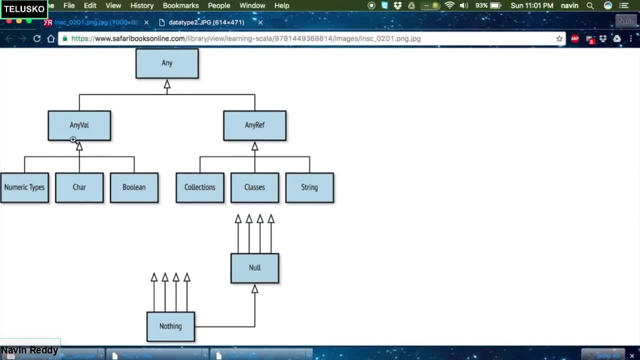 So it returns you any. because, as per the hierarchy you can see, we have a number, we have a Boolean type, We have a class object which is string, So it returns any. because you have to specify, you have to be. I mean, what do you say? 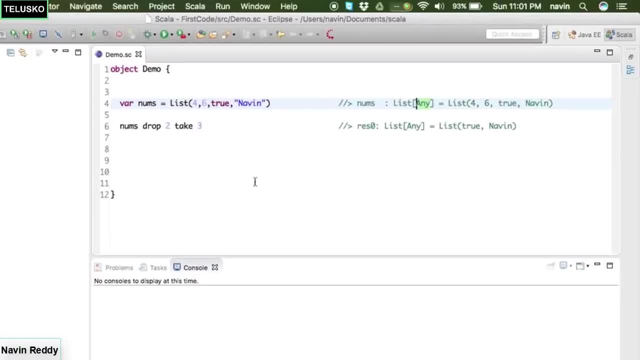 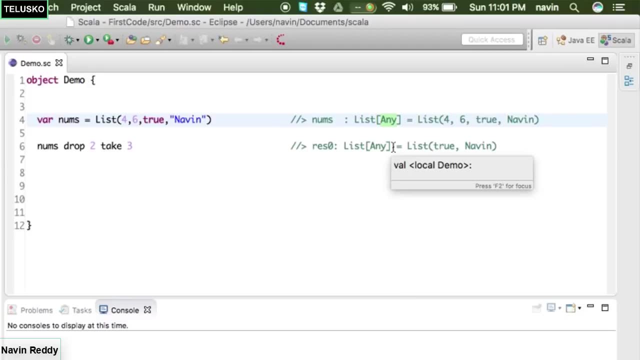 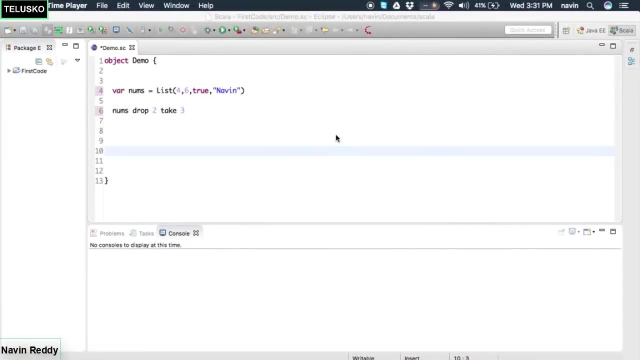 You have to be, you have to add up everything right. So it is any. So that's how you can work with the Scala type hierarchy. So now, once we know the basics of list and how exactly we store data, We can store data of different types, like we have. we can store numbers, we can store 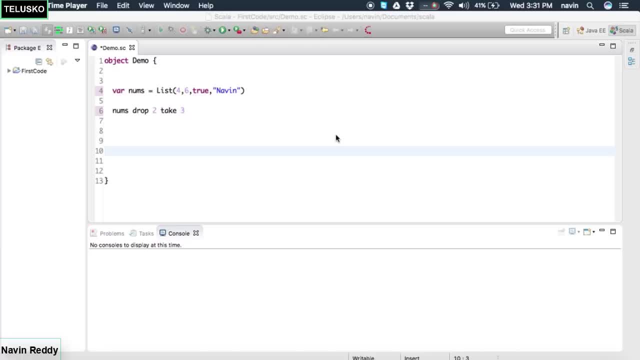 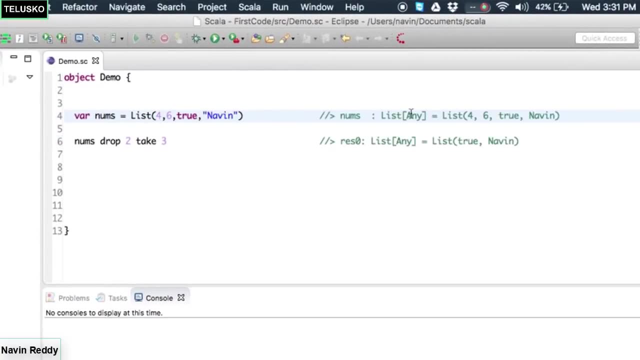 strings we can store, even, even we can have a list with different type of values. right Example we have. we have done that here, right? So when I say four, six true and Naveen, you can see the list, the type of list is. 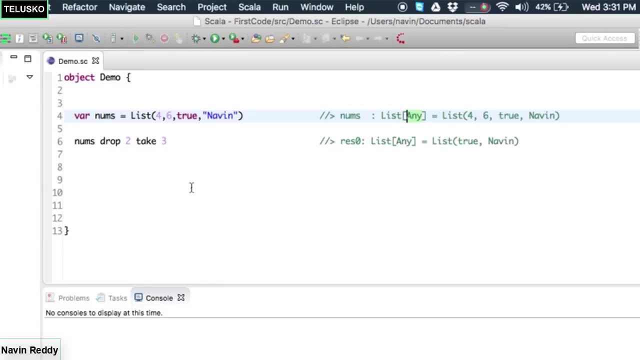 any right. We have talked about the hierarchy. What we'll do in this video is we'll talk about list again, but instead of going for primitive or the inbuilt type of objects, let's have our own objects. So something more comp, more complex objects in list. 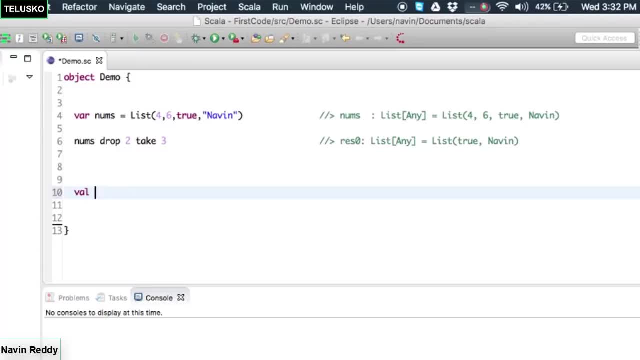 So how to achieve that? So what we'll do is: we'll say val, we'll say students. So I need a list of students now, and for that I need to create a class right, Because you can create an object of a student only when you have a class of it. 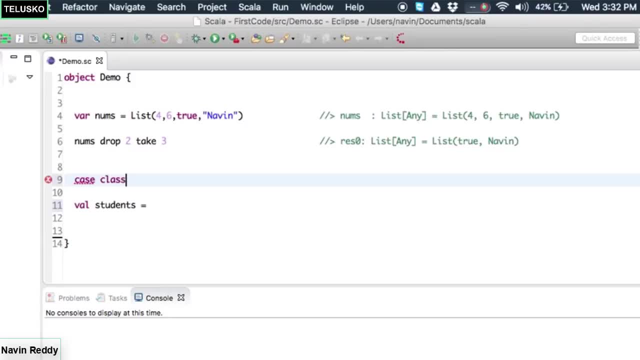 So normally, how do we create a class? We say case class, and then we mentioned the class name, which is, let's say, stood, and in this stood I will pass. I will pass three objects, Uh, three parameters as a, so we can also get a constructor here, right? 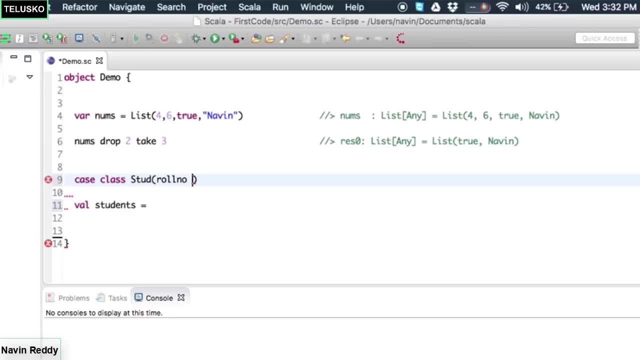 So we can see. my first value is roll number and the type of roll number is, let's say, ink. Then the next one is name, which should be string, and let's say marks, which is again ink. So we have this, we have this class which has the name is stood, and then we have this: 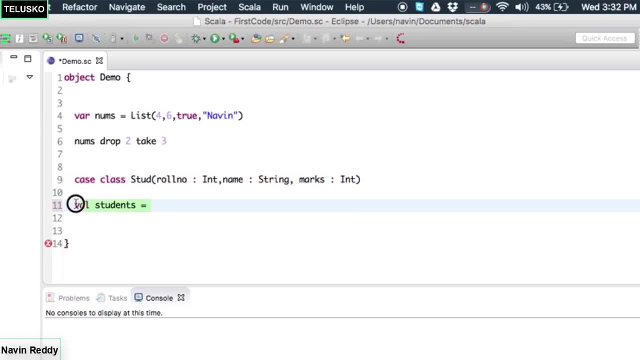 three, three types there. and now let me just remove that just to see. the output is they're getting the class there Once we get that, So let's go ahead. and yes, we got, we got our class. Now let's create the object of it. 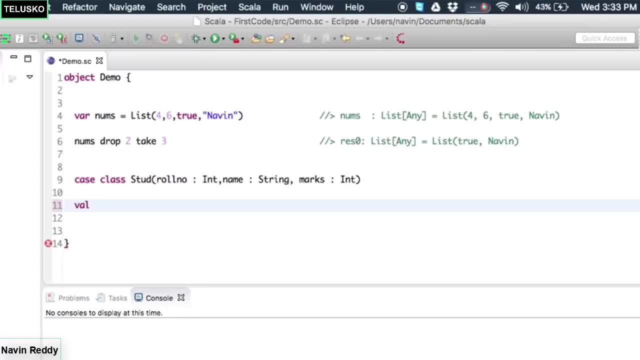 So we'll say val, and we'll simply say uh, students, and then equal to so. let's create a list of so, let's create a list and in this list I will create the first object of student. I will say stood. I will pass multiple values, since this is a list, right where you have. 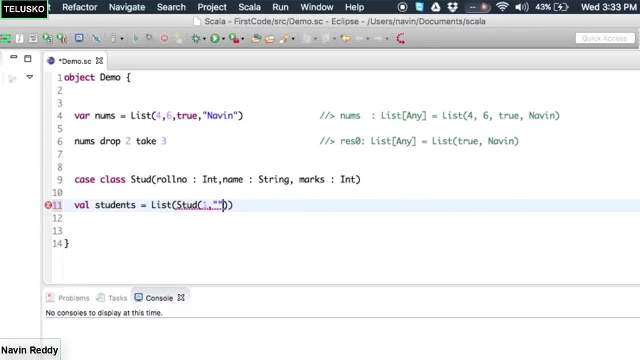 to specify multiple values. So I will say roll number. one name is, let's say, Naveen, and the marks I will assign is 40.. That's my first object. Let's say the next object is student. uh, we'll say this is two. uh, that's two. 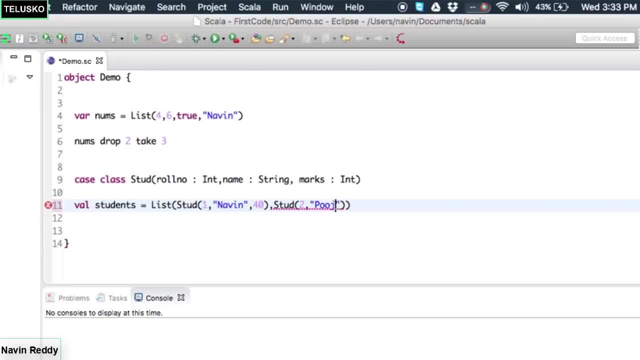 Uh, we'll say: name is Pooja, and then we got marks, as let's say, 80. that's, that's the marks, Let's go for one more. We just stood three, uh, Naveen, and we'll say: this is 60.. 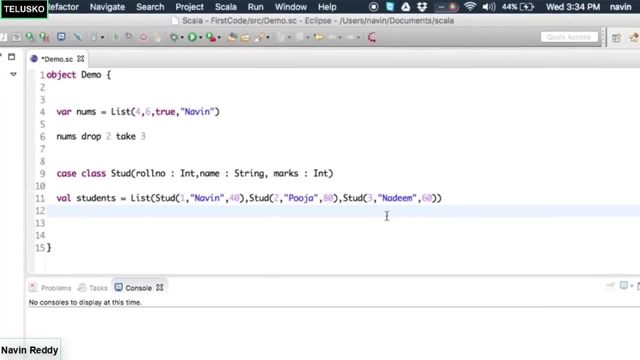 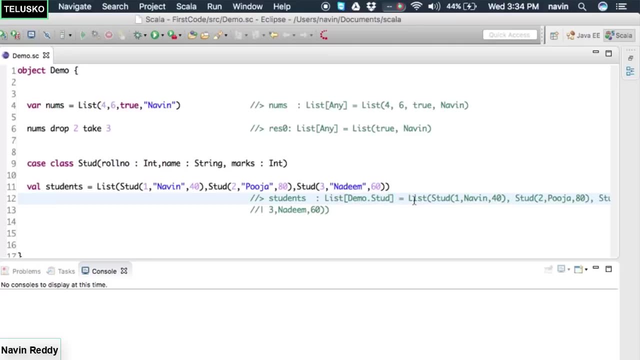 That's it, That's our list, and you can see, once I run this code, I mean once I save this code, you can see we got a list of students here. So this list is of type stood right. So we we have the three objects here. 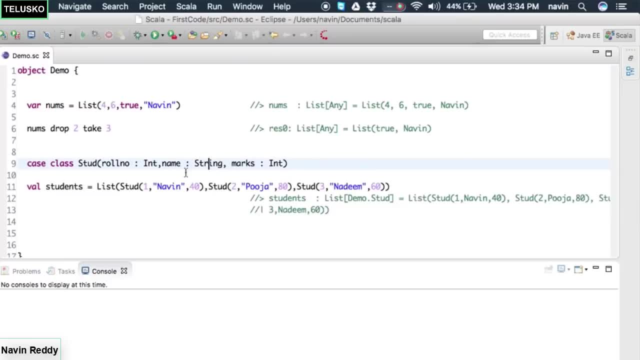 Okay Again. uh, if you're not getting this, this thing, that's okay, We will be doing so. We'll do the. we'll do the same thing in Java once we're done with this example. So we'll get the complete idea how list works in, uh, in Scala. 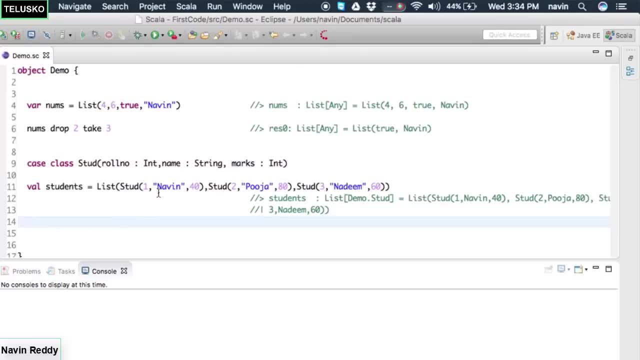 So we have the, we have the list of student here, and now we can perform certain actions, right? So, before performing some action here, let me, let me see how to do this in in Java. So let me, let me go back to my Java code, which is: this is Java code here: 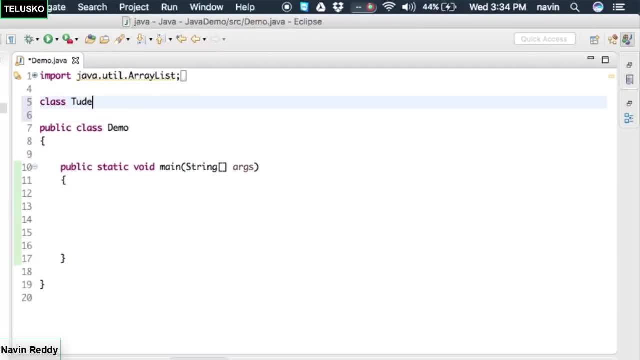 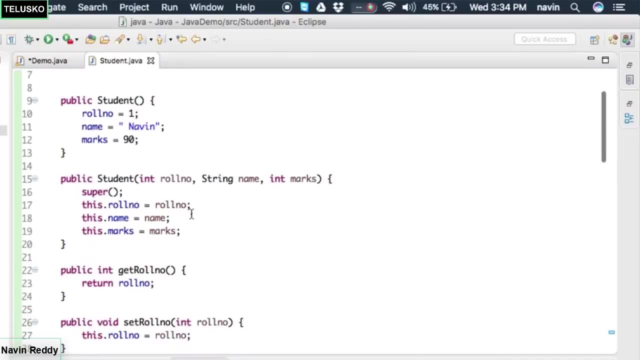 And let me create a class here, the same class which we, which we were doing there. Let's create a student class. In fact, we have a student class here. Let's do some modification. We do have three. we have. we do have three things. 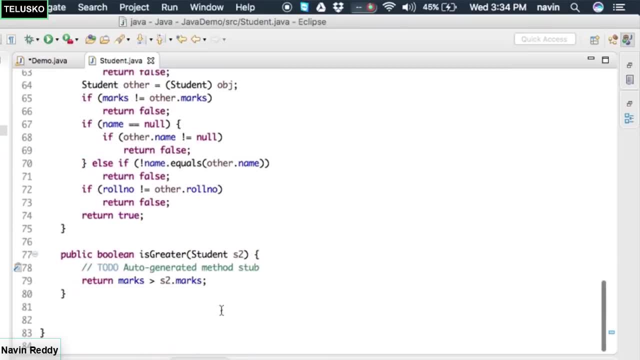 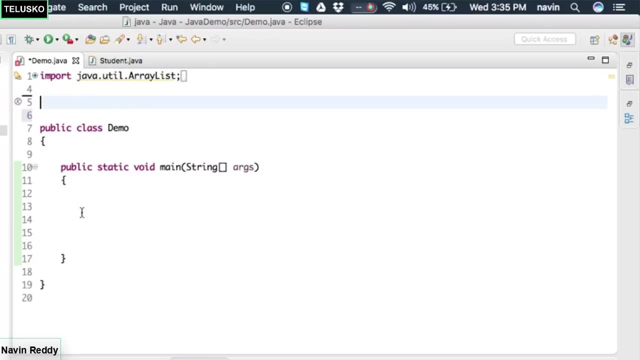 So everything is done here. I mean, we already have a class. Let me remove this thing. In fact. Okay, Uh, we have that part right. So now what we'll do is we'll simply say this is list of- uh, we'll say list of- student. 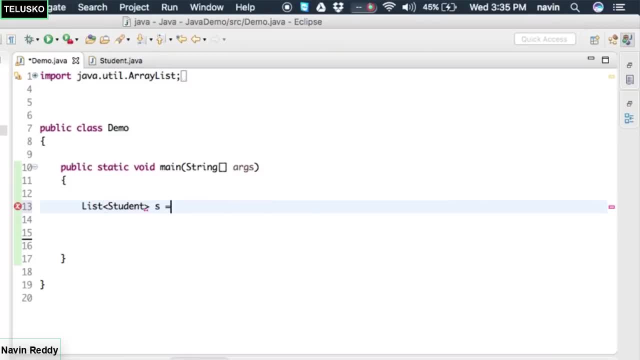 That's how you do it in Java, right? We have to create a collection. We'll say S, or let's say students, or students equal to. we'll say new, or we can directly use add a list, Or let's do that. 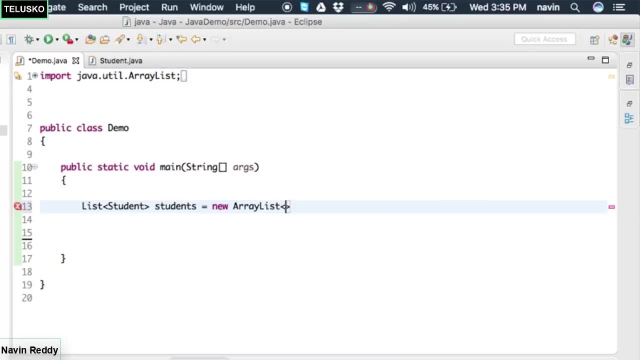 Let's say, uh, new, add a list. And so we, we got that, We got this list object here. Now, once we got that, let's add some objects here. So we'll say, students, dot, add new student by passing three values. 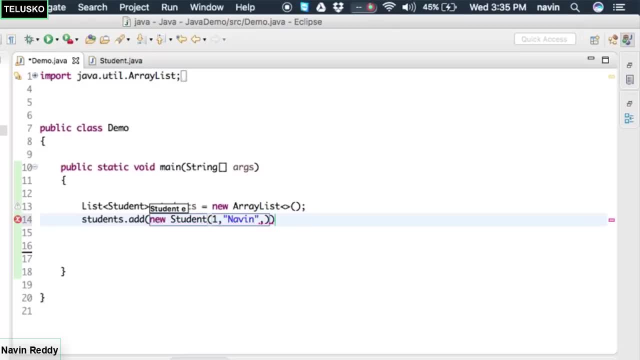 We'll say one, the same value, which is Naveen, And then we'll say: this is a 40. That's my first object. Then we can add two more objects here. We can say: this is two, this is three. 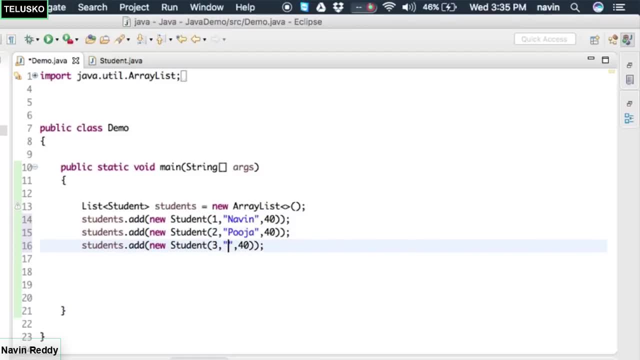 Uh, this is Pooja and this is Nadeem. Now, this is 80. And this is 60. So once we got the three objects, let's run, let's print all the values here. So it's a student as colon students. 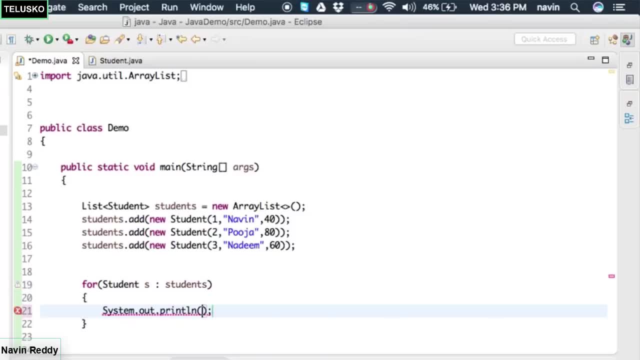 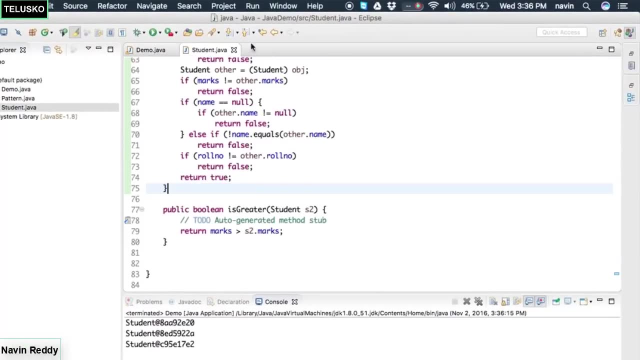 That's how you print the values, right, Using enhanced for loop, And we can say, as we can simply print the object itself, right, If I run this code and you can see, we got the output of. unfortunately, I don't have. 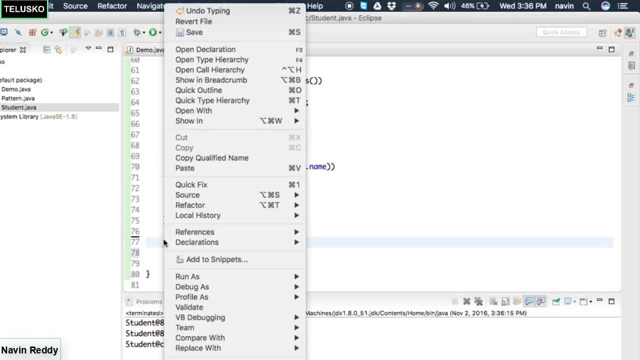 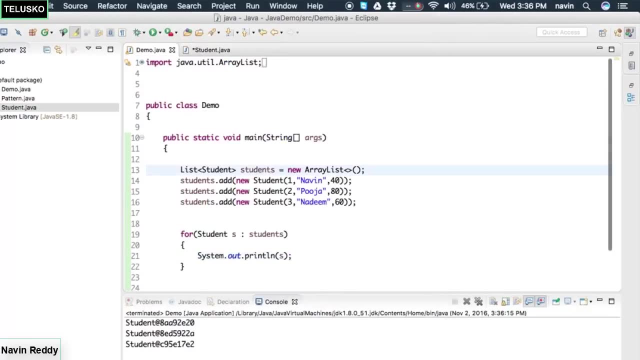 two string method here. Let me do that. Let me say right leg, So two string. I want to print all the values. Okay, I hope you're familiar with two string method And if I run this code now, you can see we got the. we got all the values here. 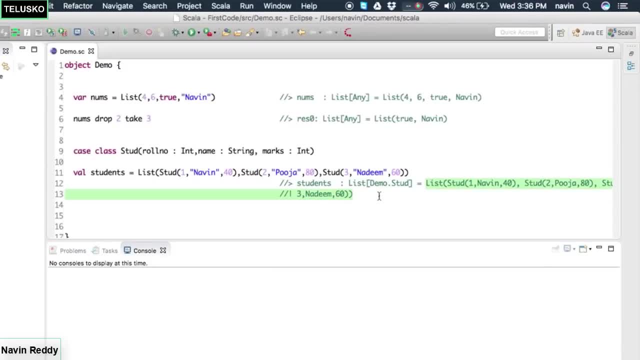 Now, if you compare, we have the same values here, right, We have the same output there, but the only difference is we have to write multiple lines of code here and we just have one line of code in Scala. Okay, Now, once we got the list of objects, what are the? what are the features? we can we 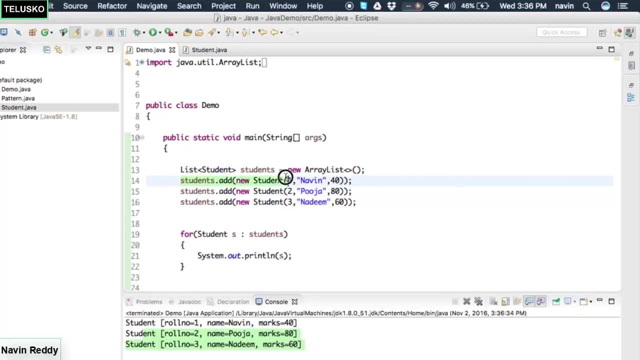 can achieve here. So let's say in this, in this list, if I want to print only one, uh, there are lots of code you have to write right, You have to use s dot, uh, students dot get, and you have to specify the first index number. 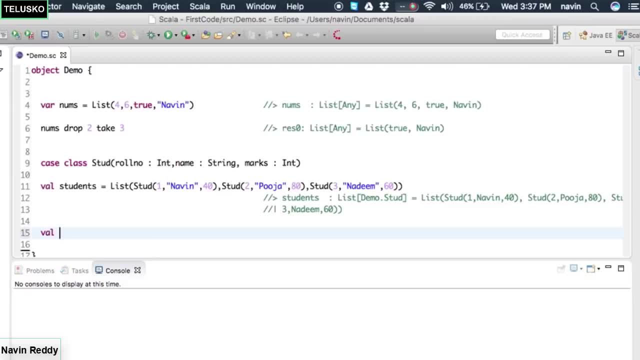 In Scala, what you can do is you can say: well, first, equal to students dot. So there's a method called as head. But as soon as you say not method, yeah, there's a method called as head- As soon as you say head, it will give you the first element, because this is the first. 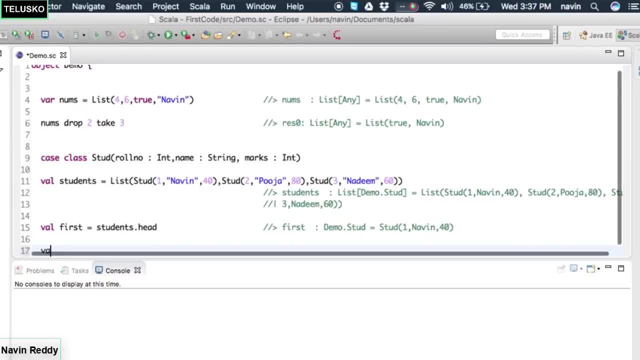 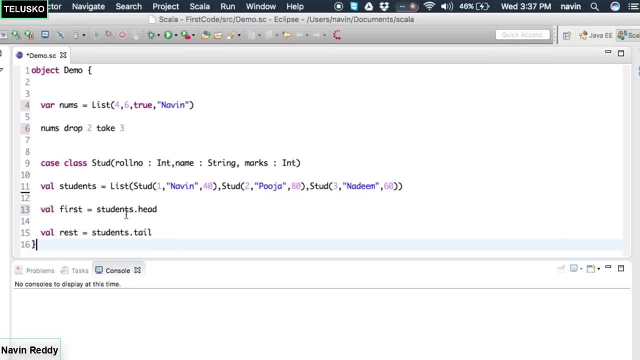 element, right? So when you say head, it will give the first element. Any guess, if I say uh, if I say students dot get Okay, Okay, Students dot tail. So we have one more method, which is tail. 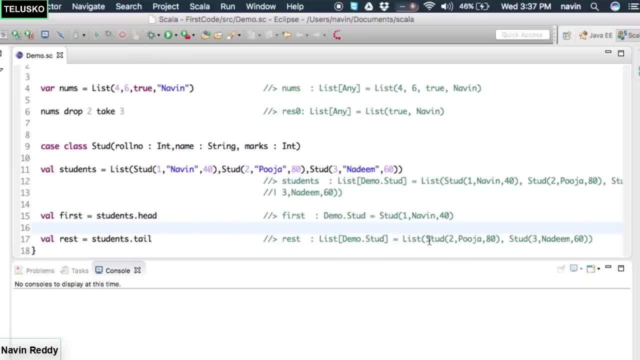 So your guess is right: instead of getting the first one, we're getting everything. So when you say head, you will get the first one. When you say tail, it will give you all the remaining elements. Now again, if you say we can also do that, we can say tail, dot, tail. 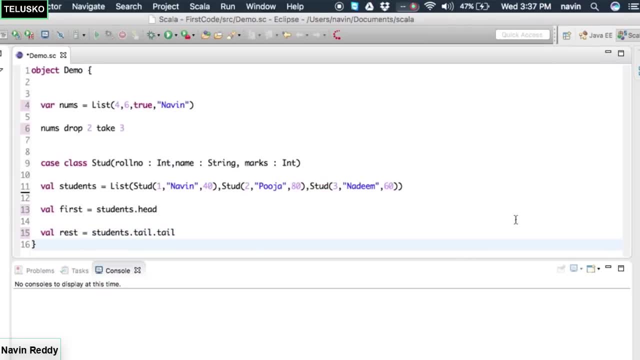 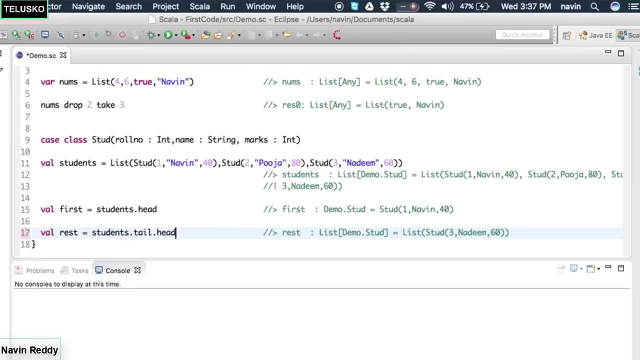 So tail dot tail will give you the tail of the tail, So it will give the last value itself. Is it working here? So we got the last value. Uh, we can also achieve tail dot head, which will give you the tails first object or the. 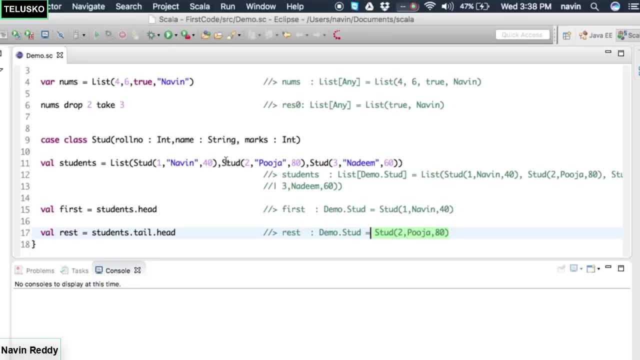 first element. This is the second one. right? So this is tail. right, This is tail and head out of it is this one. So we can use this one also. right, So we can use this head. We can, we can use head and tail as a function, as a method. 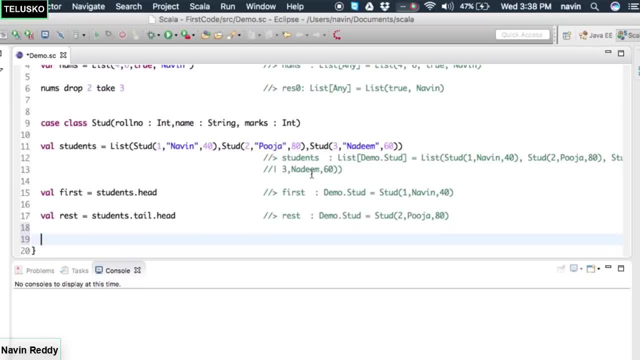 I mean there are lots of methods we can, we can work with. Now, what else we have? We also have some methods like, let's say, let me get a valve, and we'll say I want only toppers, So I want- when you say toppers, I mean those people who are getting marks about 60,, 50,. 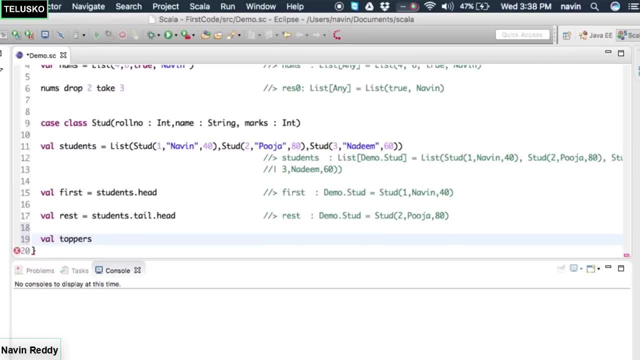 60 or more, Okay, And so I mean about 60, 60 and 60 and more, 60 and more, Okay. So what we'll do now is I want to only those people who are about 60 or 60, about 60. 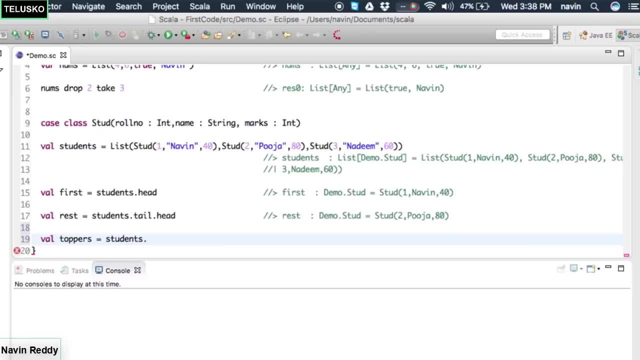 What we'll do is: uh, this students list. it has a method of this filter. Okay, So when you say filter, what you can do is in this filter, you just have to pass the condition. Now, basically, how do you pass a condition? 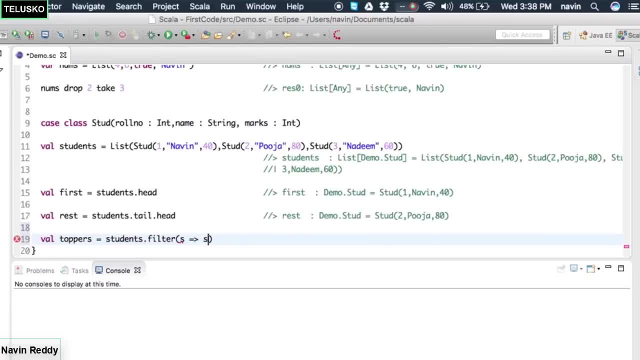 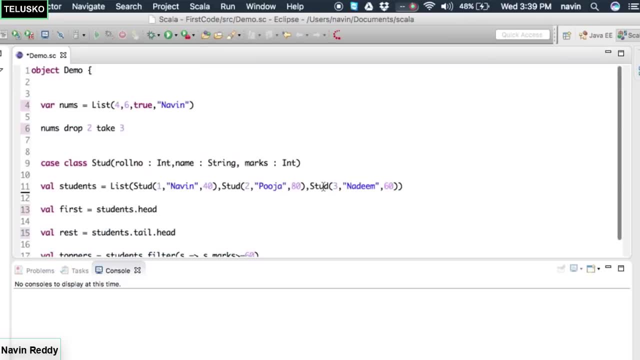 I can simply say s Uh, uh, s, Uh, s, S dot 0.. S dot, 0.. Zero, And we'll say s dot marks should be greater than or equal to 60. So I've specified a condition here. 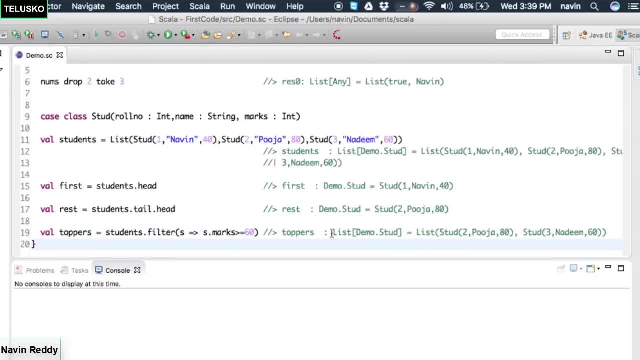 Again, again. we'll see this in Java, how this works in Java. So you can see: we got uh, we got least, we got uh 20, I mean we got 80 and we got 60, right. 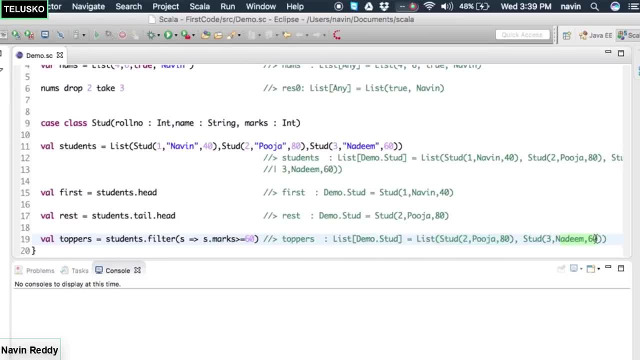 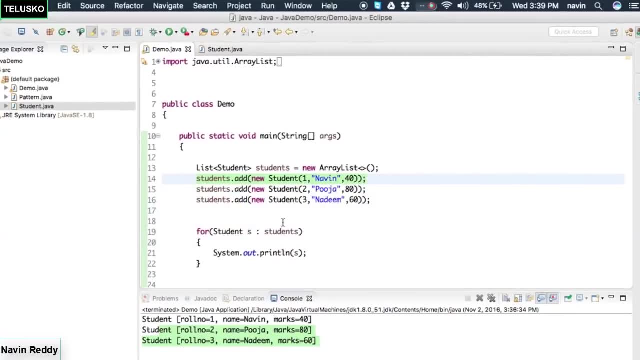 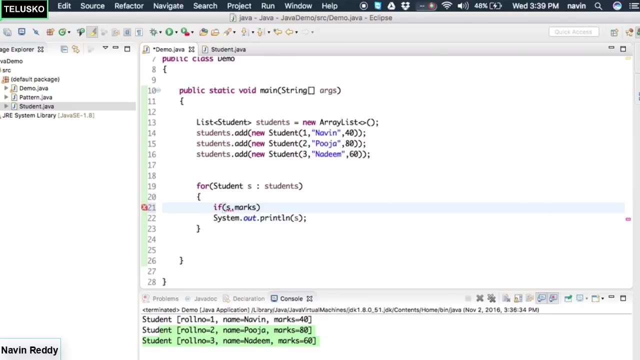 So when you say filter based on the marks, you're getting. you're getting these two things. we're not getting the first one, which is 40, because it is not satisfying the condition. Right, Right thing in Java, in this forward loop, we have to say if smarks is greater than or equal. 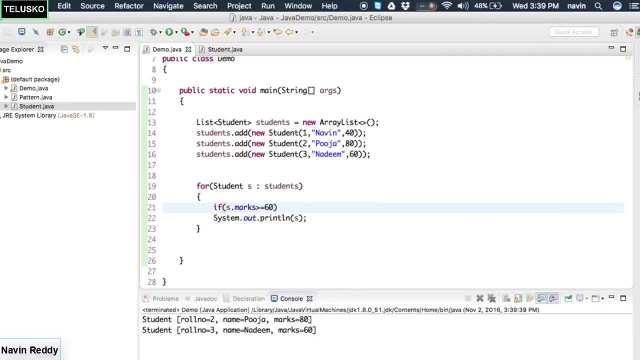 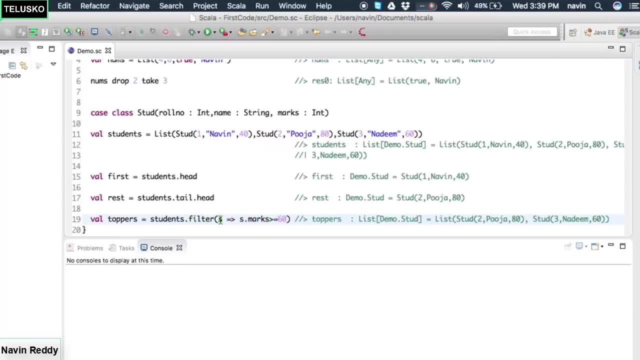 to 60, then only print, right, so it will print only those objects which are satisfying the condition. the same thing you can achieve with the help of filter method. so in this filter you have to pass the object, so it will take one, one object and it will satisfy the condition. 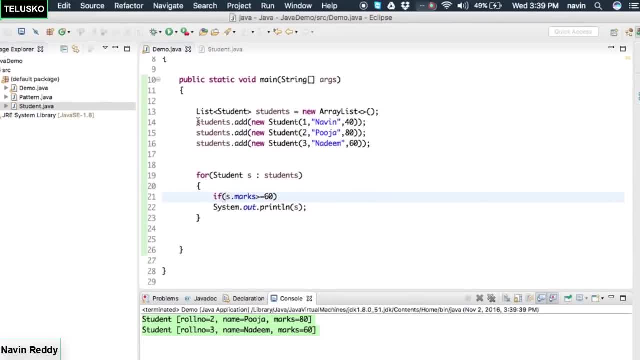 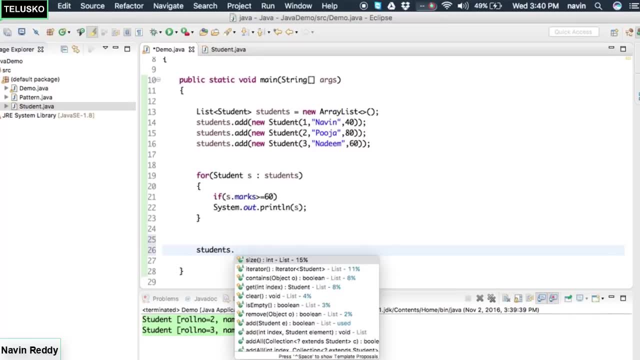 still, if you are not happy with this, let me explain this with the help of Java 8 concept. okay, let me just do that here. so how this works in Java 8 is: we have to say studentsfilter. so there is a first of all. we have to say studentsstream, okay, streamfilter, in fact. 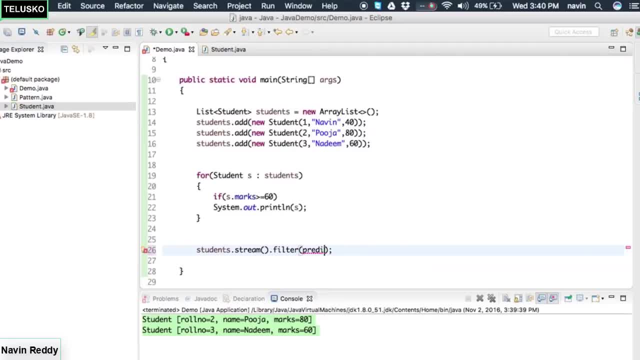 we have filter in Java also, so it was introduced in Java 1.8. it was not there earlier. okay, so in Scala we can use filter. even in Java we can use filter, but only in Java 8. it was not possible before that, And okay. so this is one way, this is one way which we have done. this is the. this is the. 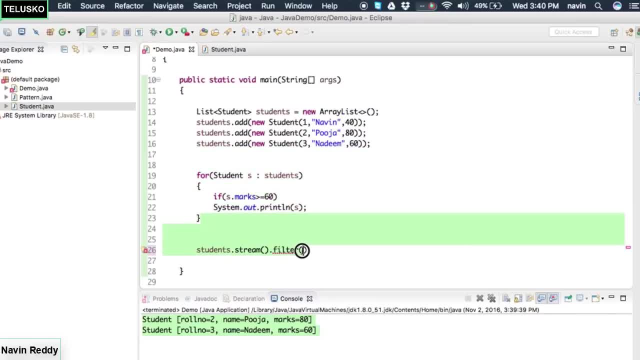 imperative type of coding which we can done in Java 7, also in Java 8. what we can do is so when you say filter, so filter will ask you. so if I go to filter method, which is which belongs to stream, it is asking you for the object of predicate, so I need to pass object. 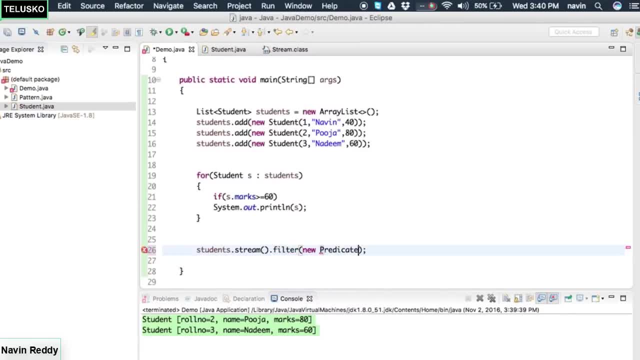 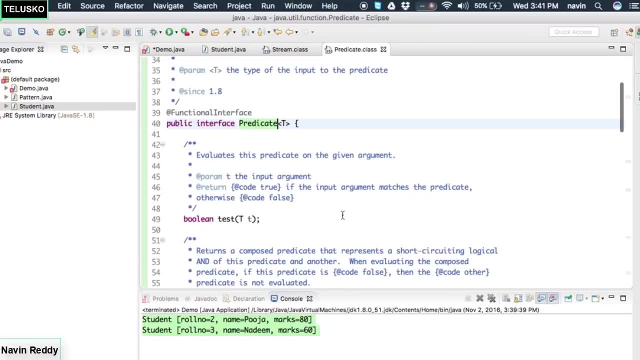 of predicate, right. so predicate is basically an interface. so if I go to predicate, there is a link. okay, if you want the complete description how that works in simple step, you can go to my. I will go to description area. there is a link for the for how this predicate predicate. 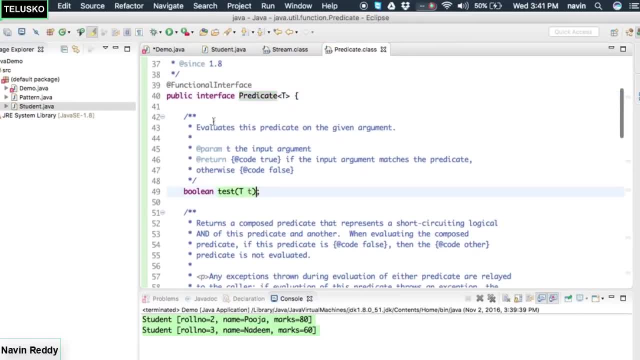 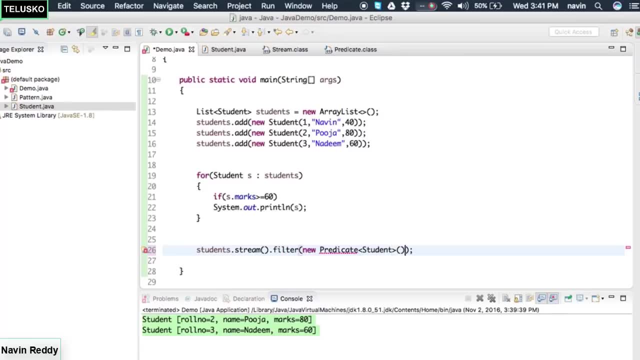 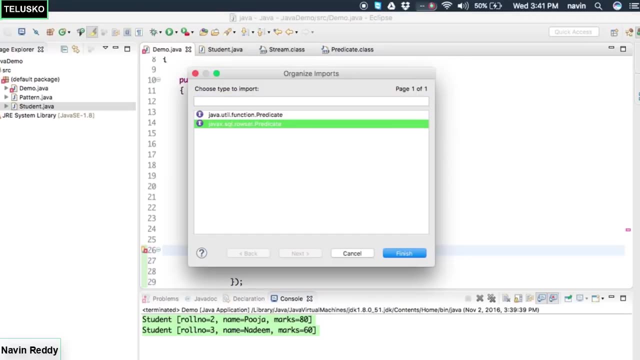 interface works. so just you will get that idea from that. so it has a method called test and it is an interface. so we have to say new predicate for students and let us define the class itself here. this is anonymous class which I am creating here. let me import the package. 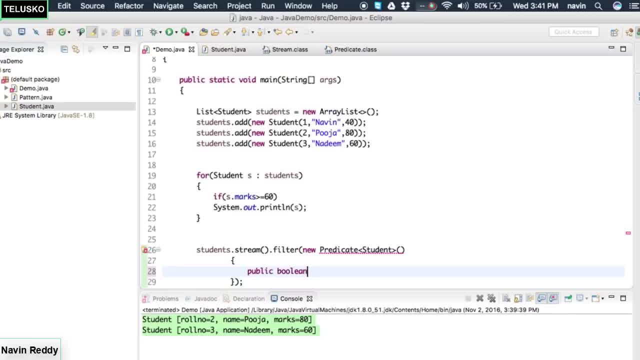 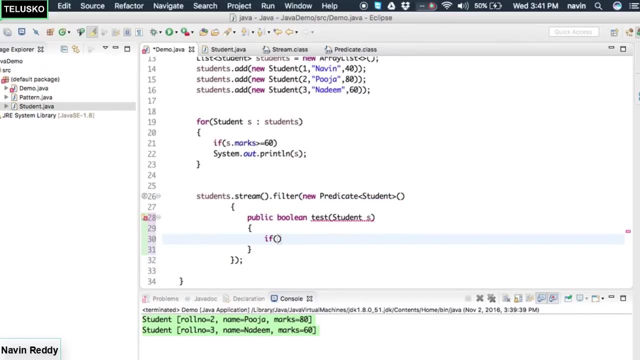 predicate And the method name is public boolean test which accepts. is it boolean? yes, it is boolean and we will say: this is test which accepts the integer value or this will accept the string student value and we will check if smarks is greater than, equal to greater than. 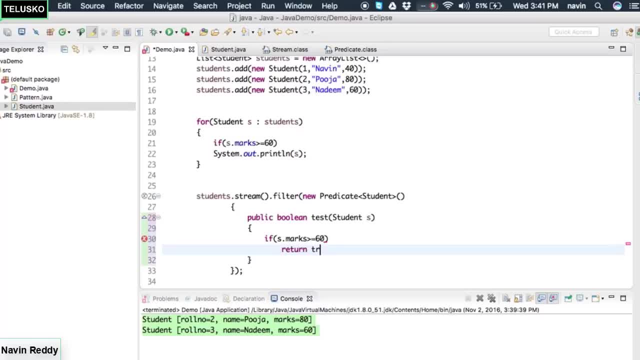 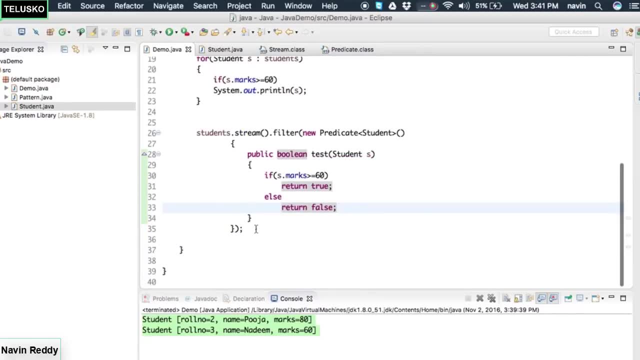 equal to 60. return true, else return false. Okay, so we got this stream and I can print all the values of stream by saying for each And we can pass. we have done with for each right. so you know how it works. so I can say: 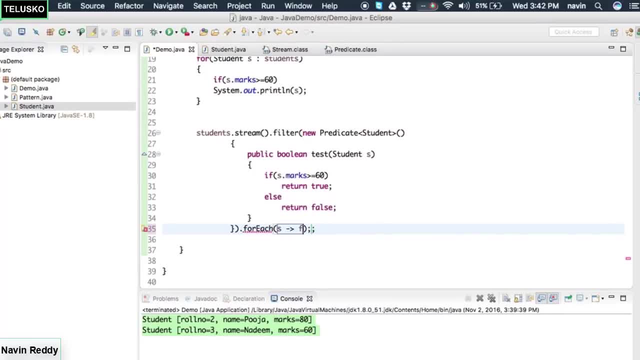 s colon: System dot out dot print. that's not right. the system dot out dot print ln is not working here. system dot out dot print ln And we can pass the value, Which is s itself. Okay, so what I am doing is I am finding the stream out of it, I am filtering out all the 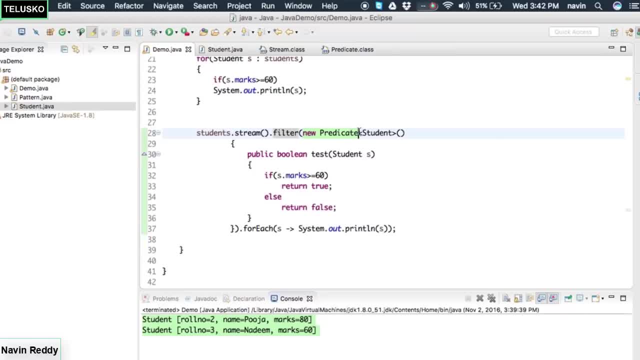 elements based. so we have to pass the object of predicate again. you will find the link in description area. how exactly predicate works. it takes the method as a definition and you can print all the values so you can see. even that works the same way. so you can. 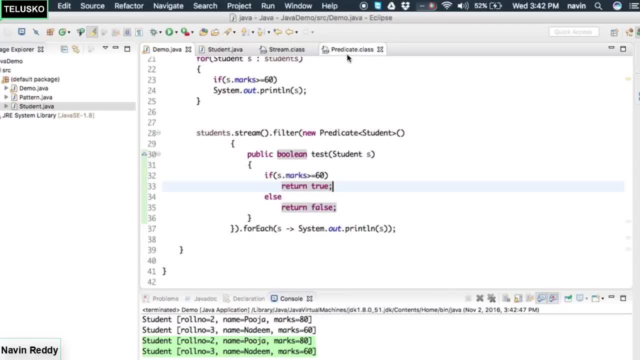 say, this output is because of the predicate. now, since predicate is a functional interface, you can see, it's a functional interface And whenever you have a functional interface, we can use lambda. what it simply means is: you don't have to mention from here to here. 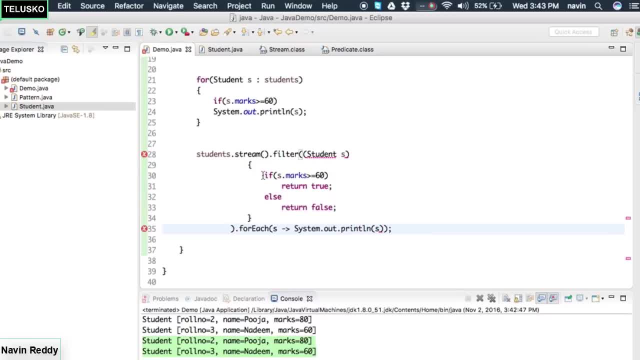 I'm just assuming that you know lambda expression. if you don't just go to my channel again, I will. I will paste the link there in the description- how lambda expression works and in fact we can show, if I think the if condition, where there we can simply say: even this will work. 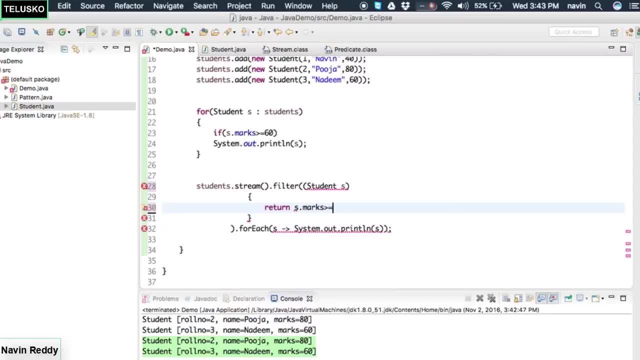 right return s dot marks Greater than equal to 60.. Okay, Okay, So if you have only one statement, we don't require return. we don't require this curly brackets, if you have only one statement and you can write everything in one line, provided. 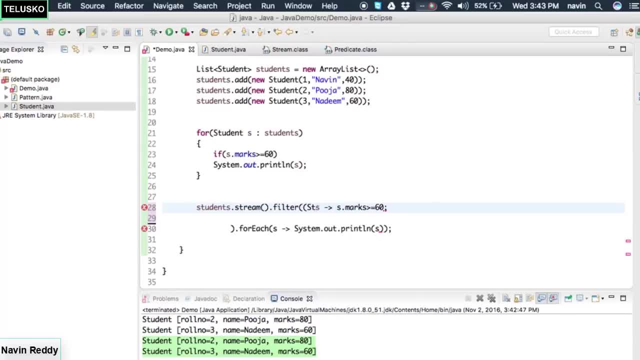 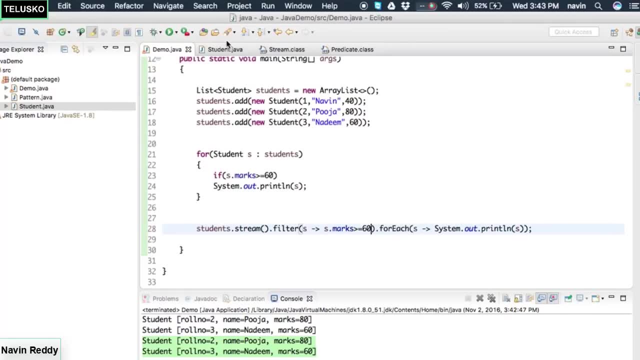 you have an arrow there, so in Java we use single arrow, right? so this is the same thing we are doing, right? we are saying: let me just write here, so that's the same thing we are doing. so if you are on this code, you are getting the same output. so we are filtering and we. 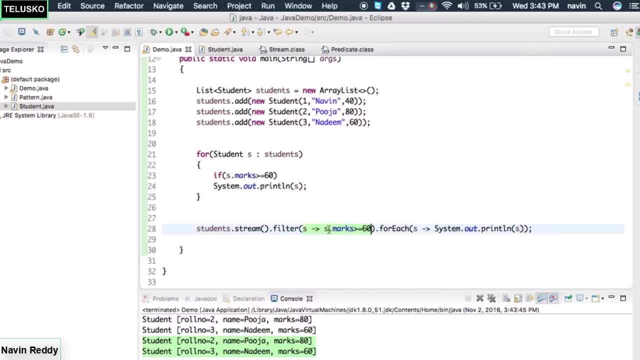 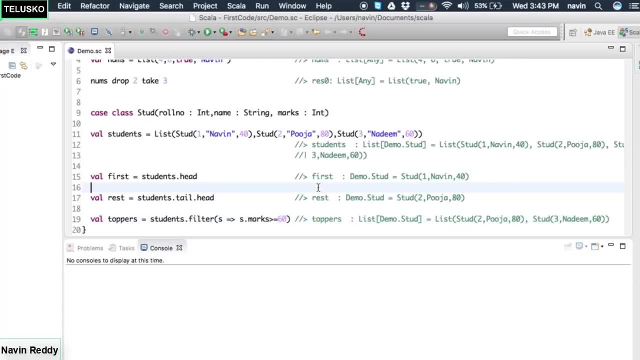 are passing the object of, I mean which are passing the lambda expression. so in Java, lambda expression is done with the help of single. I mean hyphen, arrow or hyphen greater than sign. in Scala we use equal to and greater than sign. Okay, so we can, we can use filter. in fact, we can also do partition based on this. we can. 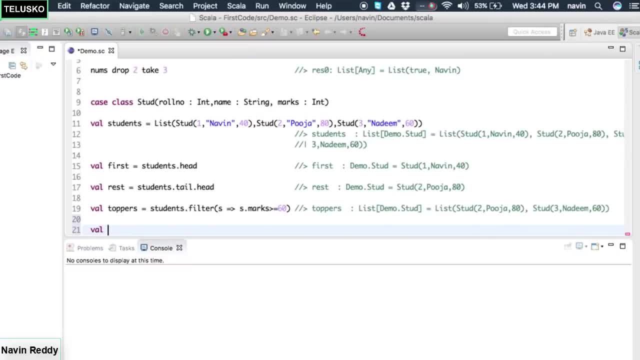 say val, we can say: what, how do we do partition here? Okay, so we can say: so what I want partition is I want people, so person who scored below 60. There should be one partition, one if you are scoring about 60, that should be one partition. 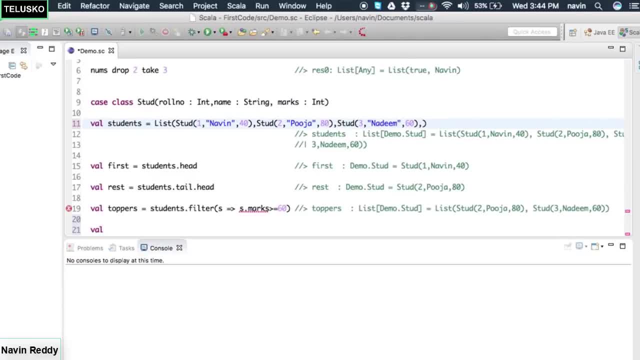 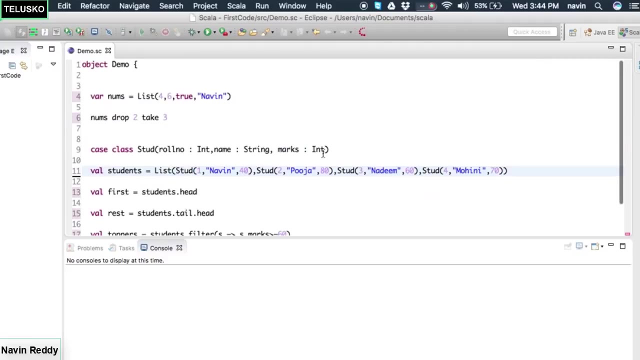 let me add one more object, just to give you a more glimpse out of it. we'll say: this is student 4 and this will be, let's say, Mohini, and let's say this is 70. okay, so we got. we got two people. I mean, let's say, let's say 50, so we got two people below, below 60 and 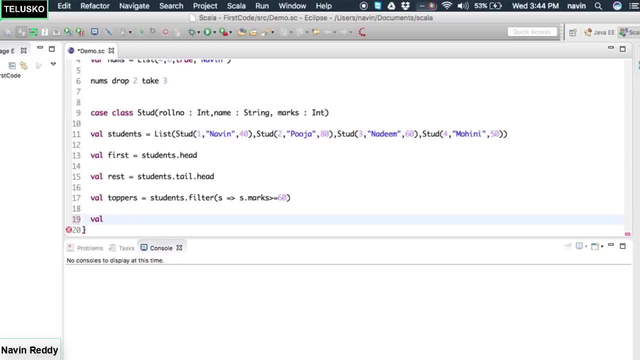 we got two people above 60 right, So we can create a partition here. we'll say: this is parts equal to student dot partition. so we have one more method which is partition. so we have to specify the condition here, on which basis you want to find the partition. so I can specify the condition there I can. 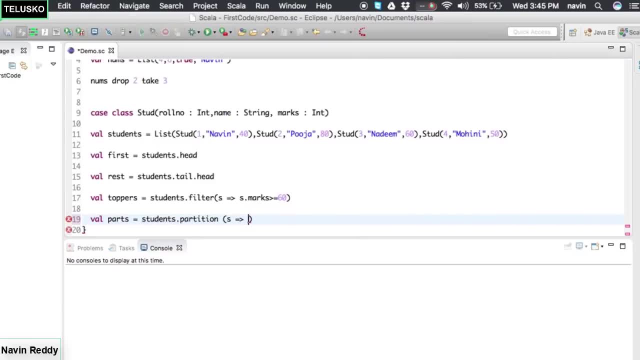 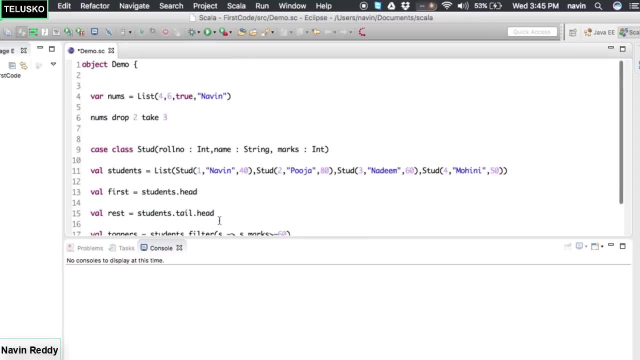 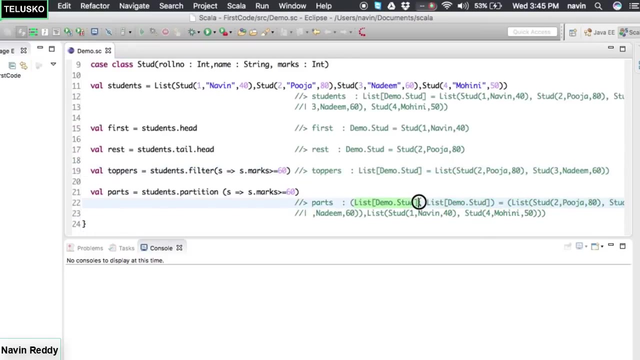 say for student, again we can. we can use lambda expression and we can say student dot marks. again the same thing: dot 60. now this parts will give you all the values, but in two particular partition. We are getting a partition of two values we got. we are getting one list, comma, second list. 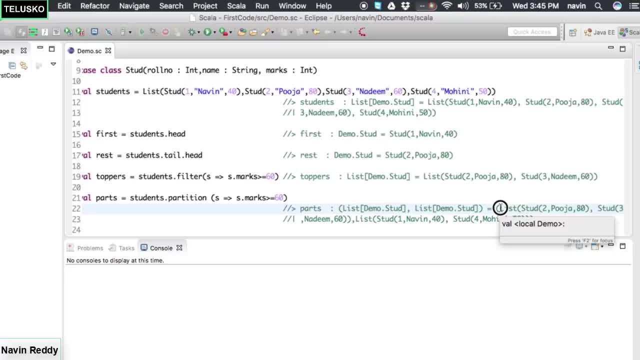 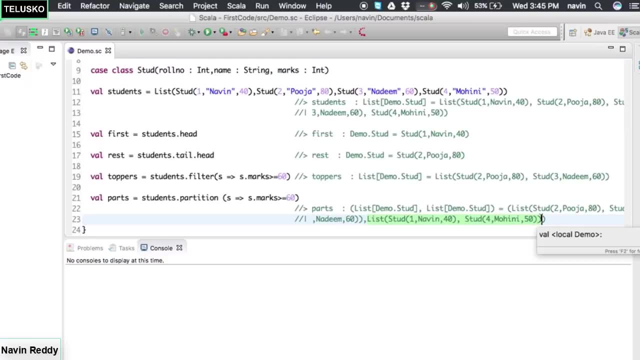 so the value of the first list is from here to here. that's your first list and this is your second list. so that's how you create. that's how we create a partition in Scala. okay, so we can use partition method, which is inbuilt method, so there are lots of inbuilt. 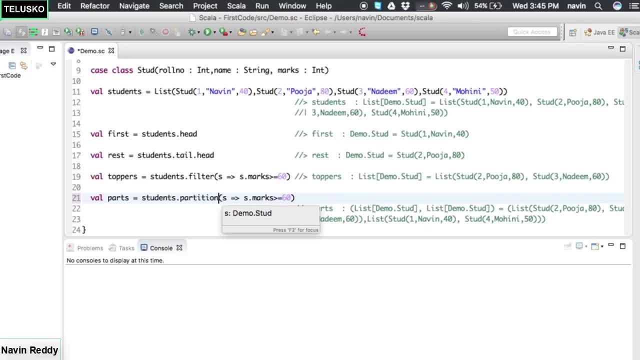 features available in Scala, as you can see. so we are. we are working more on these stuff. I mean In Scala, just to give, just to get the power of it. so that's it. that's it from this video. we have talked about lots of, lots of stuff. we have talked about how to create a list. 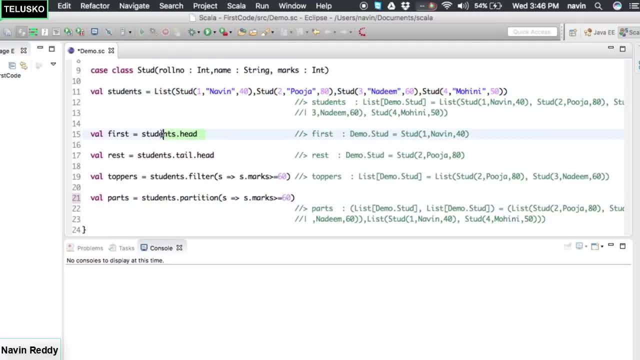 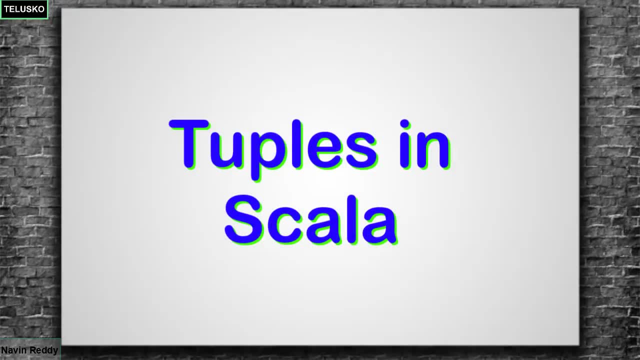 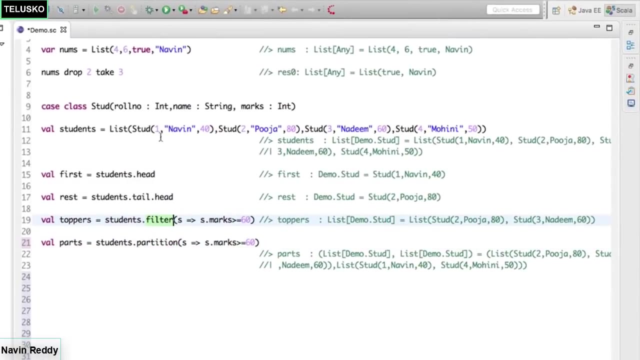 of complex objects. how do we use head? how do we use tail? how do we use filter? how do we use partition? In the last video, we have talked about how to use partition, how to use filter and then how to create a complex object. right now, what we'll do now in this video is we'll, we'll. 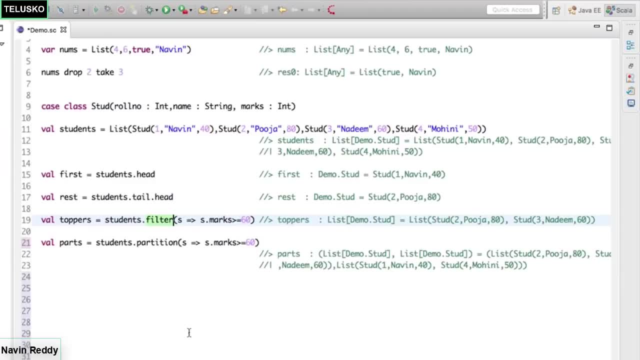 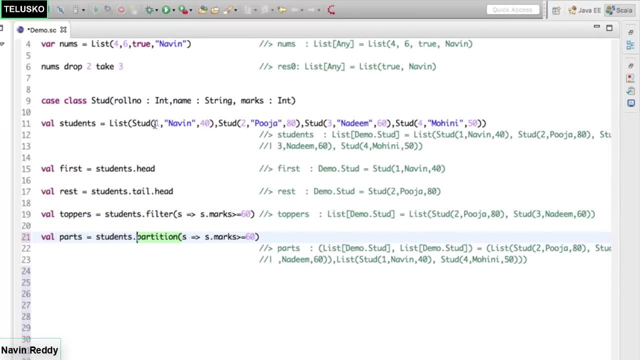 be working with tuples or tuples, we can say. so what exactly tuples are? so let's say, you have so many when you run a partition. so it is dividing the list into two parts, right? the first part is this. I mean, the first part will have two elements, which is 40 and 60. 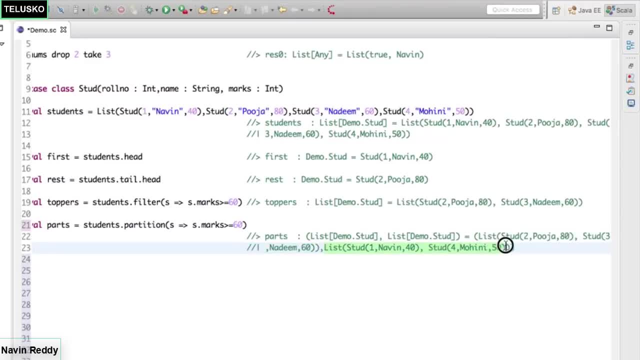 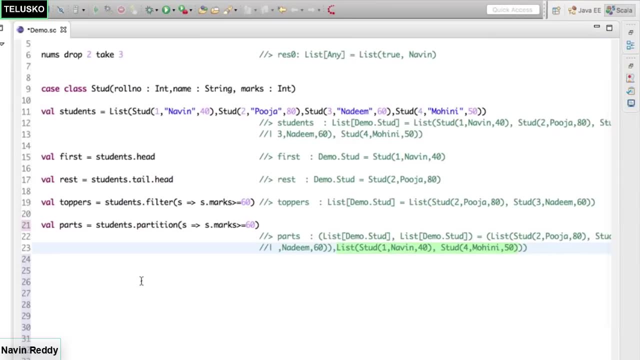 and 80, which are satisfying the condition, and then last two, which is 40 and 50, they are not satisfying. satisfying the condition, right? so again. so we have two partition, I mean we have two parts here, part one and part two. So this is so normally. what happens is, when you work with a method, it returns only one. 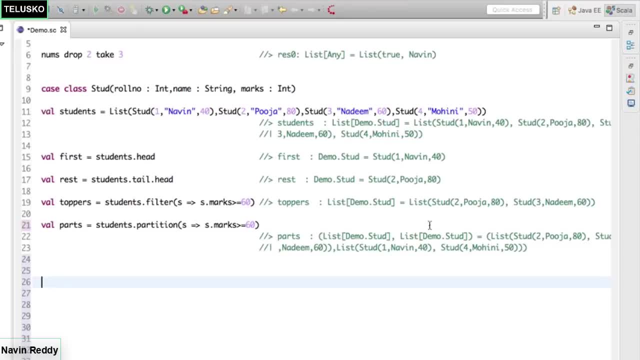 value right, but in Scala we can return multiple values and those values are called as tuples or tuples or whatever. whatever you can prefer, you can call it okay, so it is normally referred as tuples or tuples. I don't know how you pronounce it. let's say tuples. I will use the term tuples. 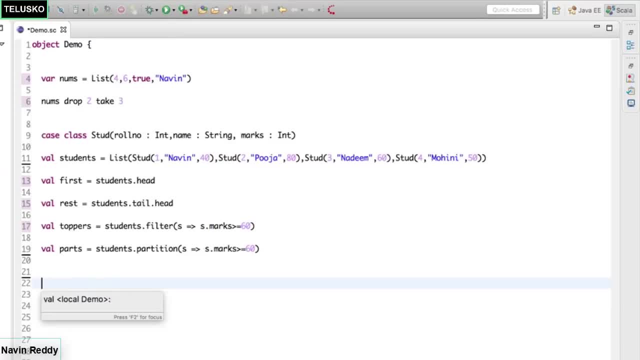 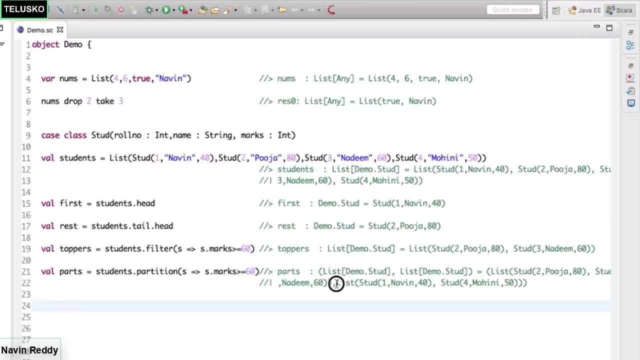 here. okay, so it is returning a tuple to you, right? because you're not getting one value, you're getting two values, two lists. now how do you fetch one list out of it? I don't want the second value, I want only the first list. so I want only the first list here, from here. 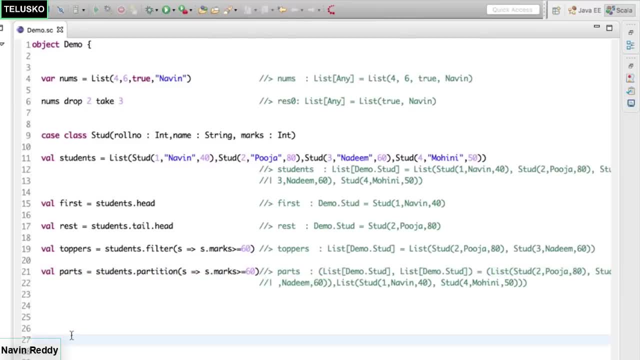 to here. so how we can do that is: we'll say val, so we'll say val, part one equal to, so that again we can use any name there. so we'll say part one, parts dot. now how do you fetch the first value now? we cannot use index numbers here, so tuples doesn't support index number. 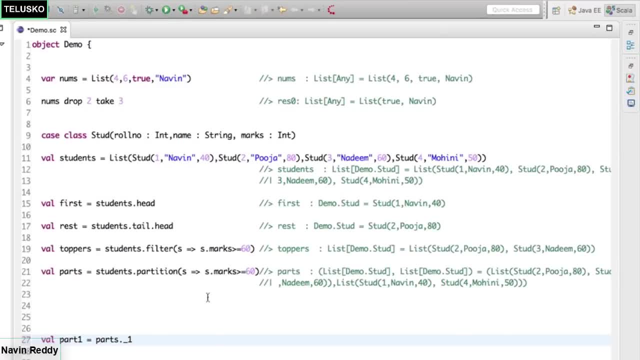 but we can use underscore one. underscore one means the first part of it and if you say enter, it should give you the value. Hopefully. yes, so you got the value, which is 80 and 60, because you are fetching the first part of tuple. we can fetch the second part also. we can say: part two equal to parts. 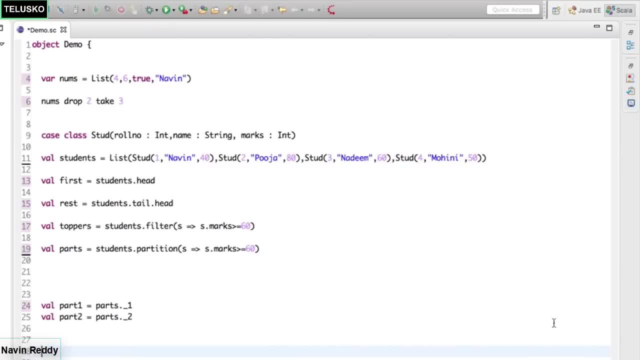 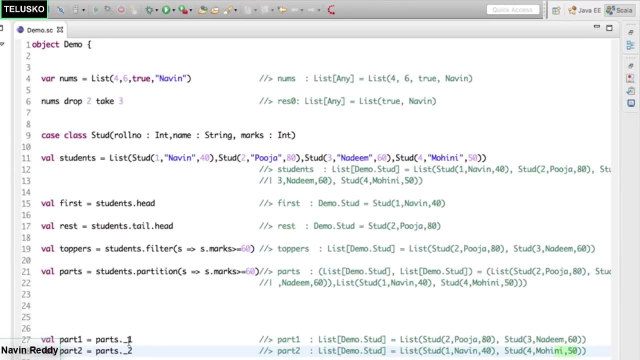 dot underscore two, so it will return the second part of tuple, which is: which is this right, which is 40, and Navin and Mohini 50? now we cannot, we cannot do. we cannot use something in this way. normally we do it in list. we cannot do that here. this will not work because in 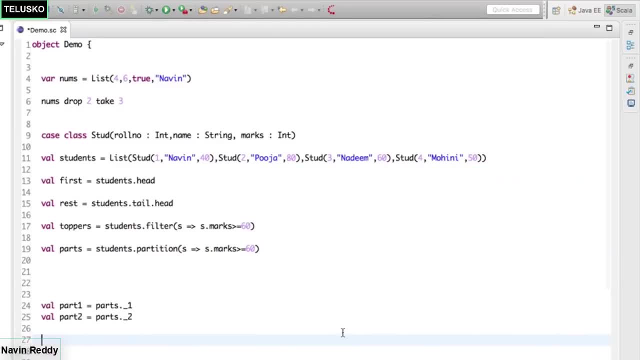 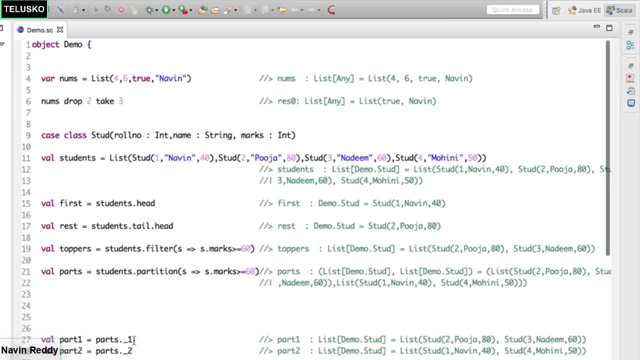 tuples, We need to use a syntax as underscore one. okay, that's how you get the value right. so this is one way. so if you're not, if you're not comfortable with this underscore one- I mean even I'm not comfortable with that- there are lots of people they're not comfortable. 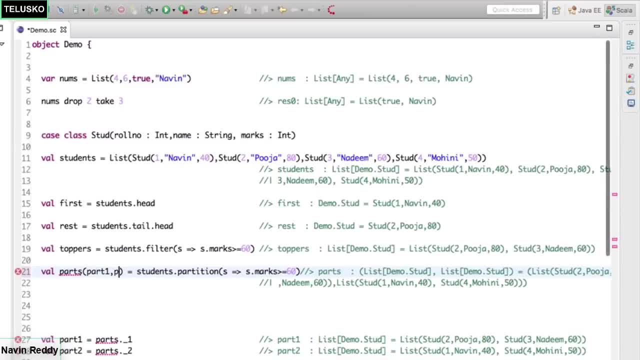 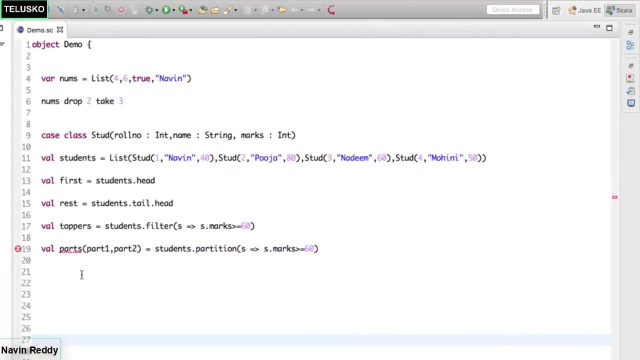 what we can simply do is here, all here itself, we can say part one, comma, part two. instead of doing this later, we can simply say part one, part two. so we are defining two things here, which is part one and part two, in fact. no, no, we do that. we don't have to use part.